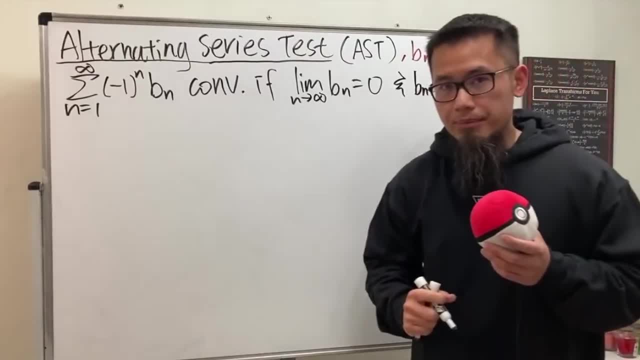 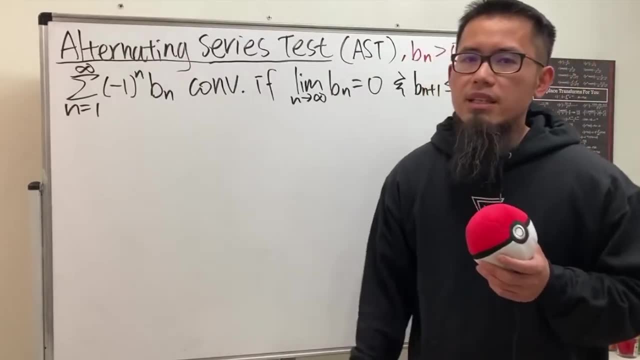 to bn. Namely. bn has to be decreasing, And you might be wondering: if bn goes to 0, doesn't that always have to be decreasing? That's not the case, because bn could have been like this. Check this out. 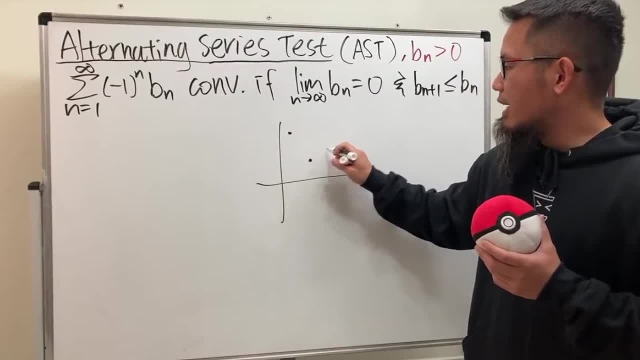 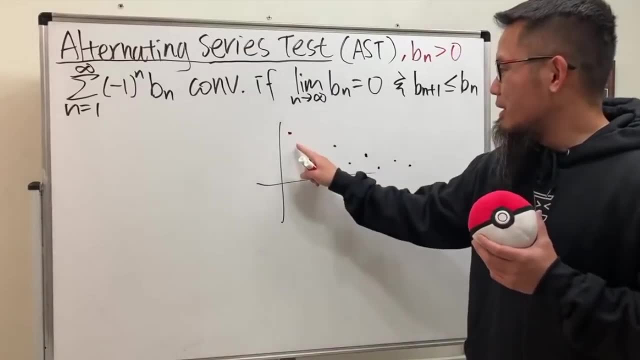 It can be like this: this and then up and then down, and then up and then down, and then up and then down. As you can see, bn is not decreasing, but bn is approaching 0.. So be really careful with that. 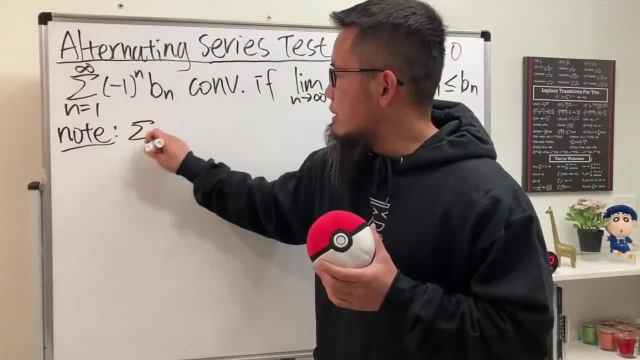 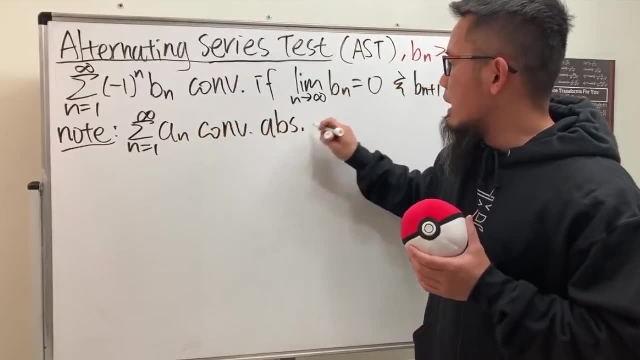 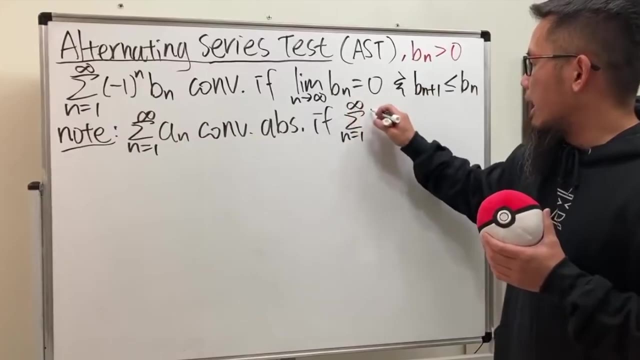 Here is a quick note. We say that the series as n goes from 1 to infinity a n. this right here converges absolutely if you apply the absolute value to the a? n And this thing right here still converges right. 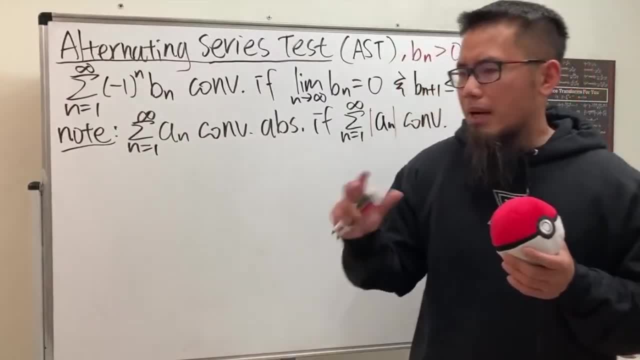 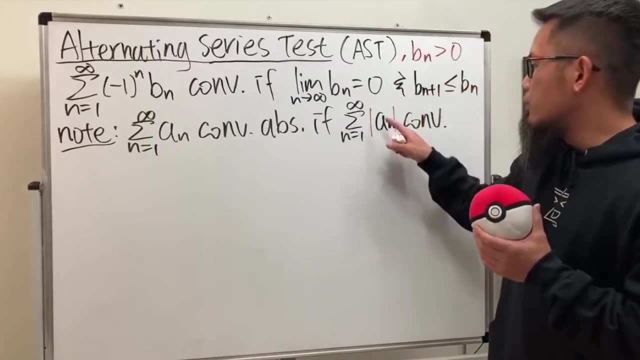 So you see, sometimes when you have a n, it might have some positive, negative terms, And when you have some negative terms you will have a bigger chance to get a convergent. But if you make everything positive, if it still converges, we say that it converges. 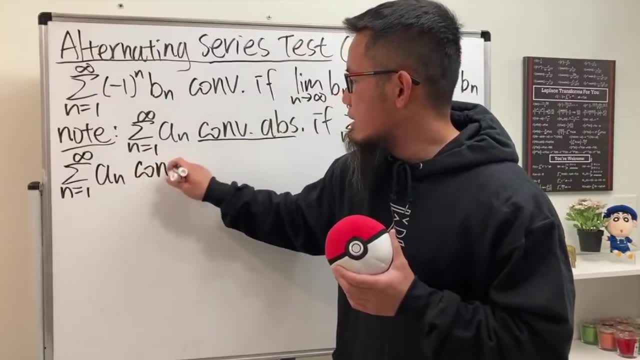 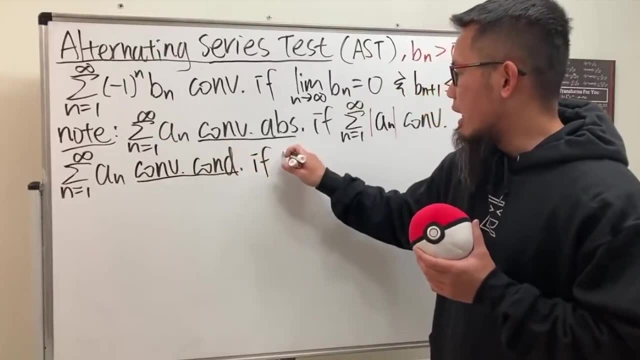 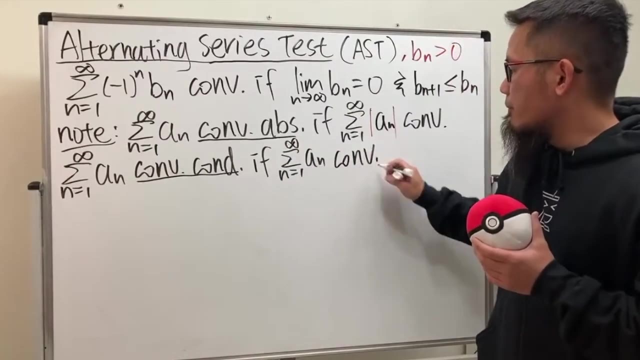 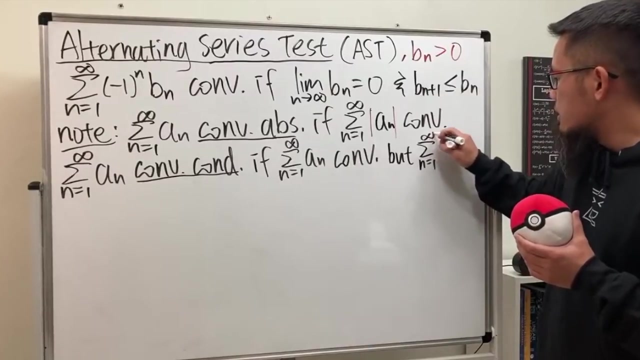 absolutely. We say that this right here converges conditionally. Conditionally if the series itself converges. So you don't do anything. You don't do the absolute value whatsoever if the series converges, But the absolute value version of it. if you apply the absolute value right here, this 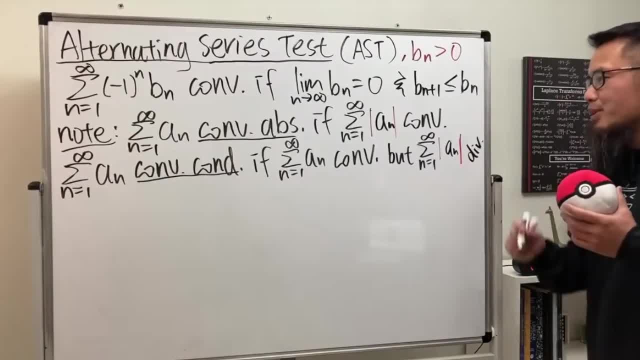 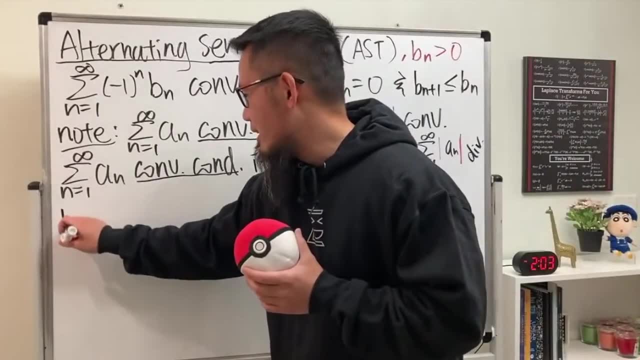 thing right here diverges, So I'll just put on div. All right, cool, We're still getting everything on the board, So this right here is usually converging. This is usually a continuation after we have the alternating series. The next one is the ratio test. 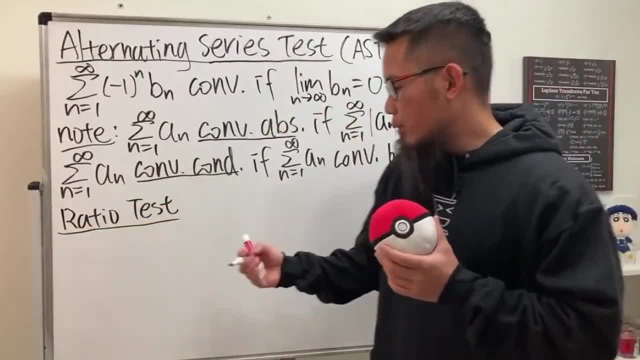 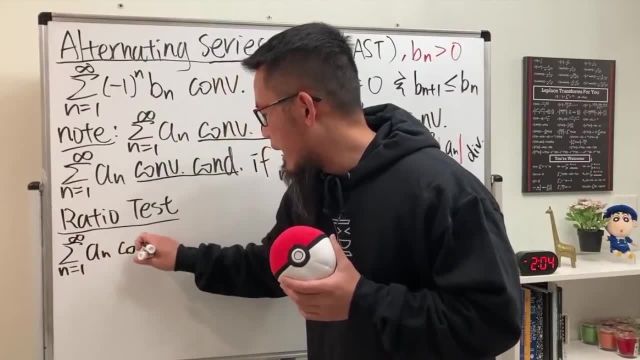 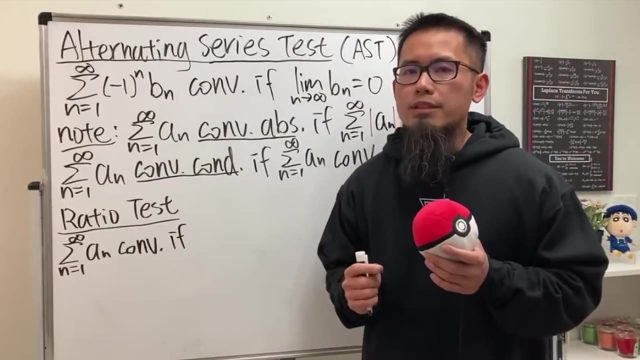 And that's what we will be going over today as well, And I will tell you that. well, here we will just say the series as n goes from 1 to infinity of a. n. this right here converges, And for this right here it has similar flavor with the limit comparison test. 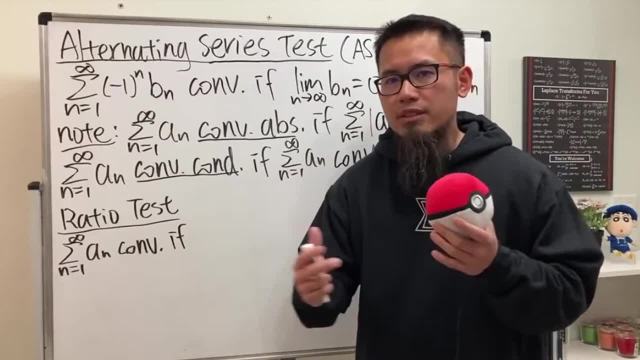 But remember, for the limit comparison test you will have to come up with another series. Okay, So let's say, you come up with another series that you know much better And then you just compare the a, n and b? n, right? 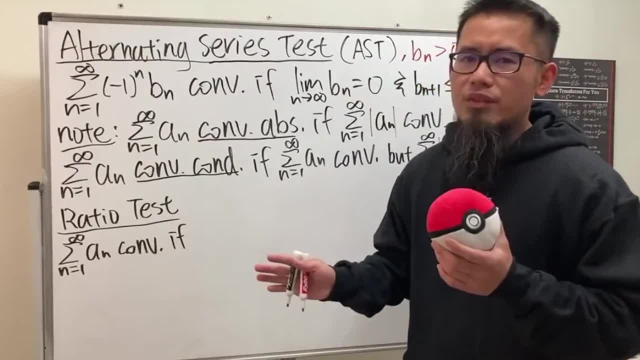 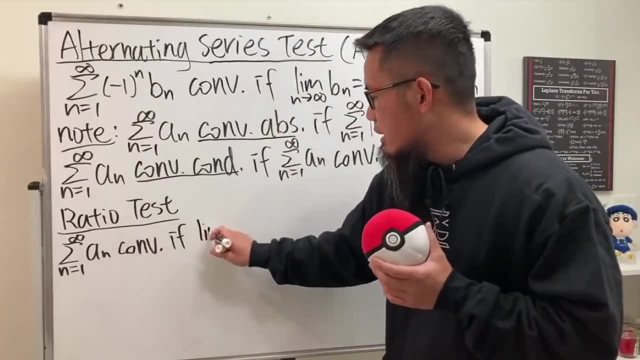 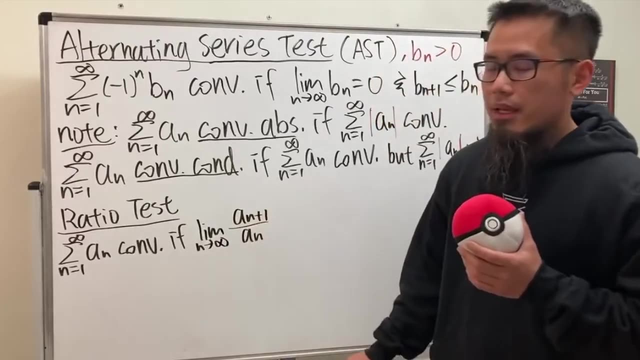 For this right here. you don't have to work out the series of b- n whatsoever, You just do this with yourself pretty much. Look at a? n here and just compute the limit, as n goes to infinity, of a? n plus 1 divided by a? n, namely the next term divided by the current term. 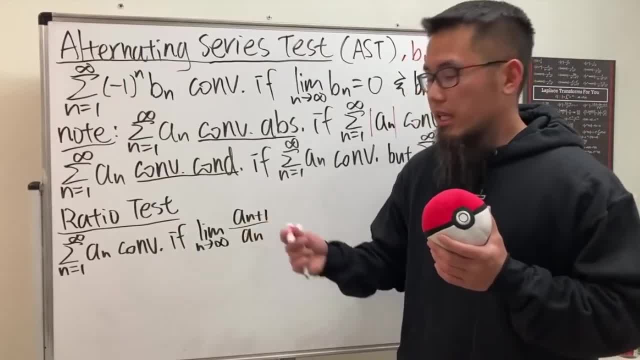 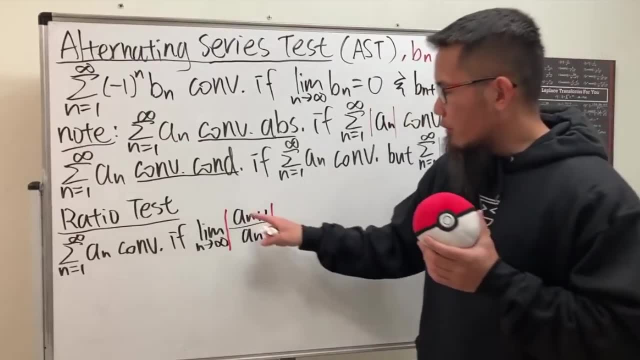 And you know what's actually really cool about the ratio test? No, it's not, It's not. It's not is that you actually apply the absolute value here. so we just care about the size of the ratio of the next term and the current term, right, so we don't really. 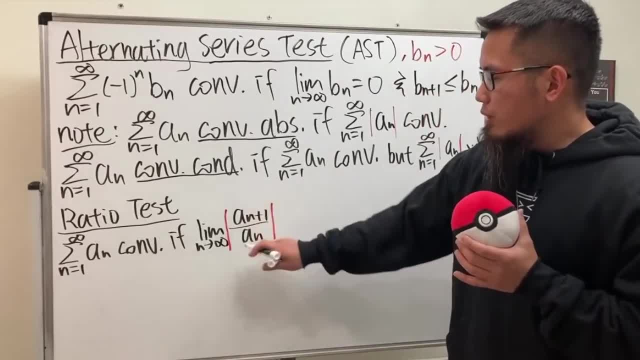 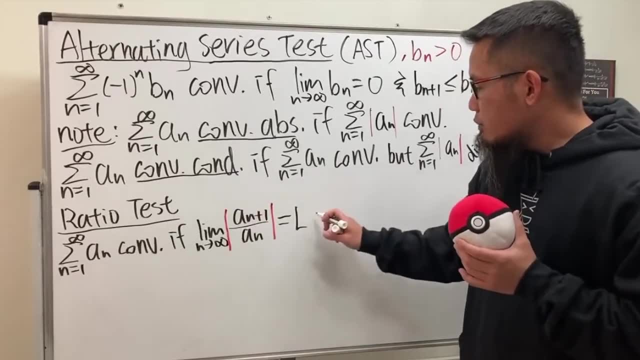 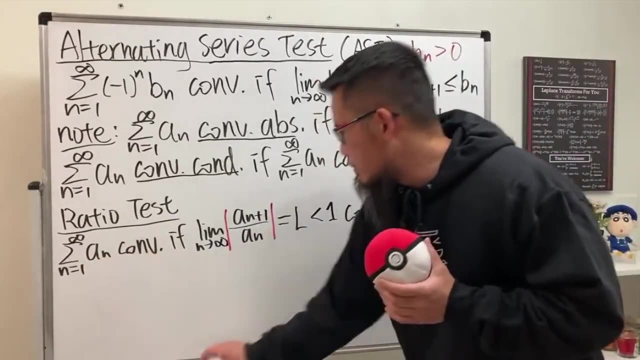 care about the sign in terms of positive, negative. and once you do this, if this right here, let's say we do get the L right, the number L, if this right here is less than 1, this right here will converge. actually I wrote down over there already: this series converges if this quantity, this limit right here is less. 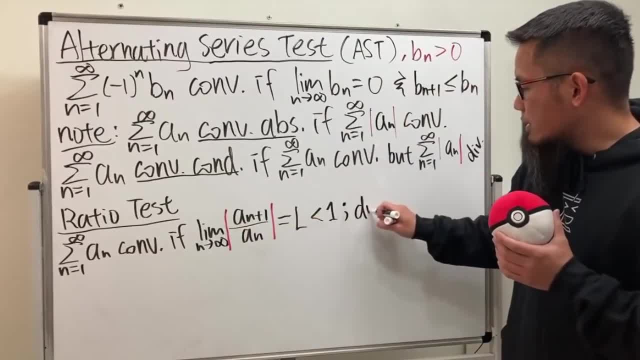 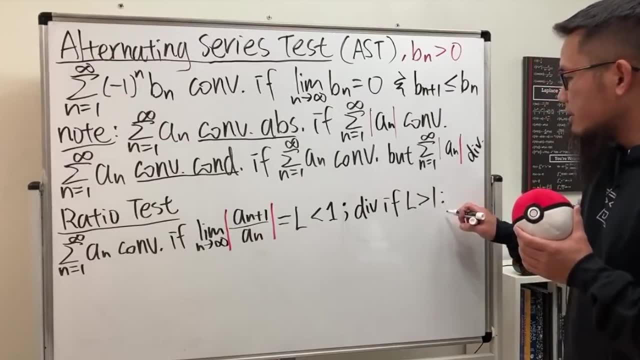 than 1 will diverges. if L is greater than 1, all right, and here's the that thing. if- oh, I'm going to write it down later because I ran out of space- if L is equal to 1, then L is greater than 1. then L is equal to 1, then L is greater than 1. 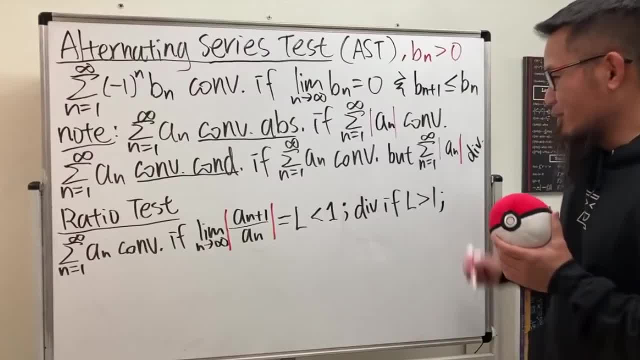 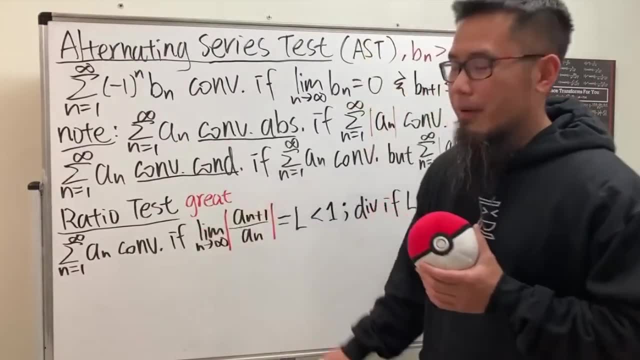 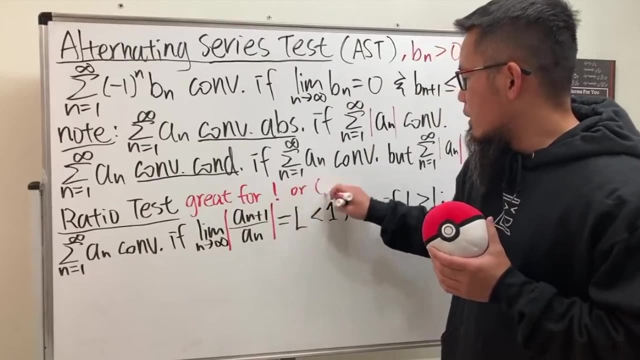 unfortunately we cannot draw any conclusion, so I will just pause, even on the run of space, and I'll tell you guys this though: ratio test is great- I would like to use the word great- for the situation that you have: factorial, or when you have the n in the exponent right, when you see 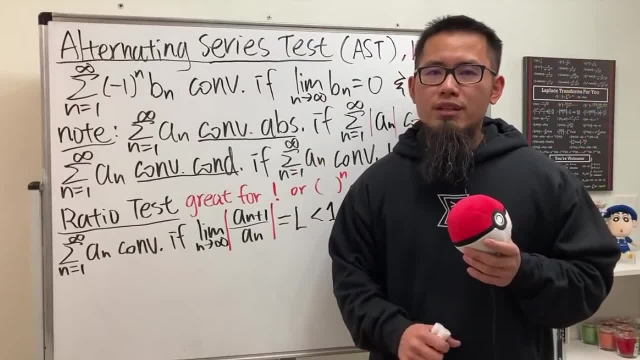 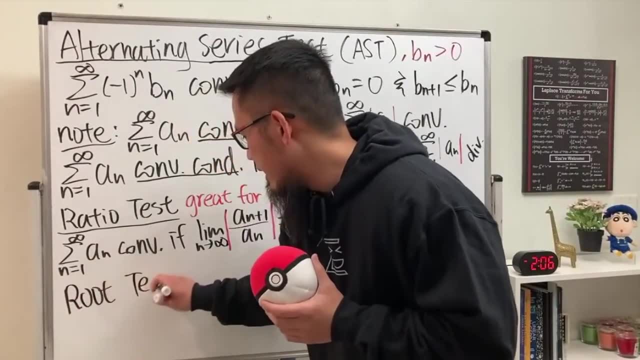 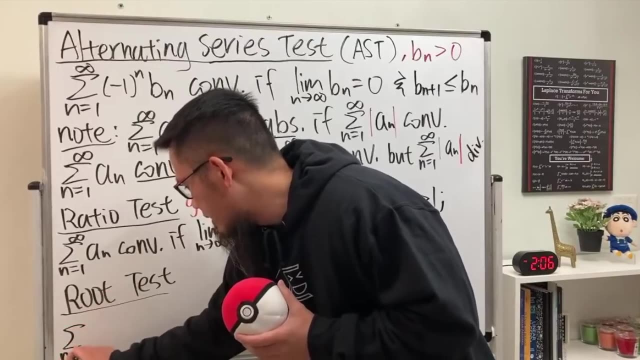 factorial or n in the exponent. go ahead and give ratio test a try, all right. on the other hand, we have the final one. we have the root test, you, and it's very similar. and for the root test I will write this down: really similar to that and goes from 1 to infinity a and this right here converges. 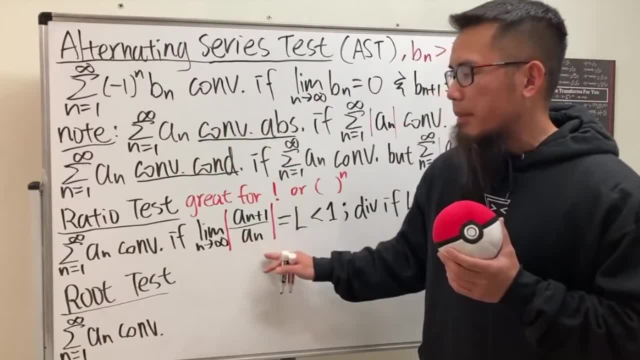 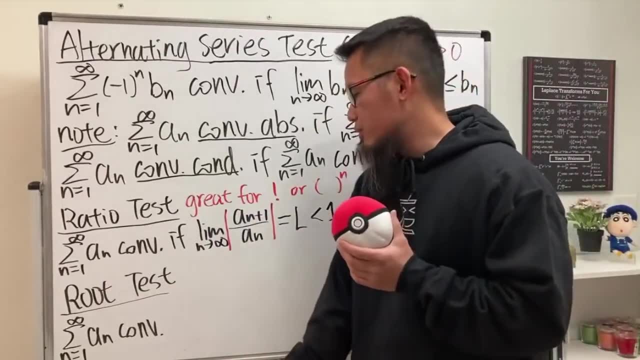 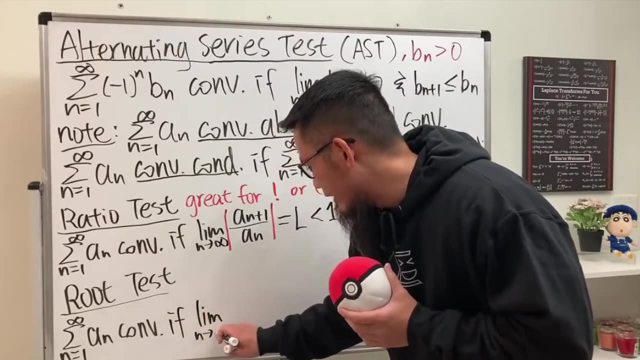 and you know, in fact, because we have the absolute value, we can actually say this right here: converges, absolutely so for the root test as well. but we can just say that converges anyway. this right here converges if the limit at the bend mod of L is greater than 1 as an equals to infinity. for the root test of. 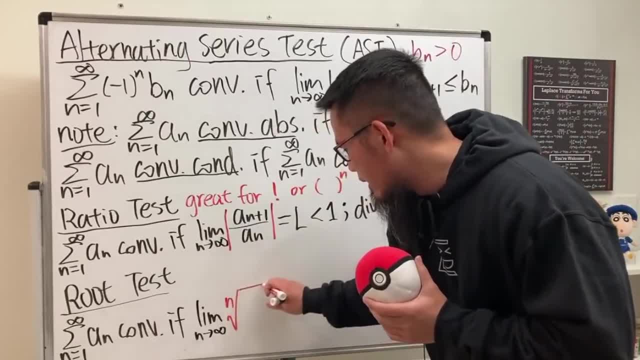 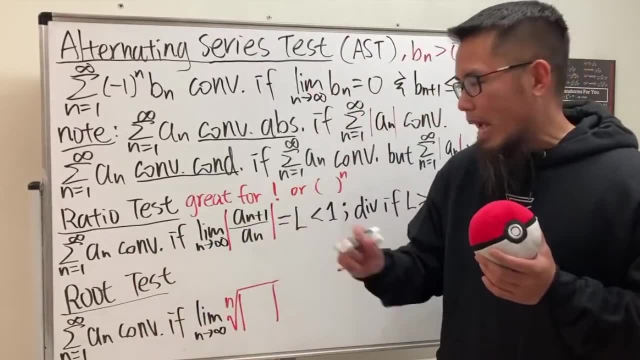 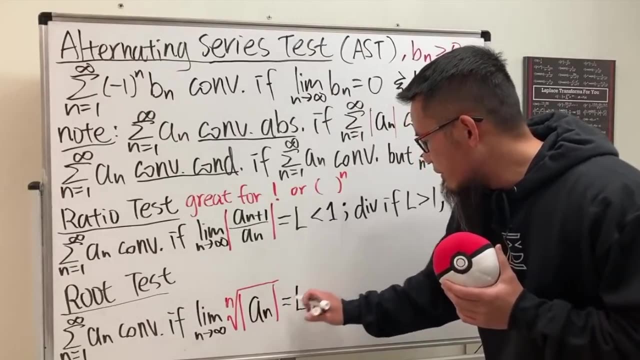 course we take the roots and we do the ganz India absolute value. so again, here and here we can actually say they converge absolutely. right here, inside we just 2 a and if this right here keeps that number L, if this L is less than 1, then you'll see that this right here converges well. 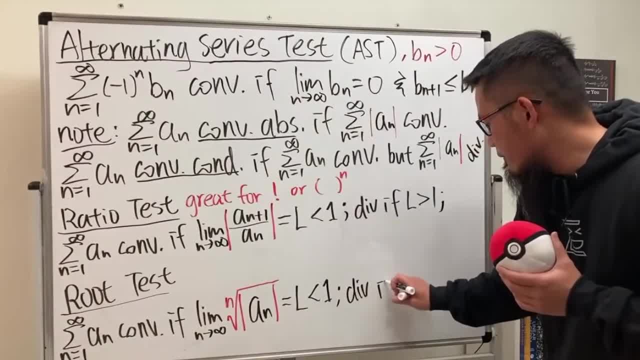 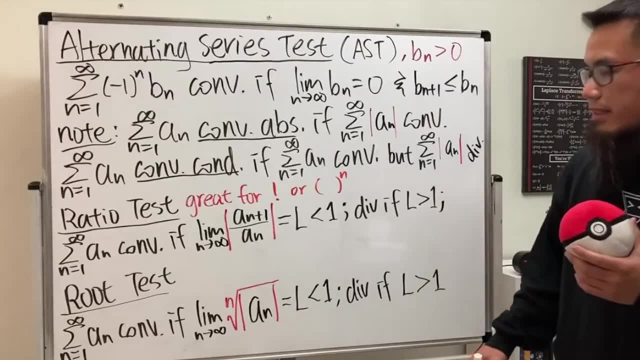 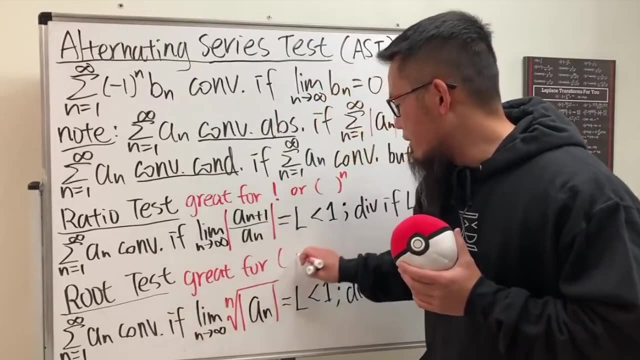 well, diverges. after the Hobby test it converges and we take this lower ever here". if L is greater than 1, right, Let me just make the 1 more artistic. So that's it. Root test, I will tell you, is great for when you have the n in the exponent. 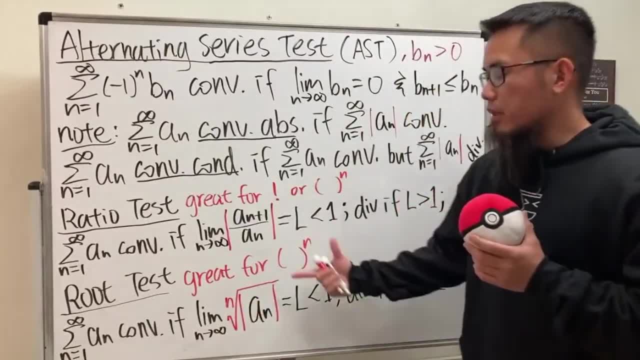 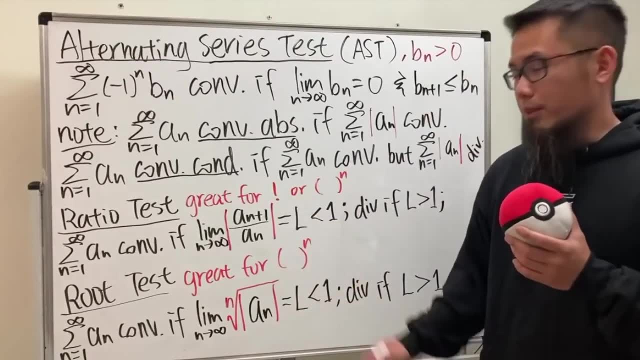 Well, of course, when you take the nth root with the n in the exponent, they can pretty much cancel, and sometimes you may have some variation that may be n squared right here. Go ahead and try the ratio test. I mean the root test. 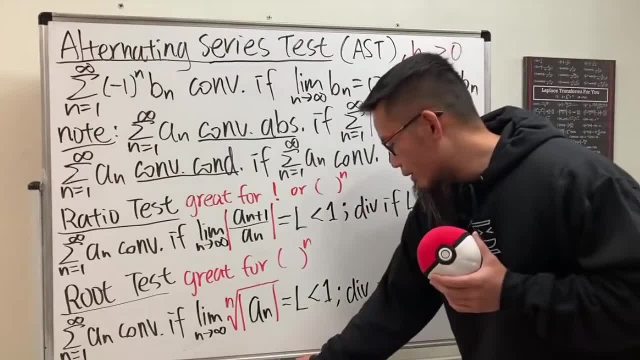 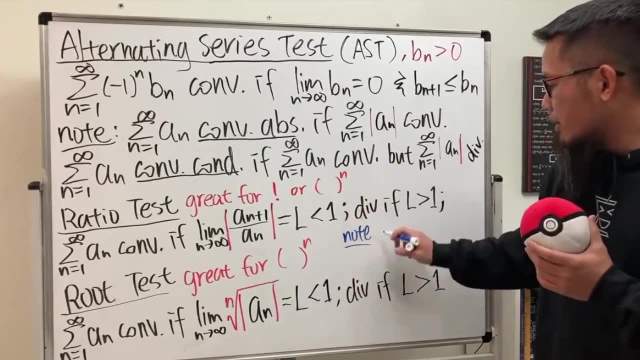 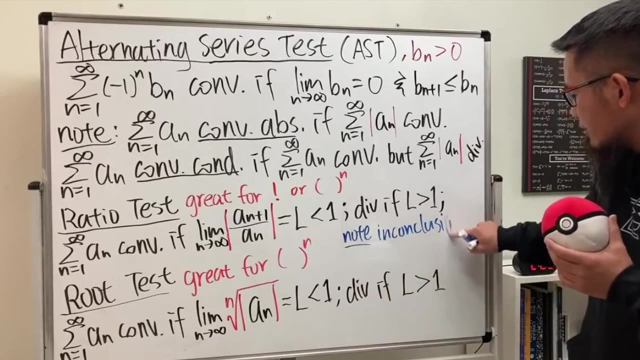 Ratio test will still work. yeah, But anyway, though, for both of these right here, I'll just have to put down a node right here in blue. These two right here is inconclusive. inconclusive. inconclusive meaning that we have to do more work. 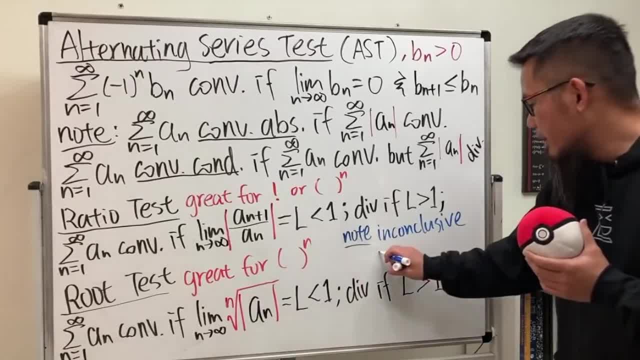 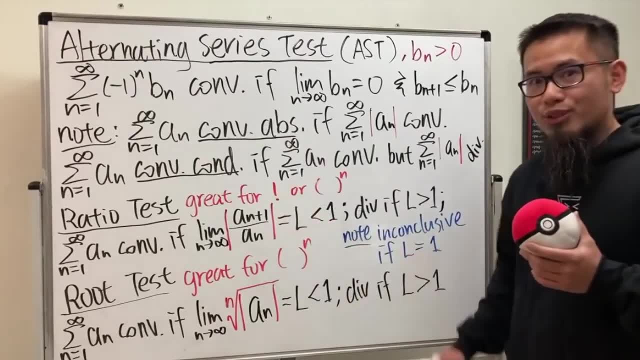 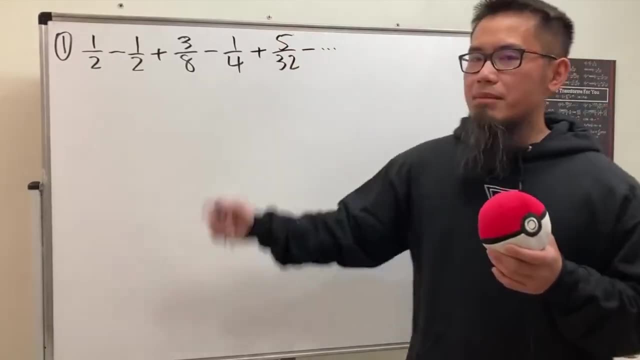 meaning that they don't work Inconclusive if L is equal to 1, for both the ratio test and also the root test. So just keep that in mind. So here we go, question number 1.. Alright, let me know the formula for the nth term. 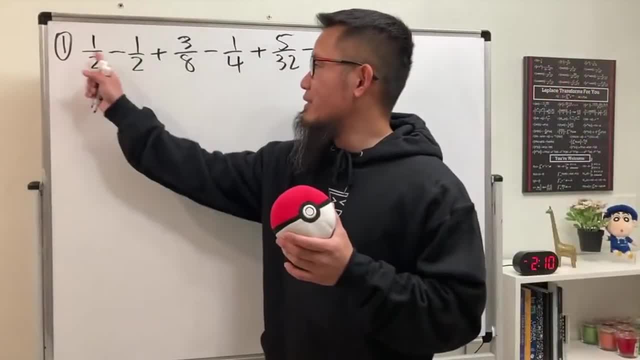 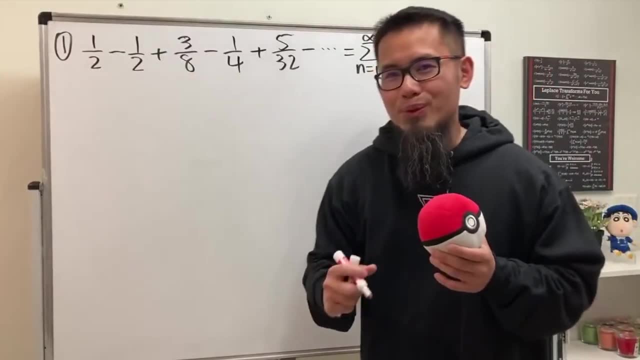 So what exactly is happening? We will have to be careful because, as you can see, the sign alternates and we start with positive. And right here, this is the trouble when you reduce fractions. sometimes, In fact, you have to make this: okay: multiply by 2,, multiply by 2.. 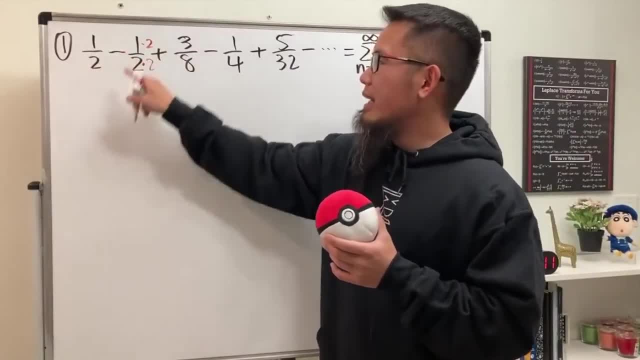 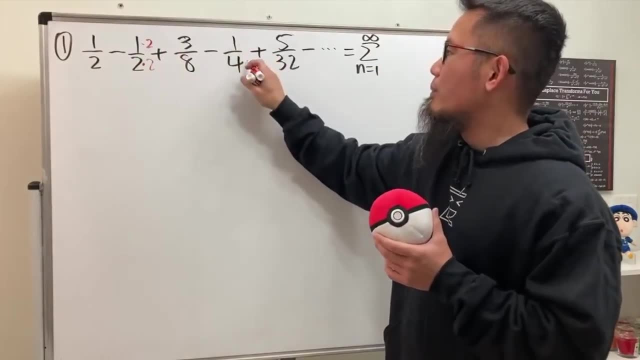 So you can see this is 1.. So you can see this is 1 over 2, and this is 2 over 4, and it's 3 over 8, which is 2 to the third power. Next, I will multiply this by 4 and 4.. 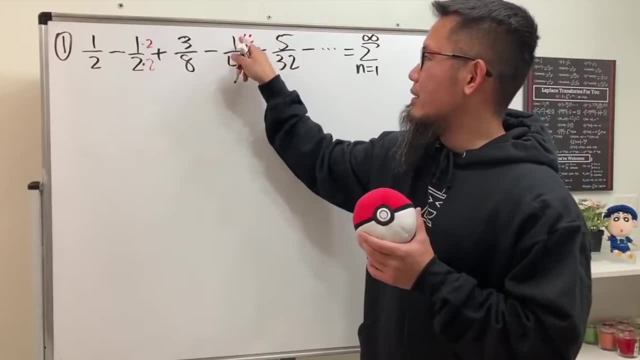 So this is 16,, which is 2 to the fourth power, and then on the top is 4.. So you can actually see we have 1,, 2,, 3,, 4,, 5 on the top. 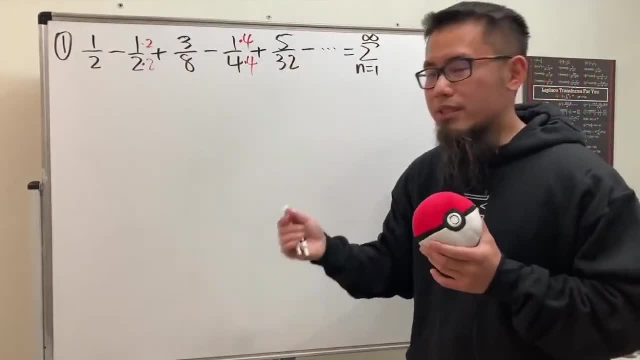 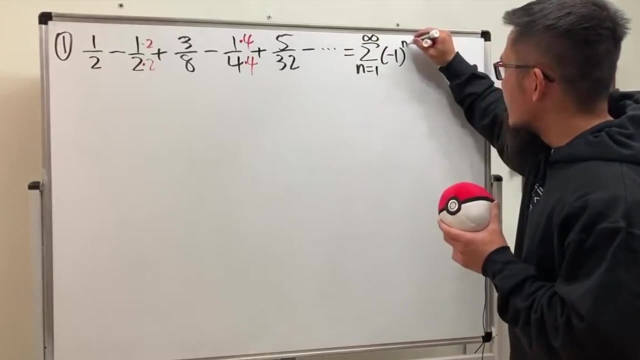 and then on the bottom is 2 to some power, But again the sign alternates. Because the sign alternates, we have negative 1, and because we start with positive, let's have n minus 1 here. If you put down n plus 1 here, nobody will get mad at you, alright. 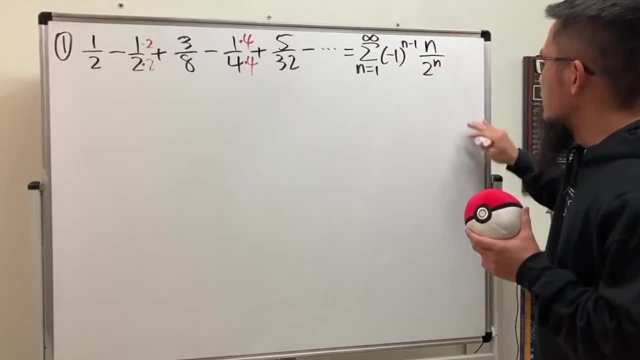 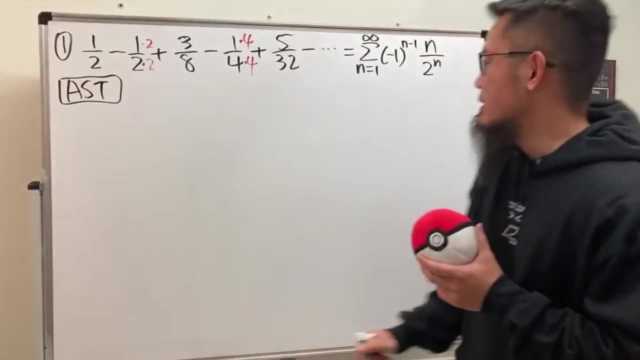 And then we have n over 2 to the n. So this, right here, is the series. So here we will apply the alternating series test and this is all you have to do it. Pay attention to the positive terms, which is the bn portion here. 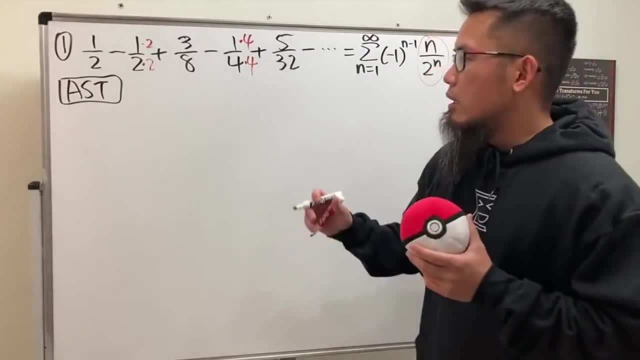 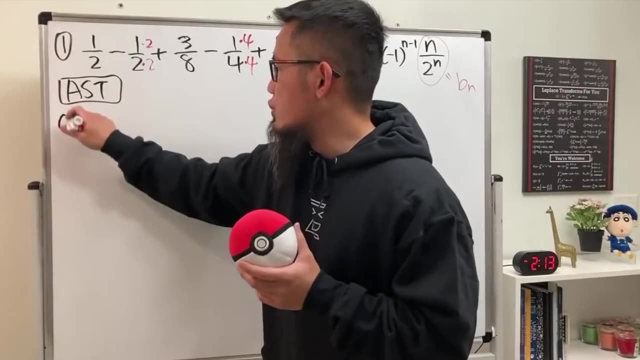 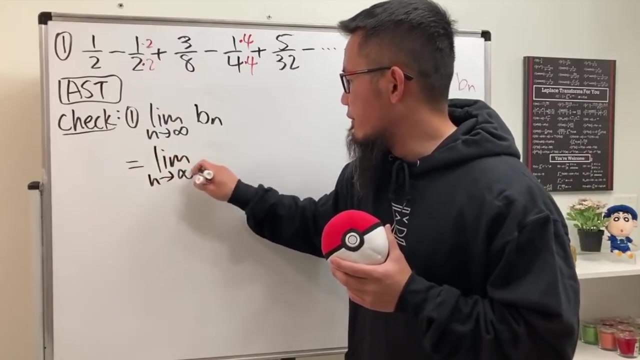 which is right here, n over 2 to the n, And because we have this factor, so we can use alternating series. And to do so all we have to do is we check the following: The first thing, this right here, is the limit, as n goes to infinity. 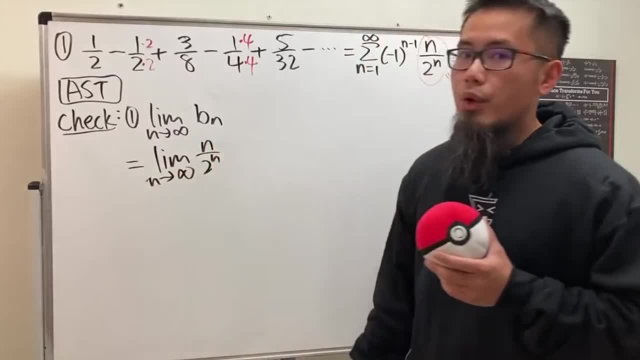 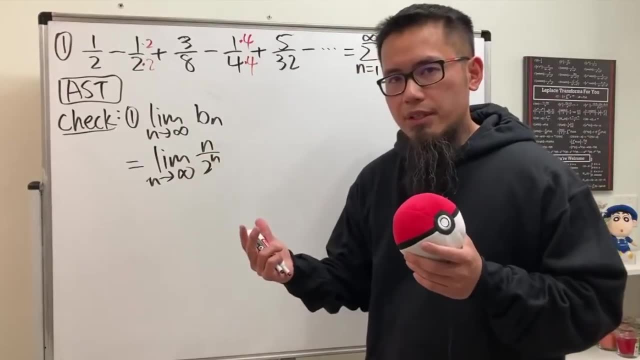 and bn is n over 2 to the n. Well, as n goes to infinity, we have infinity over 2 to the infinity. This is technically infinity over infinity, but we can use the list, So this right here is actually just equal to 0.. 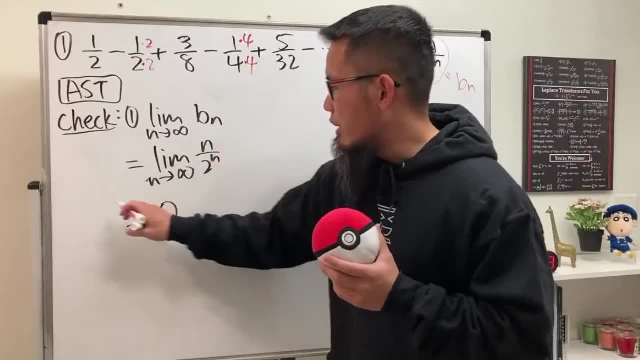 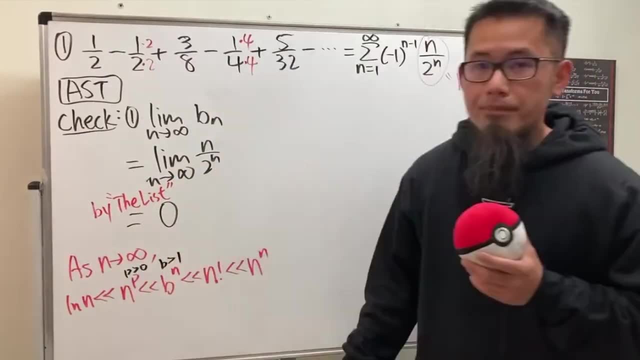 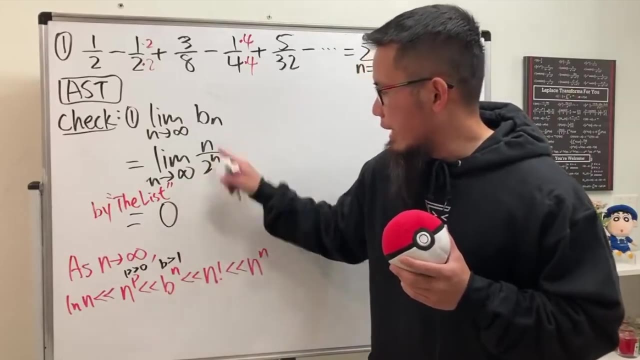 And for my students, you can just go from here to here and maybe you can just mention by the list And let me just review with you guys real quick. As you can see, this is n to the first power and this is smaller than 2 to the nth power, right? 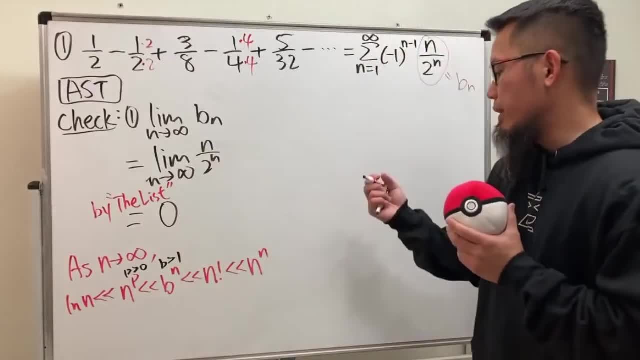 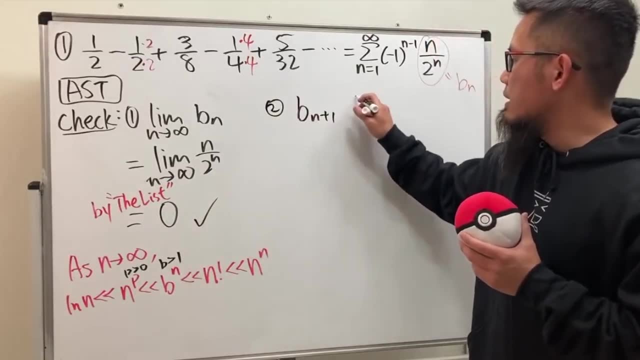 So that's why it just goes to 0.. So quick and nice way to do it. Secondly, we are going to check. We are going to check if bn plus 1 is less than bn or not, And you can put down less than or less than equal to. 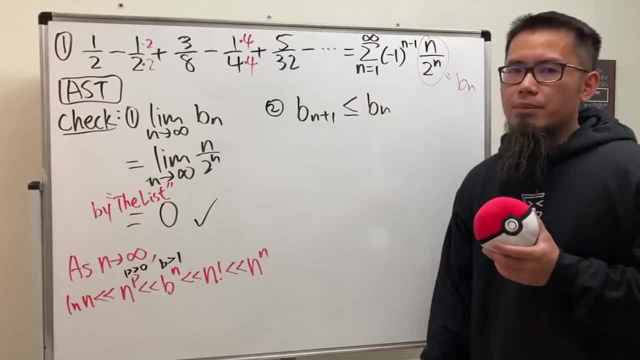 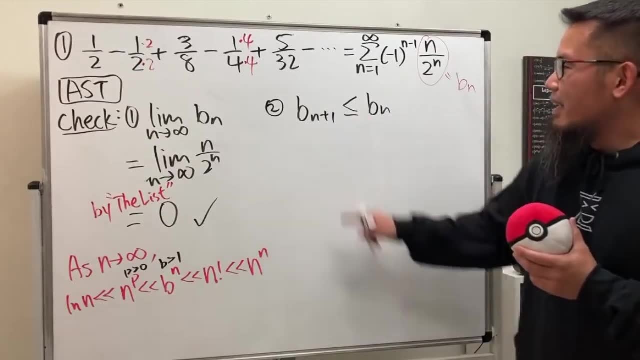 doesn't really matter that much, But I think I have about- I don't know- at least hundreds of videos that I put down less than or equal to, so I'll just keep it in that way. If you put this down, okay, bn plus 1, you just put n plus 1 into here and here. 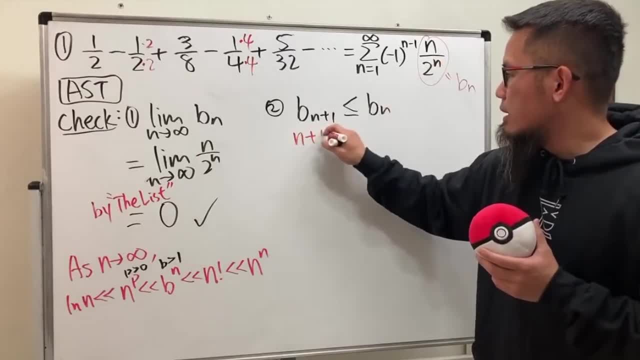 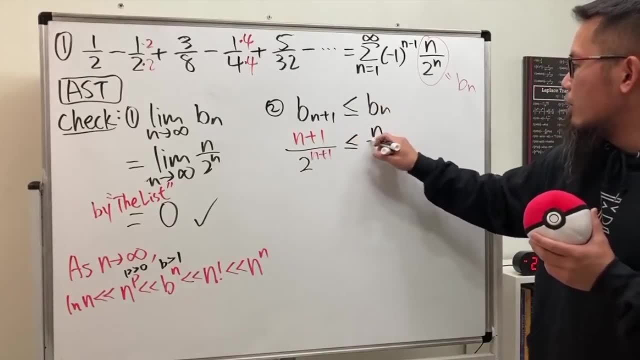 so we get n plus 1 over 2 to the n plus 1.. And we are trying to see if this is less than or equal to n over 2 to the n And just do the typical work, Because everything is positive, so we can cross, multiply. 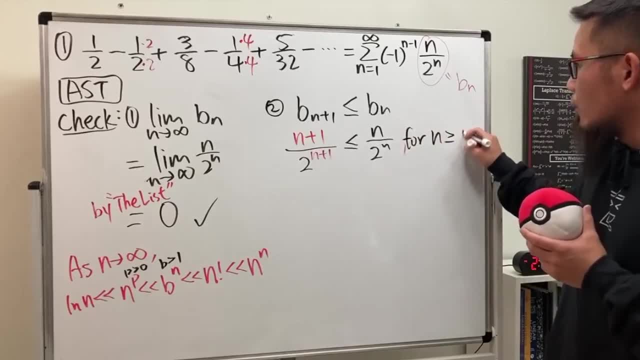 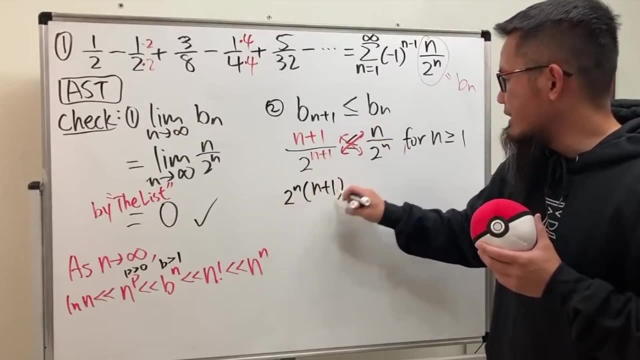 and by the way, we should say for n is greater than or equal to 1.. Anyway, just do the usual thing. So this times, that is 2 to the n n plus 1.. Well, I should technically write down a question mark. 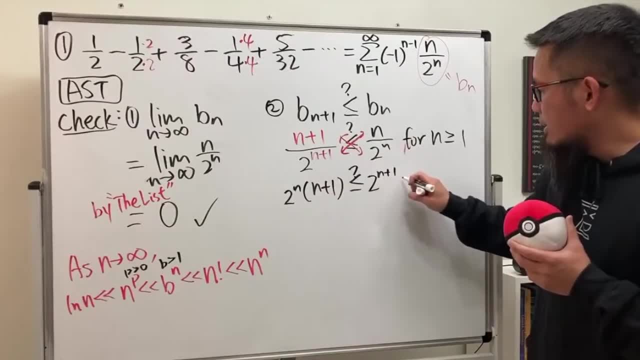 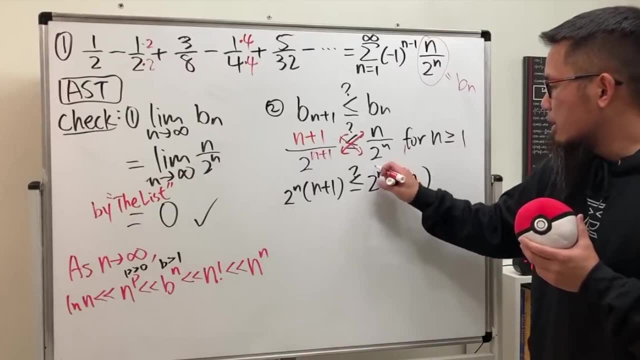 All right. this times, that is 2 to the n plus 1 times n. All right, is this true? Well, we can do the following. This right here is the same as 2 to the n times 2, right. 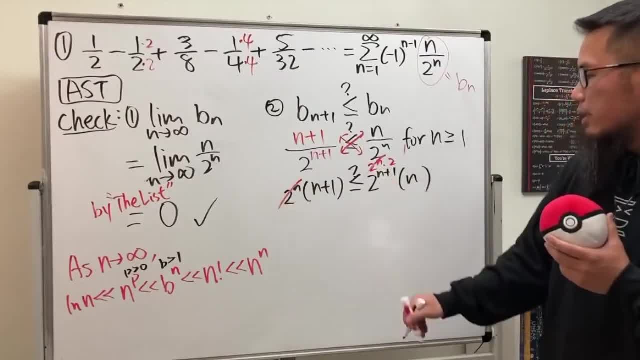 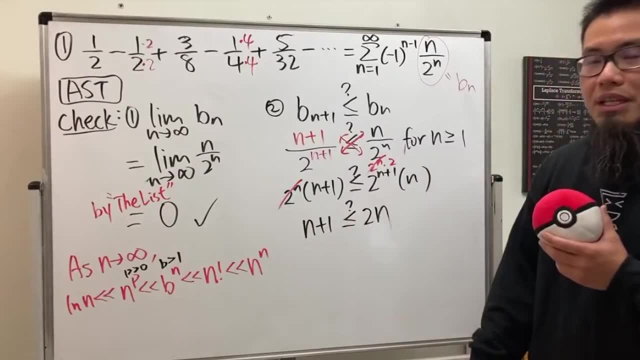 Both of them are positive, so we can cancel And, as you can see, on the left-hand side we have n plus 1.. Is this less than or equal to, 2 times n? If you would like, you can minus n on both sides. cancel this out and have a look. 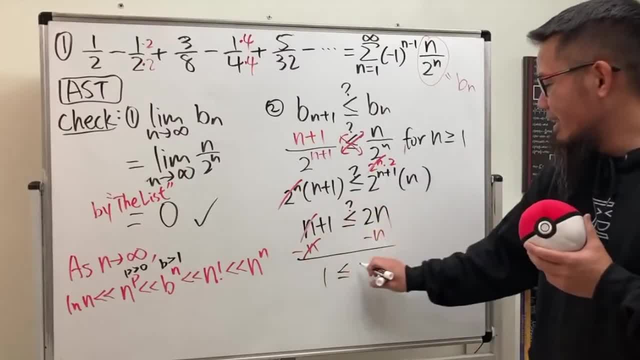 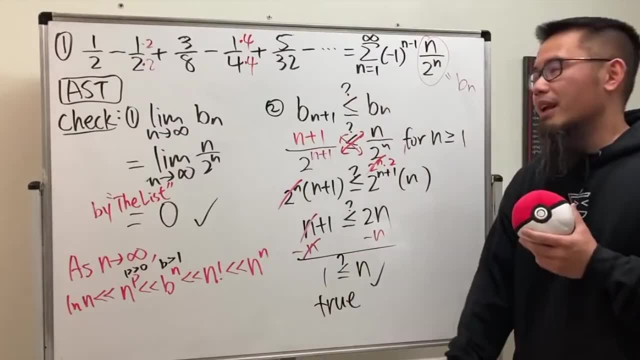 This right here is 1 less than or equal to n. Is this true? Yes, right, Because the series goes from 1 to infinity, So it's so true. Therefore, as you can see by the alternating series test. 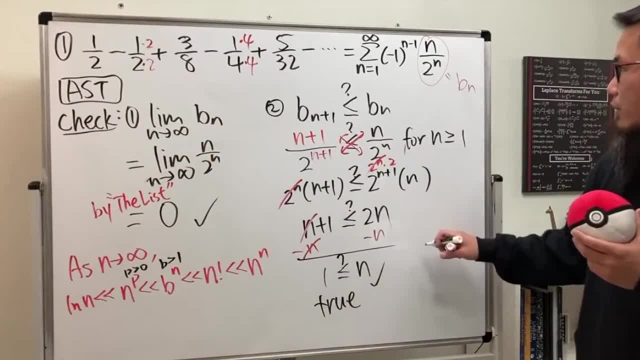 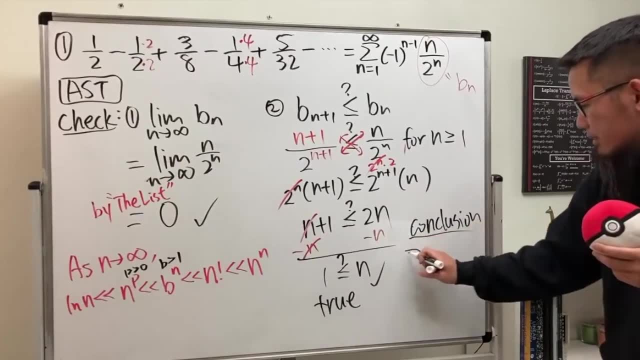 this right here converges, So I will just write it down right here. So here is the conclusion, right. The series as n goes from 1 to infinity negative, 1 to the n minus 1, n over 2 to the n. 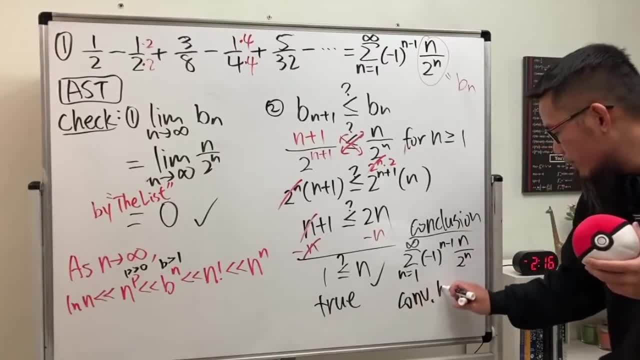 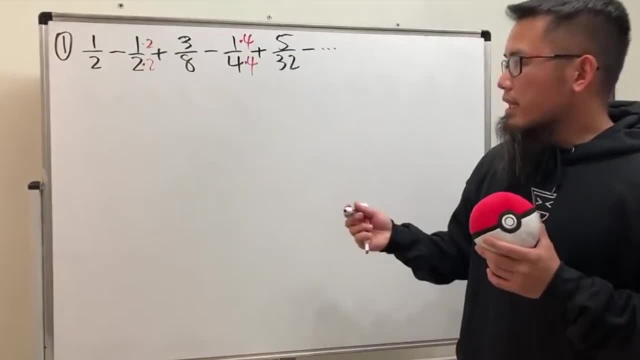 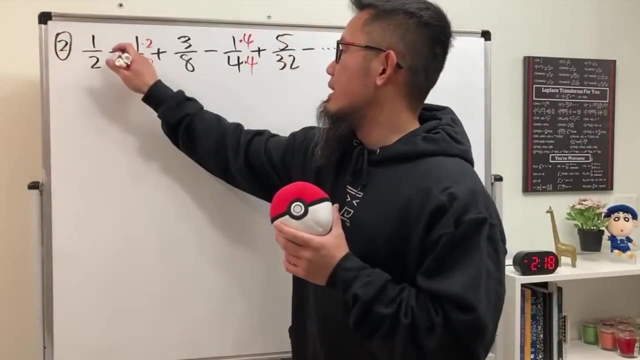 this thing right here converges- and we can just mention that- by the alternating series test Yep. so that's how it works for that. Alright. for the second question, it's actually the same thing, right? You have the same numbers. but everything is positive now, right? 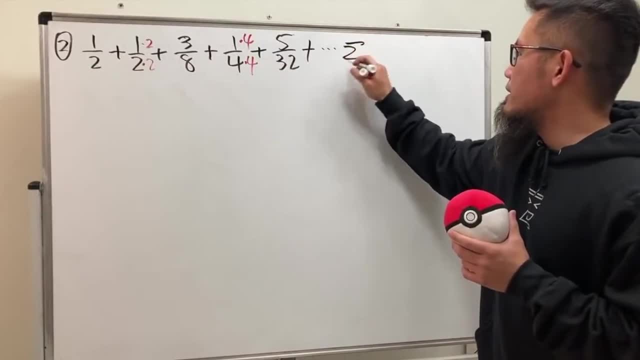 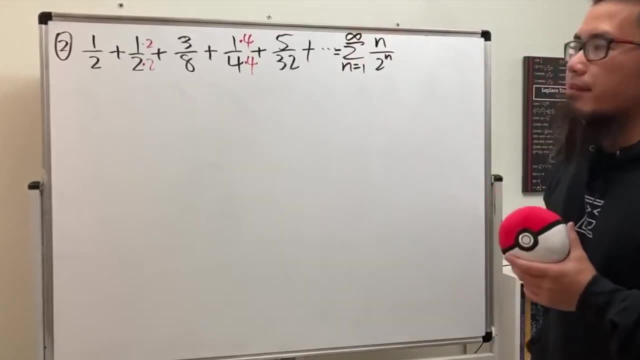 And the truth is this: right here is just going to be the series as n goes from 1 to infinity, n over 2 to the n. So this is the absolute value version of the first one, because it does not alternate anymore. 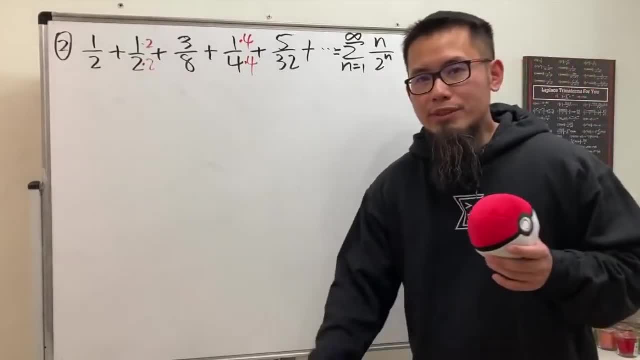 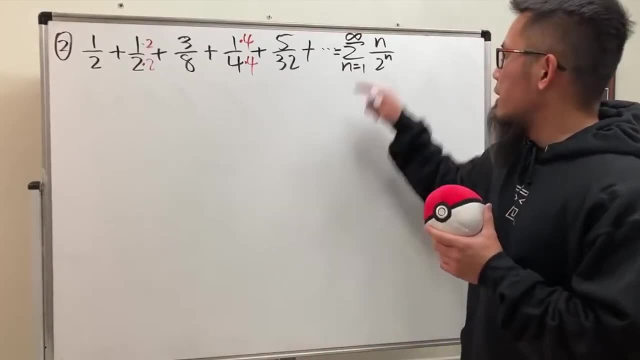 For this one though. we cannot use the alternating series anymore. We have to do it with the ratio test. Maybe the root test will work as well, but if you do the nth root of n, you will have to work out a little bit more work for the limit for that. 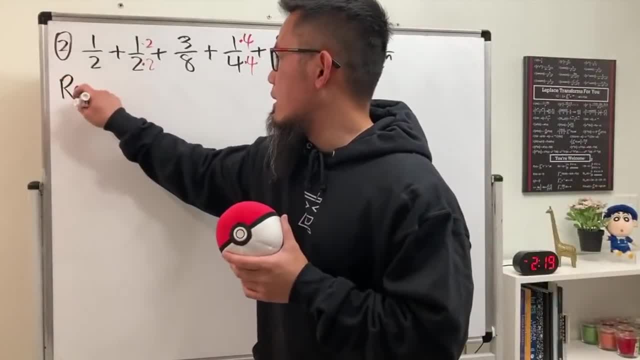 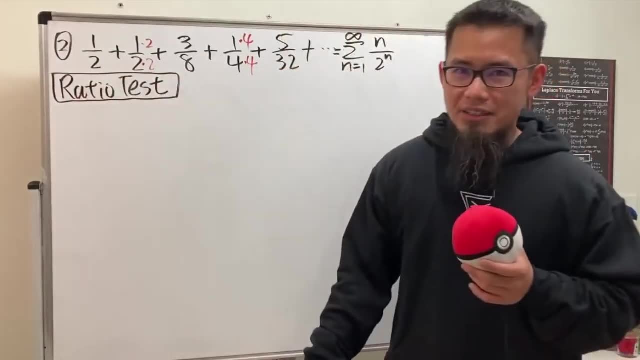 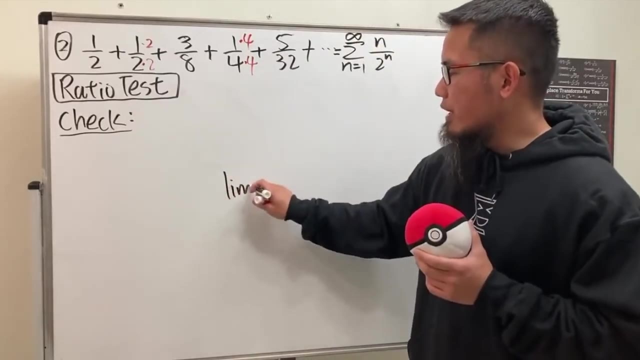 But ratio test, it will be slightly better. So here we go: ratio test, And please do not abbreviate ratio test as RT, because root test is also RT And I really don't know why. Usually, when we do the limit, we write down the LIM, right. 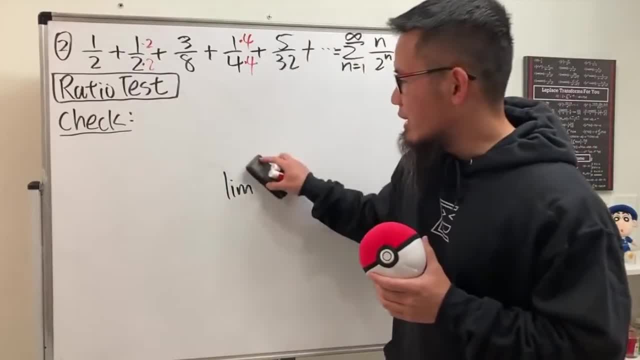 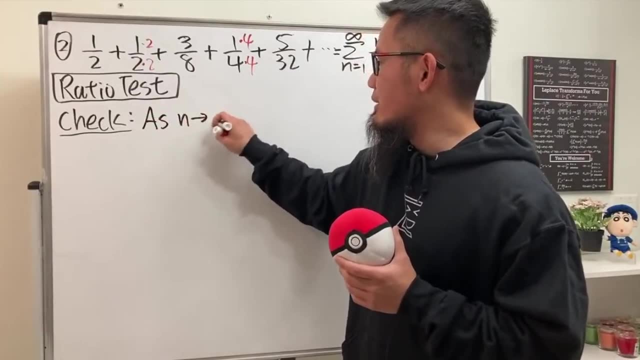 But every single time, once we are at the ratio test, I will tell my students: you can do it another way. You can just say s? n goes to infinity. When you put this down, you don't have to write down the LIM anymore. 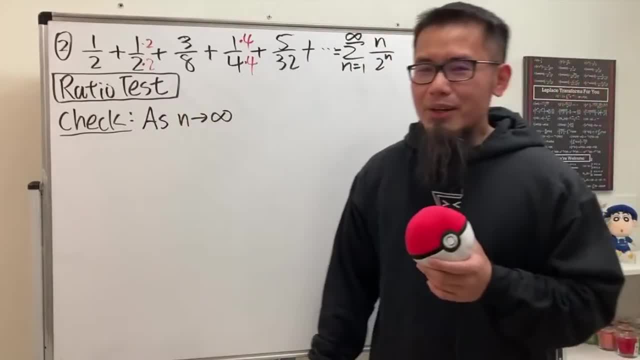 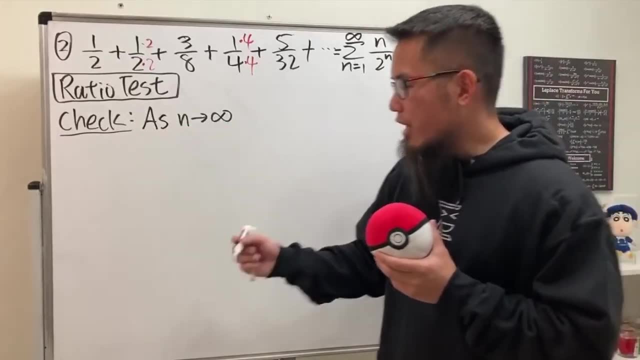 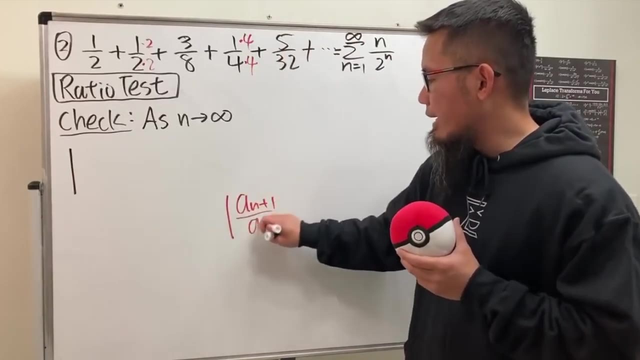 It's just a lot easier. And you might be wondering how come I don't do that any earlier. I don't know. Anyway, s n goes to infinity. we are going to check that. the absolute value- and remember it was absolute value of a n plus 1 over a n. 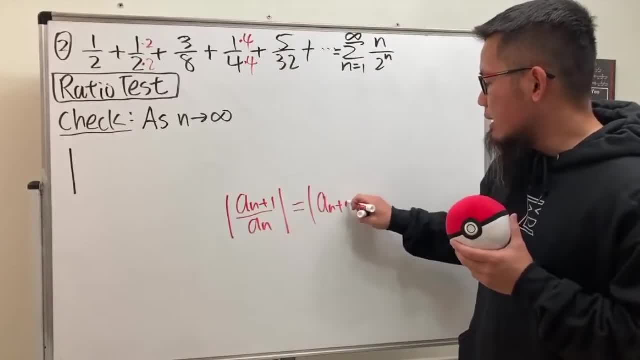 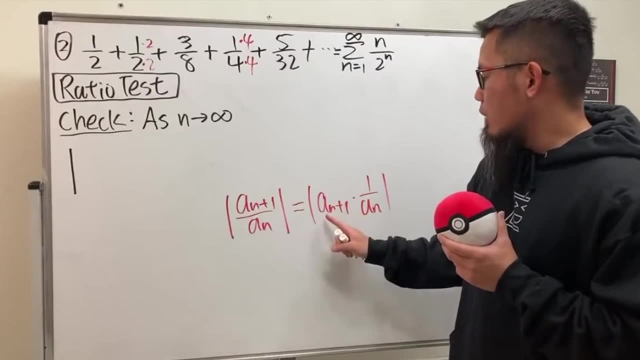 But this right here is the same as a n plus 1 times the reciprocal of a n Right. So we are going to study it like this First part. we have a n plus 1.. This time this is the a n. 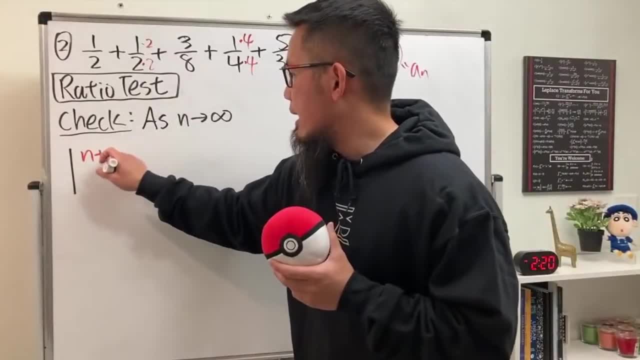 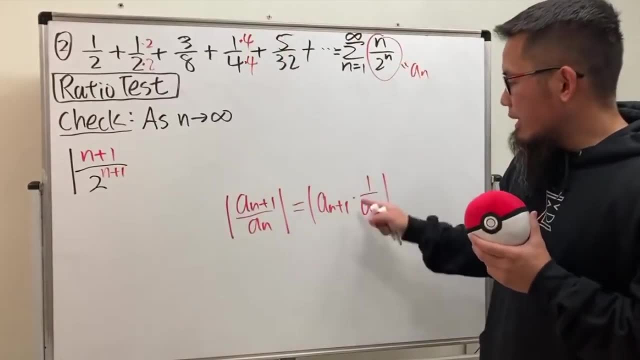 So a n plus 1, it becomes n plus 1 over 2 to the n plus 1.. Right, So that's the a n plus 1.. And then we will multiply by the reciprocal of a n. So you just do this upside down. 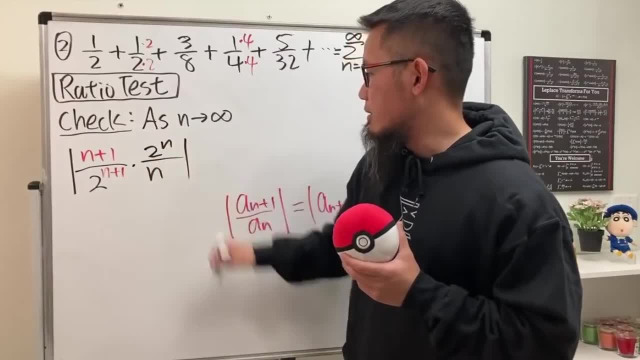 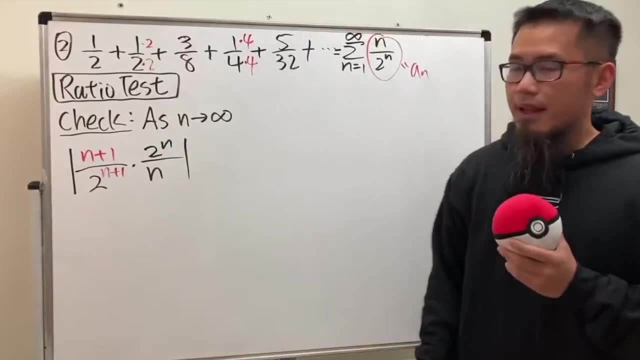 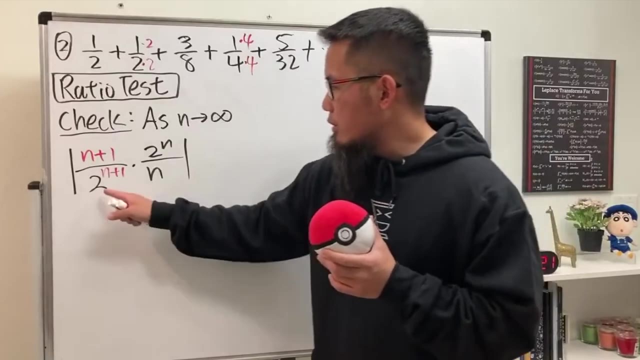 So you have 2 to the n over n like so. So this is the expression that we will be focusing on: Good. Now here's the deal: Break down the bigger exponent and sometimes maybe the bigger factorial. Here you see 2 to the n plus 1.. 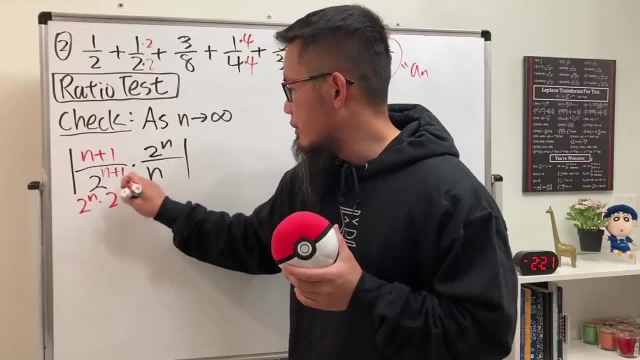 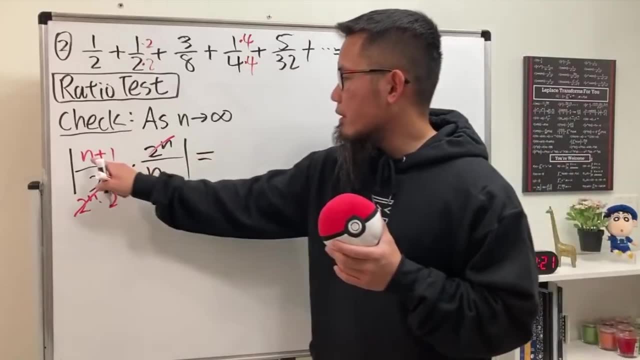 We can just rewrite it as 2 to the n times 2 to the first. This and that cancel out nicely. Well, this expression is equal to: on the top we just have n plus 1,, on the bottom we have 2n. 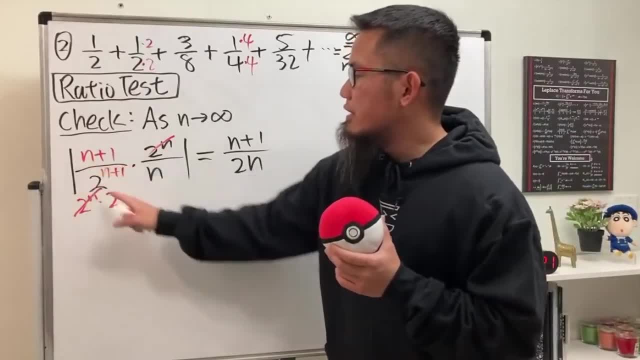 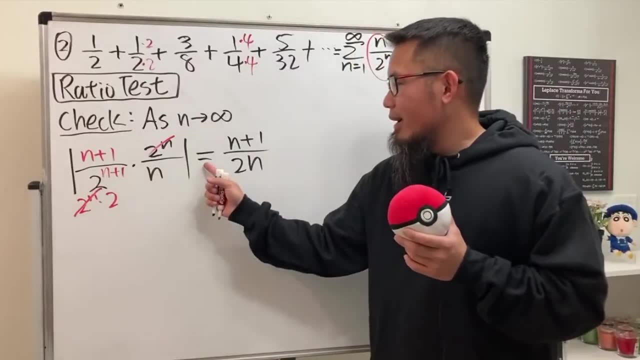 And check this out. Everything inside is positive, So the absolute value doesn't matter anymore. And yeah, that's pretty much all I have to say. Oh, yeah, and I just did algebra, So this is still equal. Well, what does this do? 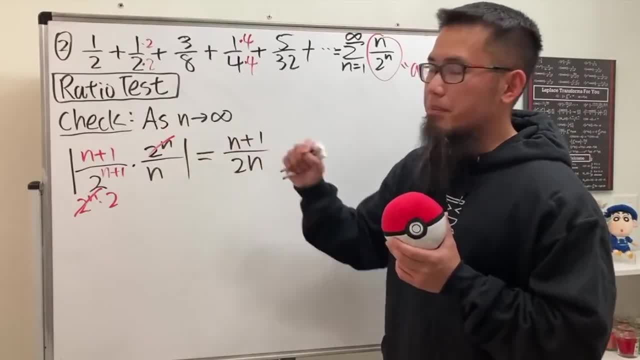 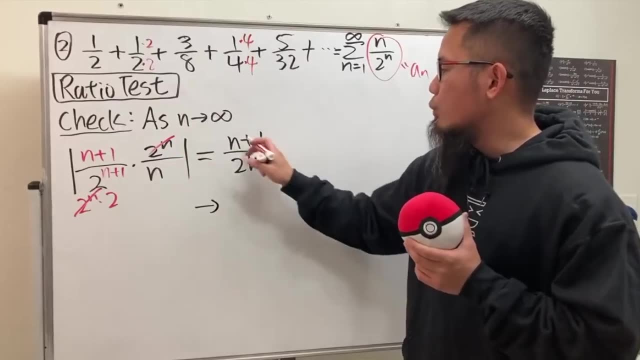 Remember we still have to take the limit. For you to take the limit, please draw an arrow. So this right here as n goes to infinity, n plus 1 over 2n. we just need to care about this and care about that. 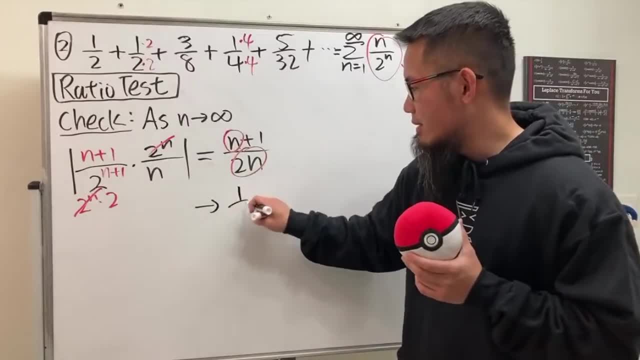 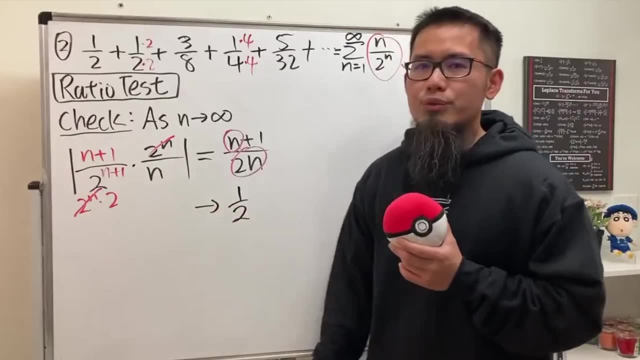 So we get 1 over 2.. Alright, And we took the limit. that's why we draw the arrow. And now don't just say, hey, this is 1 over 2.. You will have to say 1 over 2 is less than 1.. 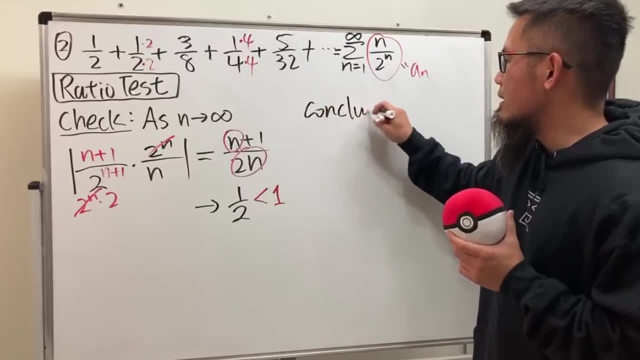 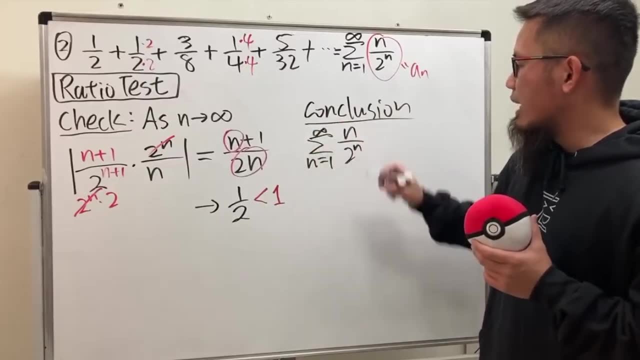 Therefore we can draw a conclusion and this is very nice. The conclusion is this series, the series as n goes from 1 to infinity, n over 2 to the n, this thing right here converges and we know this is by the ratio test. 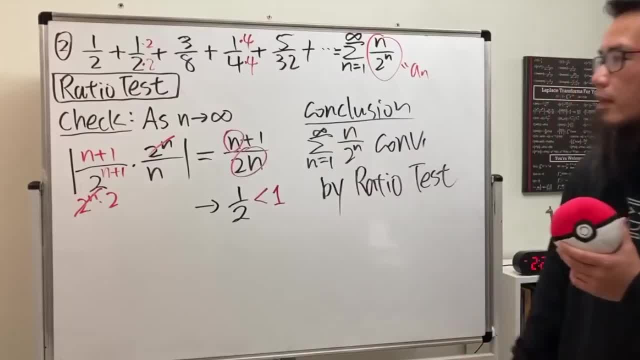 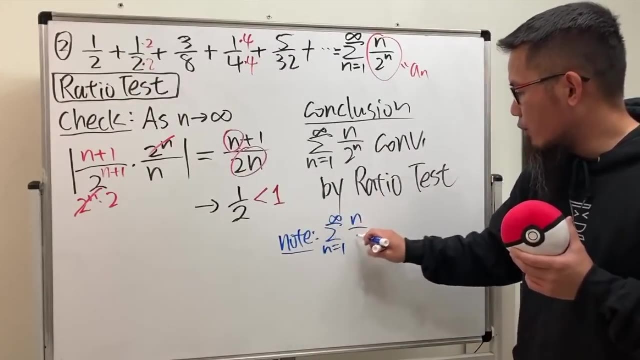 Right By the ratio test. Alright, so that's it, And in fact I would actually like to mention, as you can see, this right here we can actually say the series as n goes from 1 to infinity, n over 2 to the n. 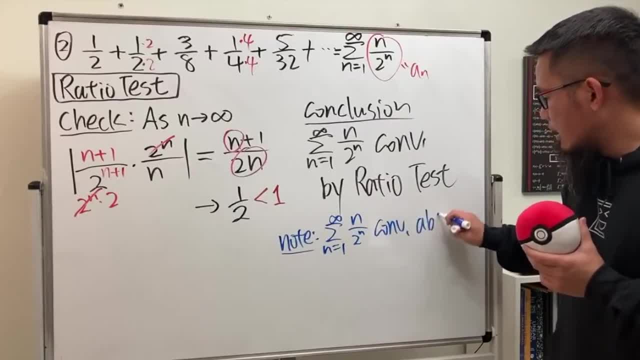 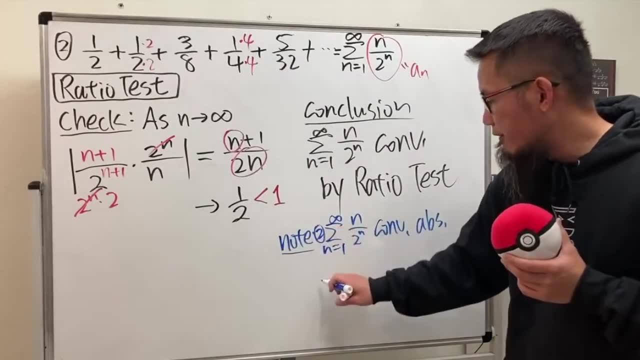 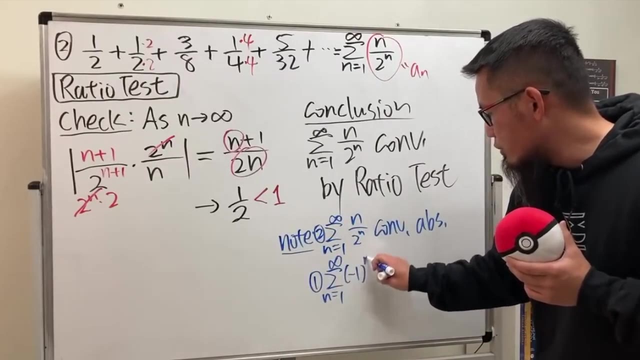 this, right here, converges absolutely, because we did a ratio test and we have the absolute value. And this is question 2, right, In fact? question 1, the series as n goes from 1 to infinity negative 1 raised to the n minus 1 power. 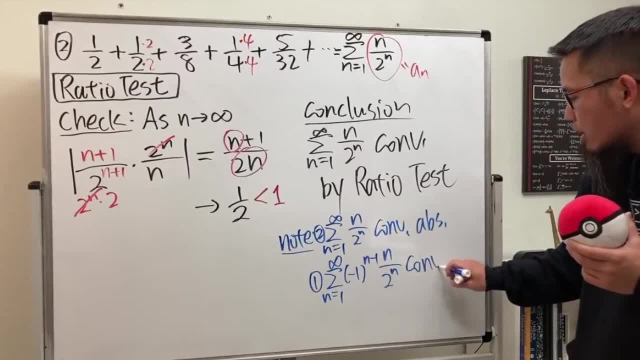 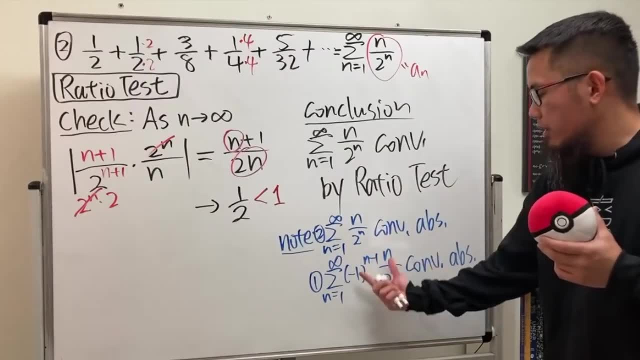 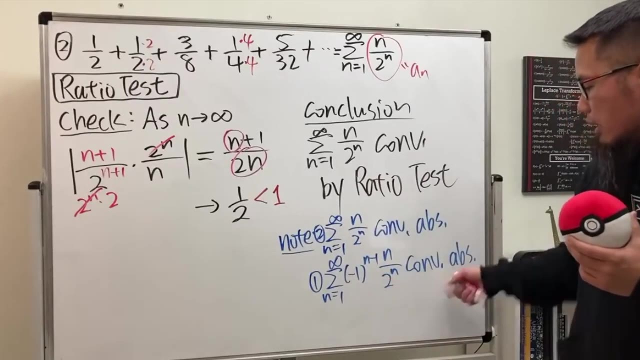 n over 2 to the n. this right here also converges absolutely. Why? Because if you apply the absolute value, this right here is the same as that. this right here converges. of course, that means this right here converges absolutely. 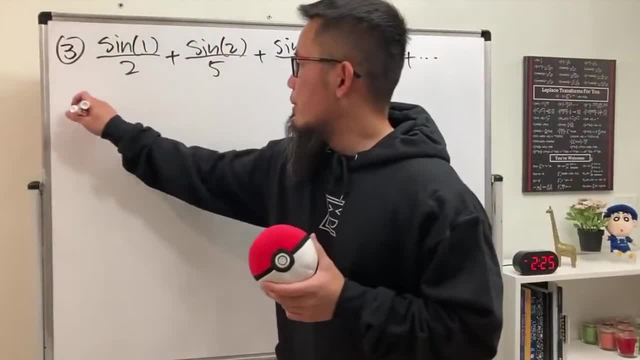 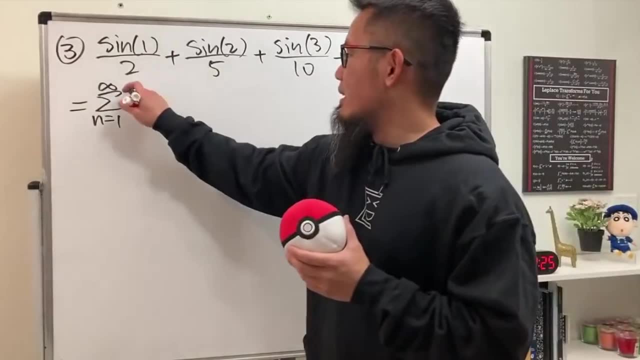 So we get 3 over 2 plus 1, which is 2 over 2, and again the formula is n over 3.. Real quick. what's the formula for this? n goes from 1 to infinity. what's the formula for the terms? 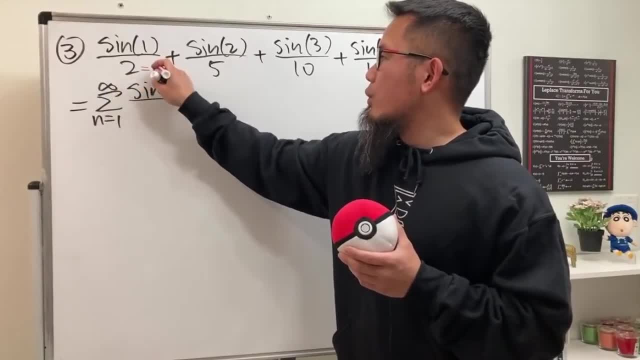 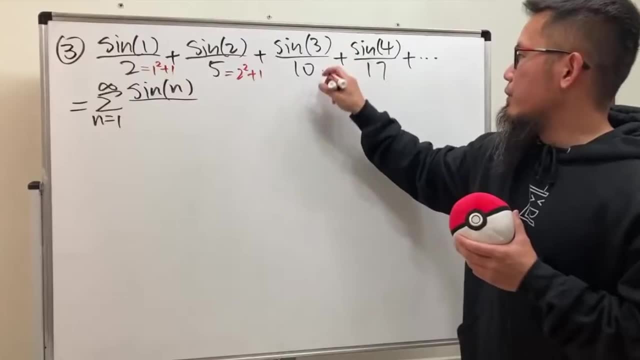 The formula is just sine of n over. notice this right here is the same as 1 squared plus 1, that's how we get the 2.. And if you square this and then you add 1,, you get the 5.. 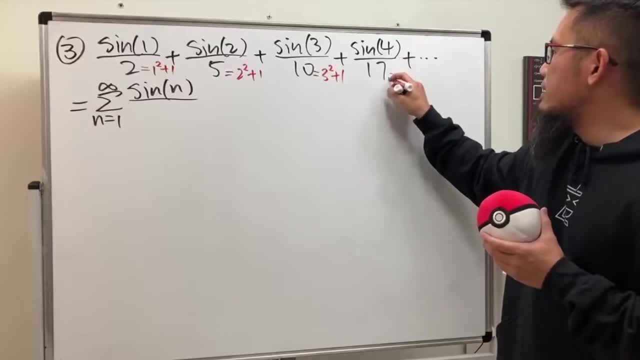 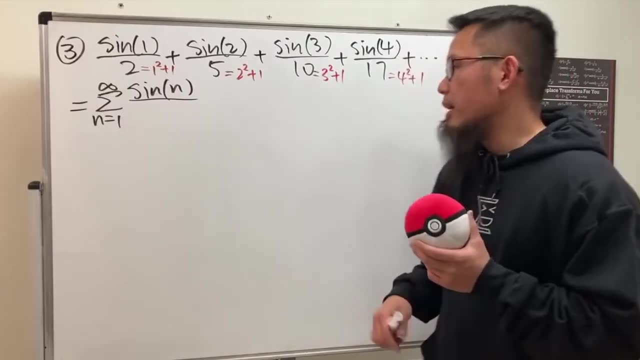 And then if you square the 3,, Likewise, this is 4 squared plus 1.. Again, you should be familiar with the perfect squares, right? Just keep that in mind. So all this is just n squared plus 1, like so. 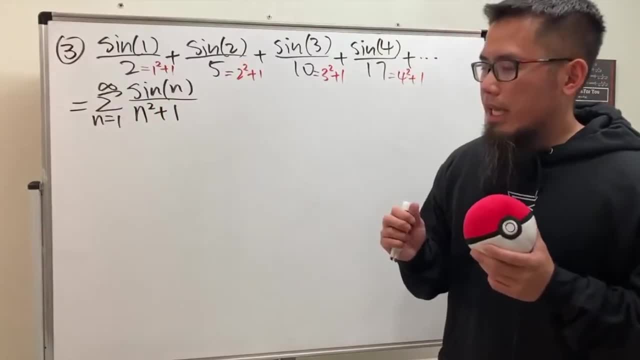 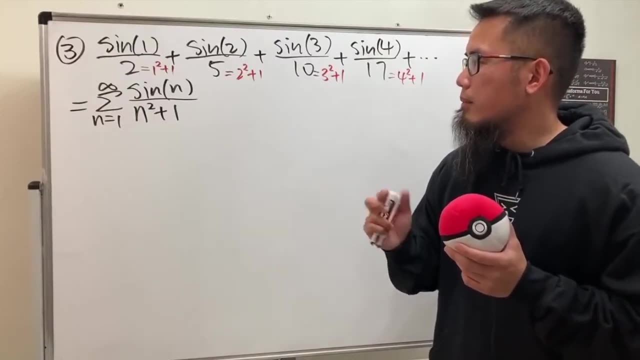 Now here is the deal for this, though We cannot use comparison yet, right? And maybe no ratio test, maybe no root test, because, yeah, just go ahead and try it. I don't think it will work out nicely. 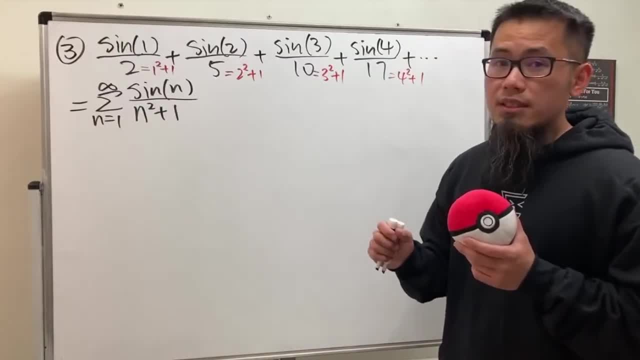 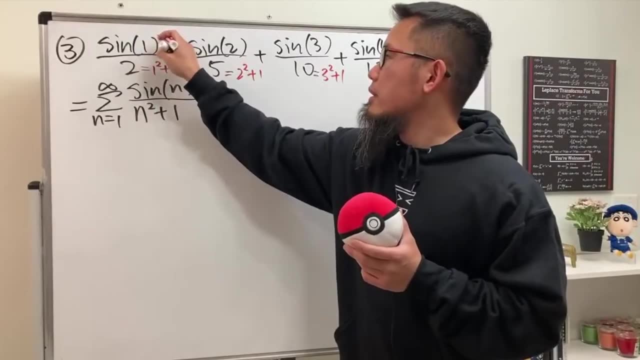 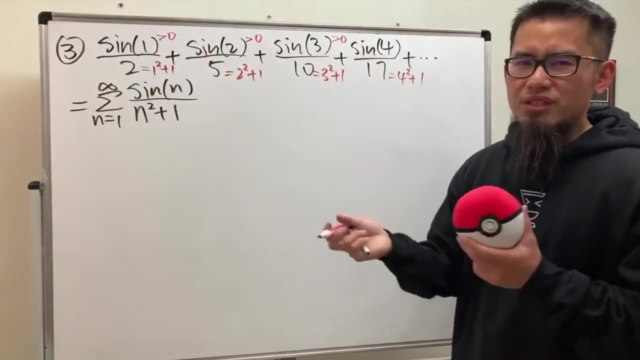 Anyway, we cannot use the comparison test because if you look at sine, sine of 1 is positive, Sine of 2 is positive, Sine of 3 is positive. You can just enter down the calculator if you would like, and make sure that you are in gradients though. 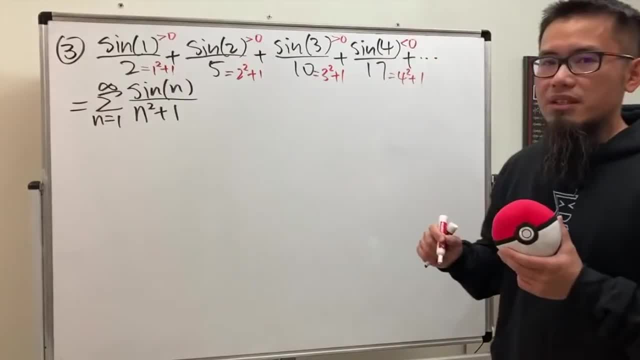 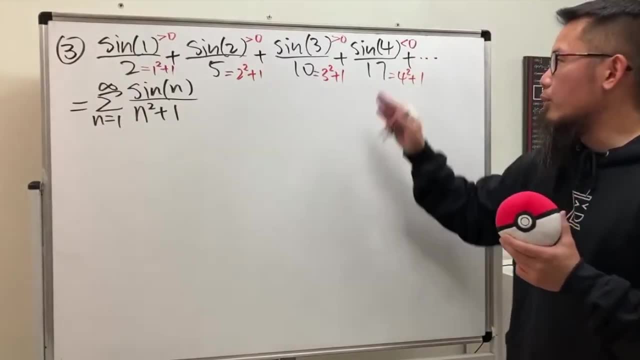 However, sine of 4 is actually negative. 4 is bigger than pi, It's actually on the third quadrant, and then you actually get a negative y-value. So sine of 4 is actually negative, And then sine of 5 is also negative. 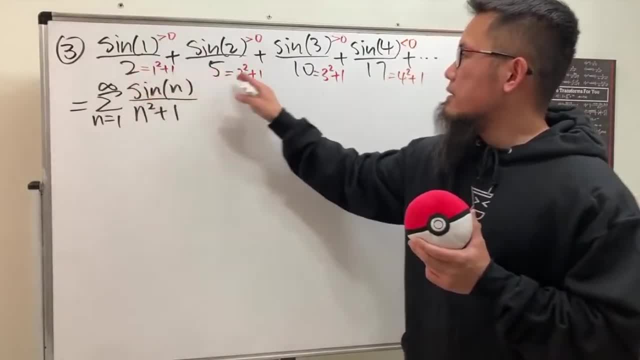 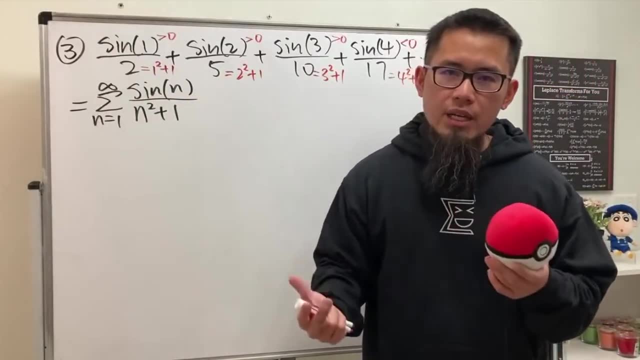 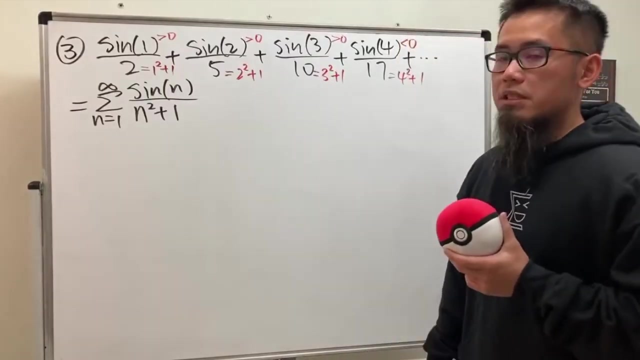 So the trouble of all this is that positive, positive, positive, negative, negative, and then it's not really alternating in the sense that we want. So we cannot use the alternating series test either. So that's bad. So the way to deal with this is that recall. 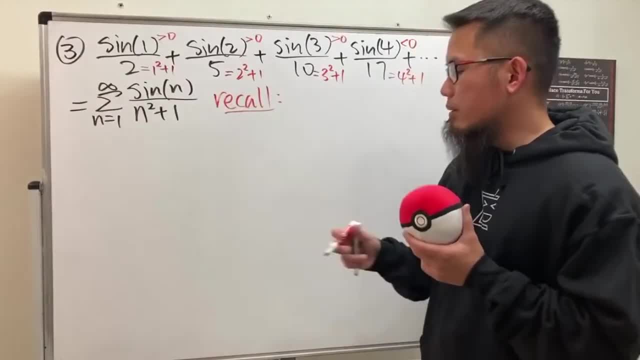 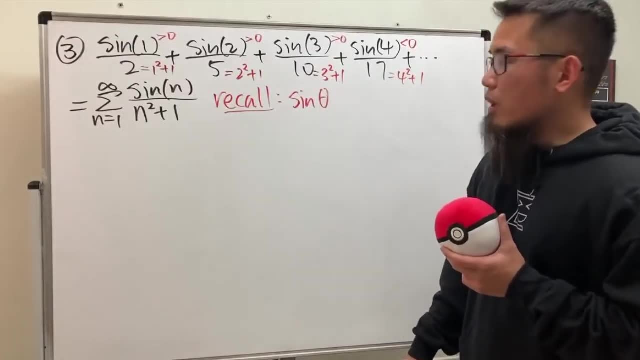 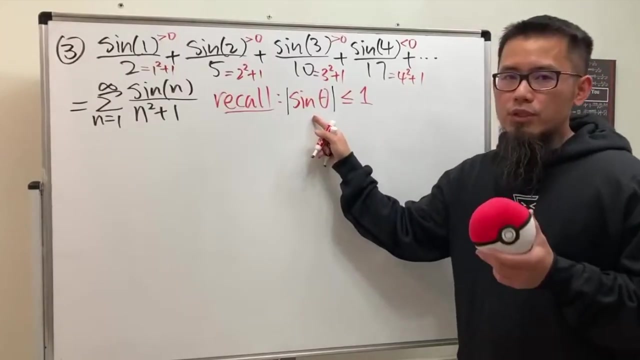 whenever you have sine cosine. one of the most important inequalities is that whenever you have sine of any angle, we know the absolute value of this is going to be less than or equal to 1.. Of course, we are talking about real numbers. 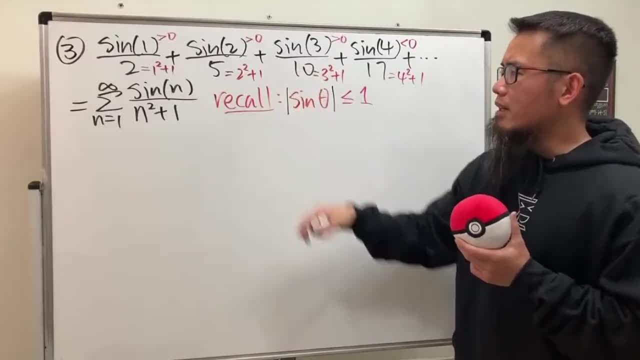 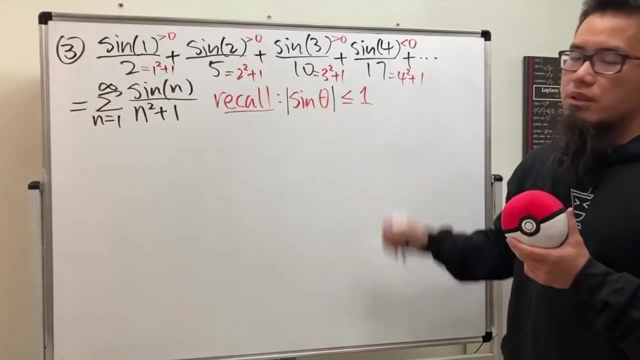 So when you have sine cosine in your formula, in your AN, always keep this in mind. The absolute value of sine or cosine, well, it's less than or equal to 1, right, The biggest value is equal to 1.. 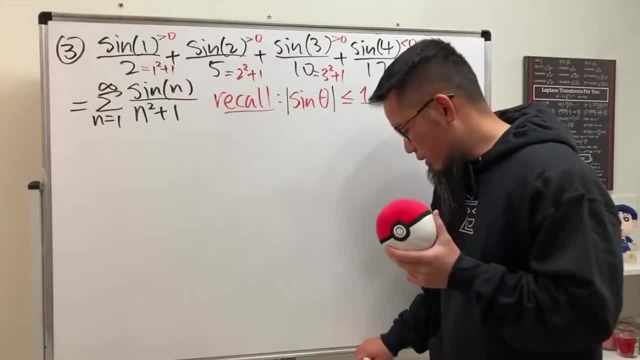 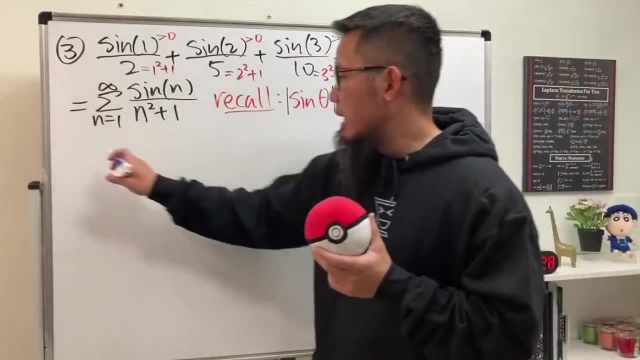 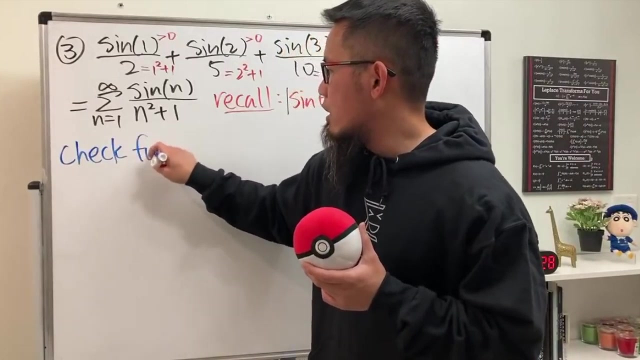 So this is going to be really helpful and this is how we are going to do it, Even though the question doesn't ask us that if it converges absolutely or not, but because we want to utilize this right here, it would be a better idea if we check for absolute convergence, right. 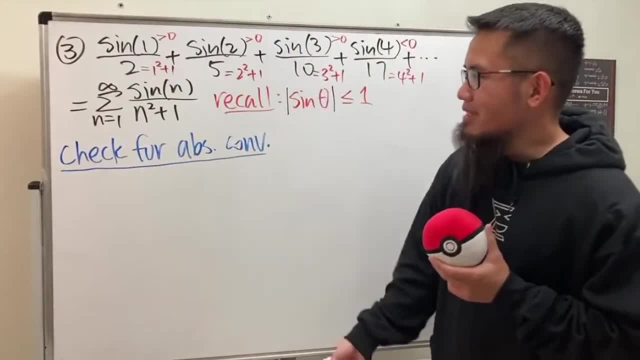 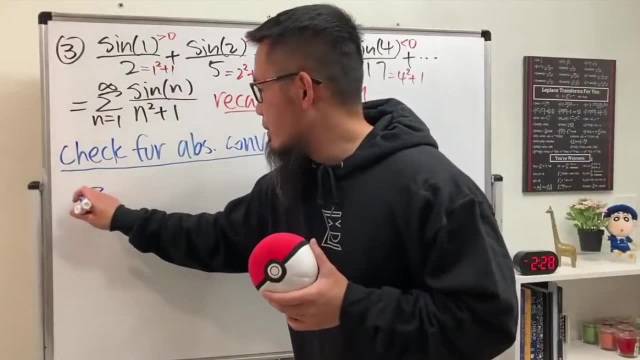 So this is absolute convergence And if it works, then we can say that it converges absolutely. So just kind of play around with the words And to do so we are just going to see. okay, here we have the series, as n goes from 1 to infinity. 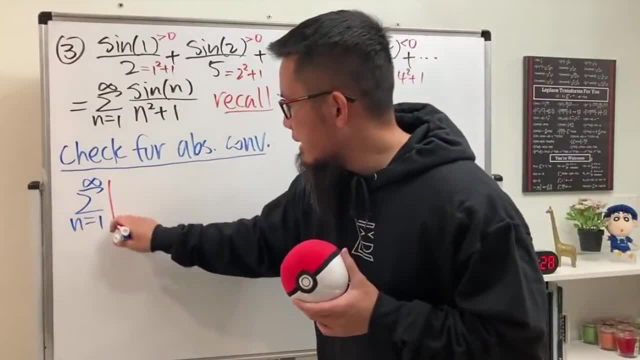 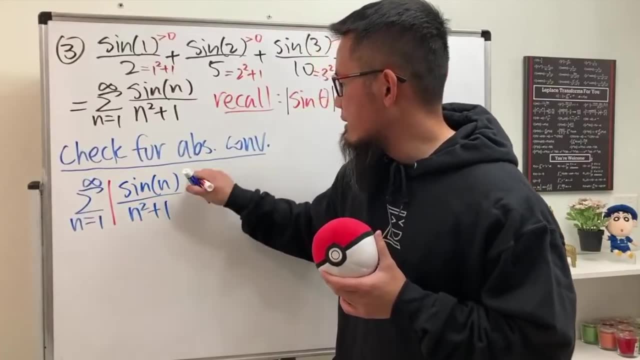 And when you are checking for absolute convergence, you apply the absolute value with this. So you have the sine n and then you have the over n squared plus 1, like so Right, So let's go ahead and just write down all the steps. 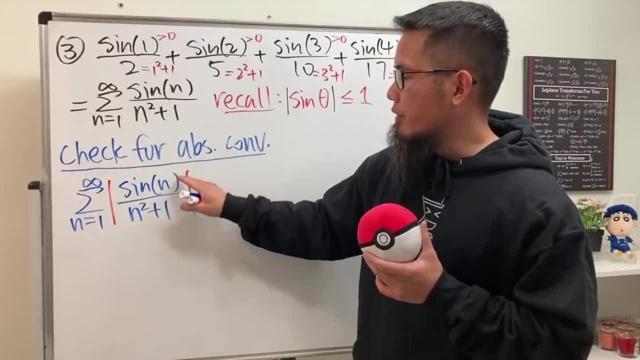 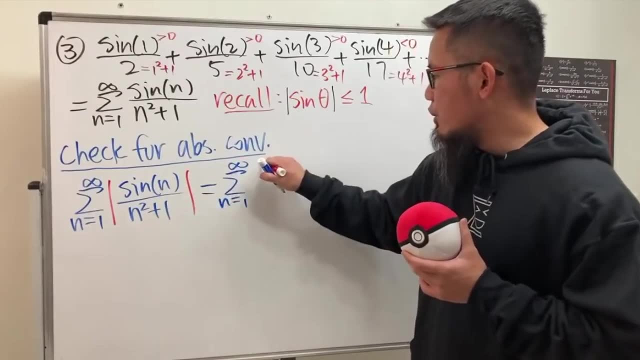 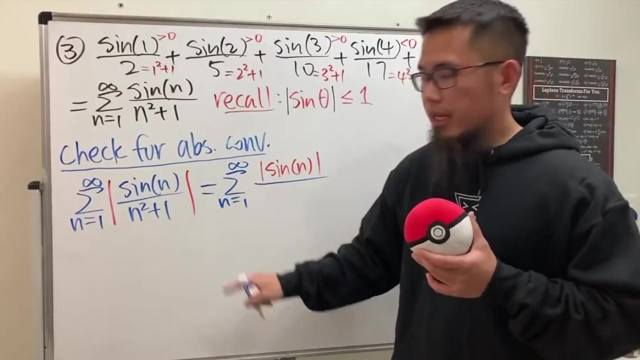 First the absolute value of a quotient. it's the absolute value of the top over the absolute value of the bottom. So this is the same as the series, and we will have just the absolute value of sine n on the top and then over the absolute value of n squared plus 1.. 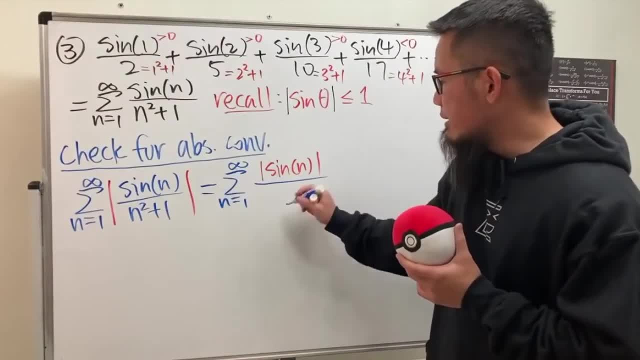 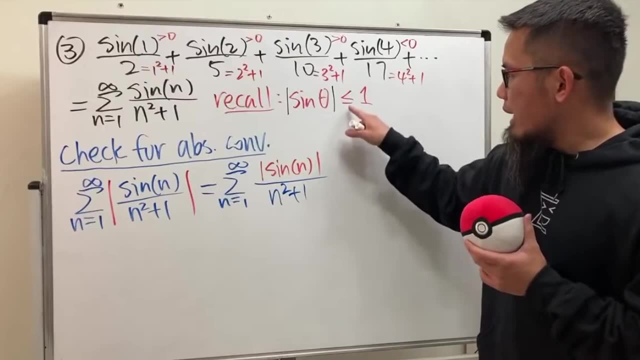 That's always positive, so you don't need the absolute value for that. So we'll just write it down as n squared plus 1.. And now check this out. Thanks to this, we can go ahead and just use an inequality right now. 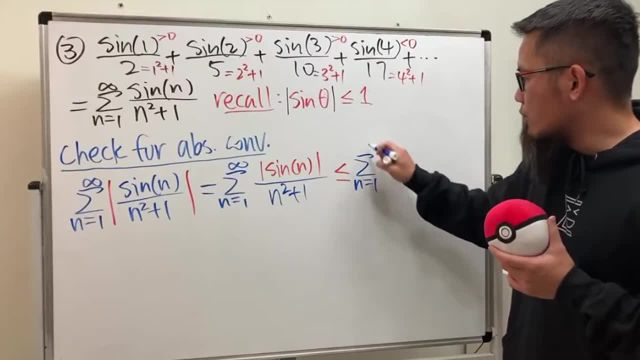 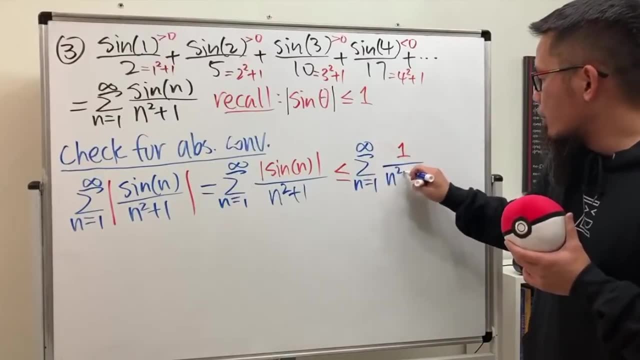 and say this: right here is the series, as n goes from 1 to infinity, And we'll replace the whole thing right here with just 1.. And then this is over n squared plus 1.. Right, So that's really good. 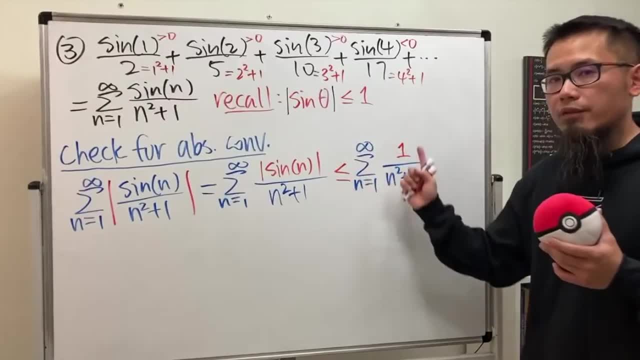 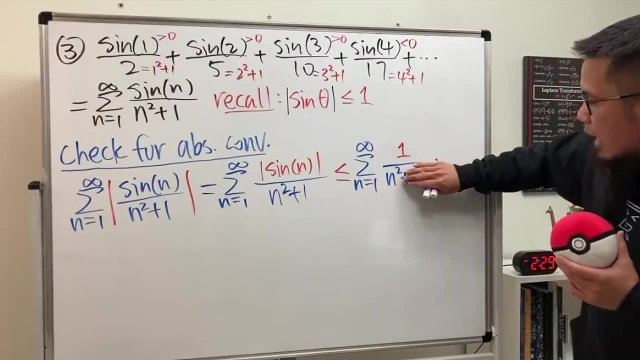 And now you just have to observe and test out if this series converges or not. But this is not so bad, because this is just 1 over n squared plus 1.. If we don't have the plus 1, you will see. 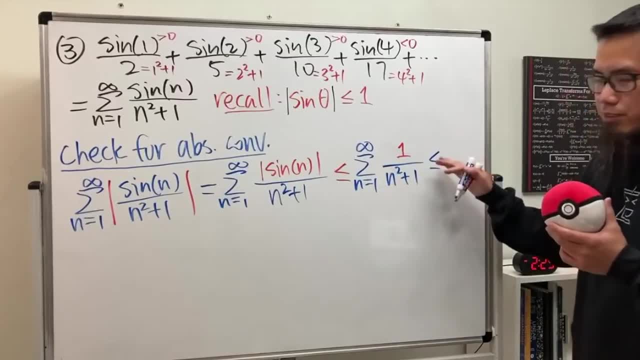 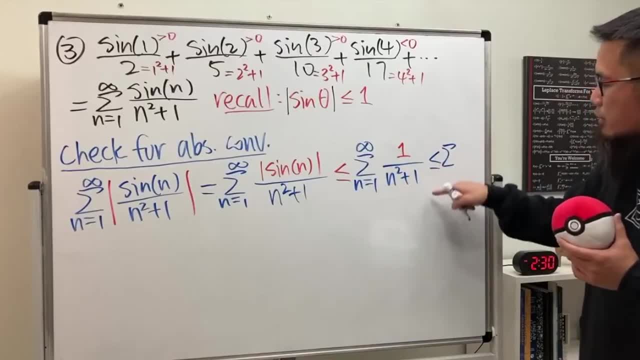 well, less than or equal to doesn't matter. This right here is actually less than or equal to. when n goes from 1 to infinity. 1 is still on the top, but you can just take away the 1 on the bottom. 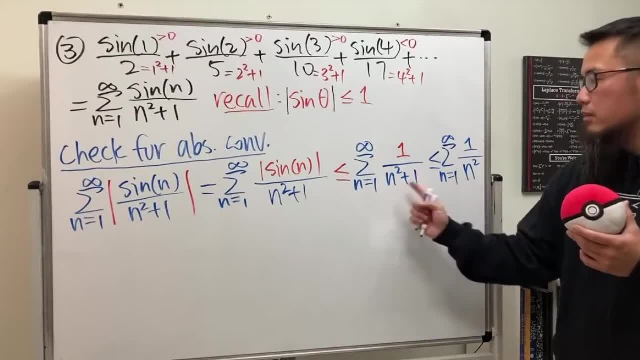 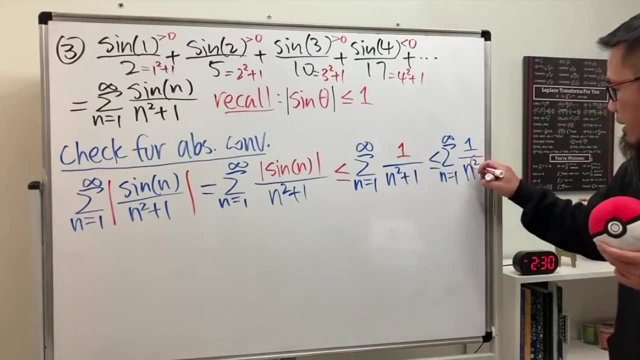 This is true because the bigger that you have on the bottom, the less. this is Right. So this right here. as you can see, we'll just indicate that Here we have a nice conversion p-series, because p is 2, which is greater than 1.. 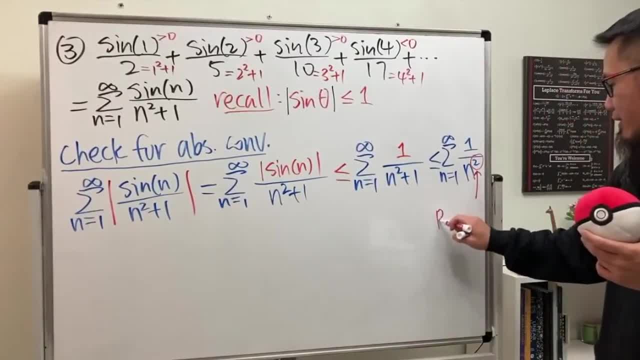 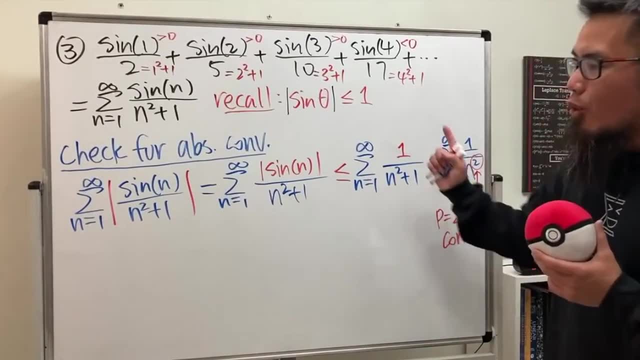 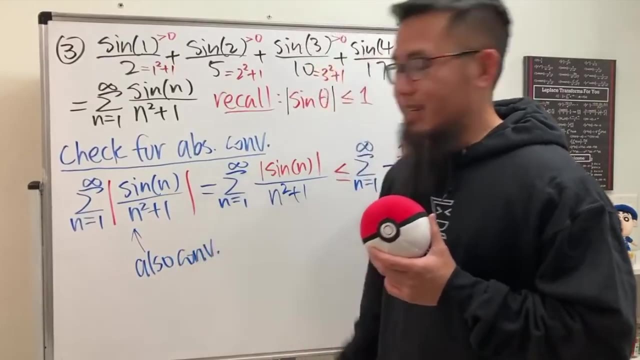 Just write this down better: p is equal to 2,, which is greater than 1.. Therefore this right here converges. So that means we can go back to here and say that this right here also converges And this right here converges. 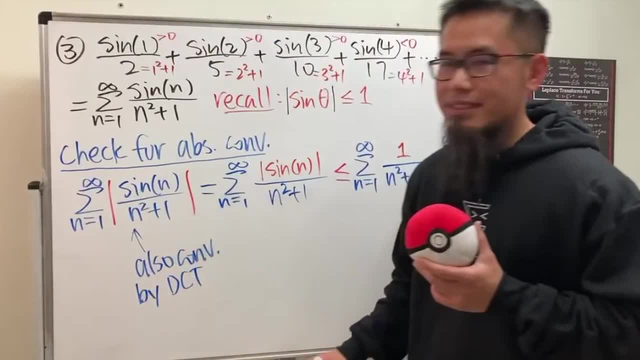 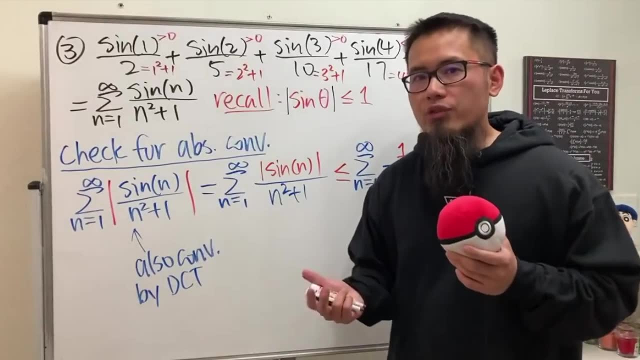 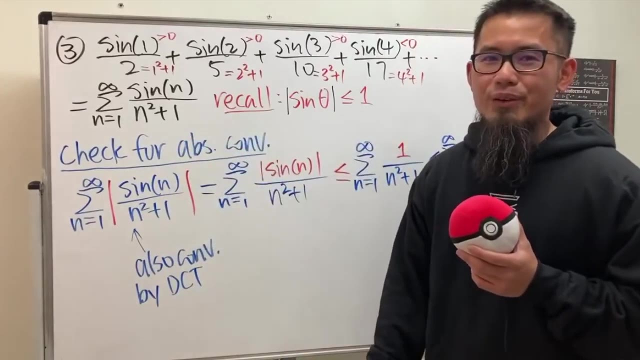 Why By the direct comparison test? Because we use inequalities right here. All right, So now, as you can see, we check for the absolute convergence and we see that this right here converges. So that means, of course, this right here converges as well. 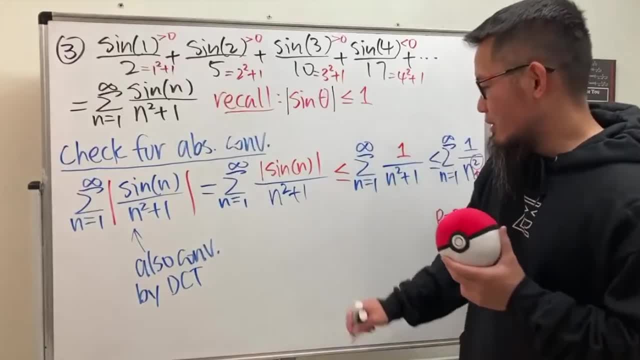 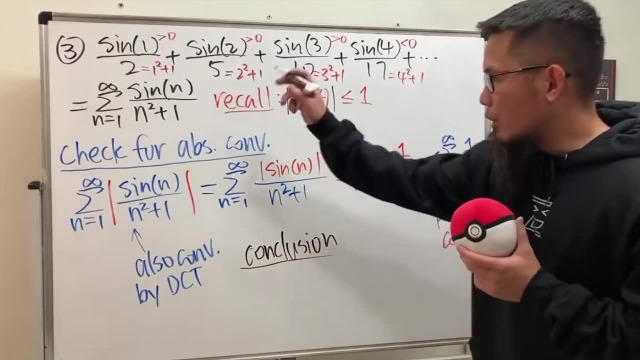 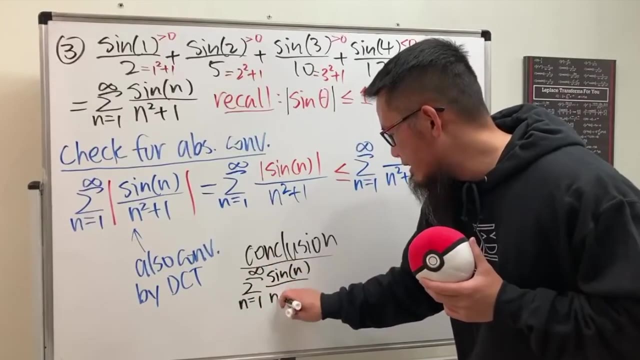 Better yet you can say this right here: converges absolutely. So here is the conclusion. I wanted to say Conclusion, I will write that down: The series as n goes from 1 to infinity sine n over n squared plus 1.. 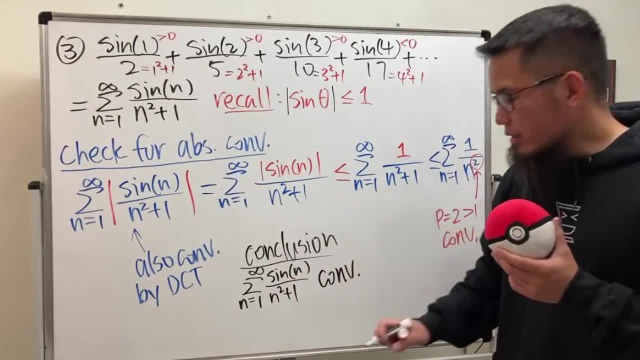 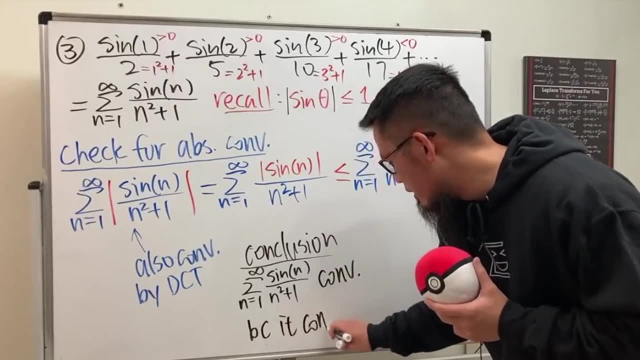 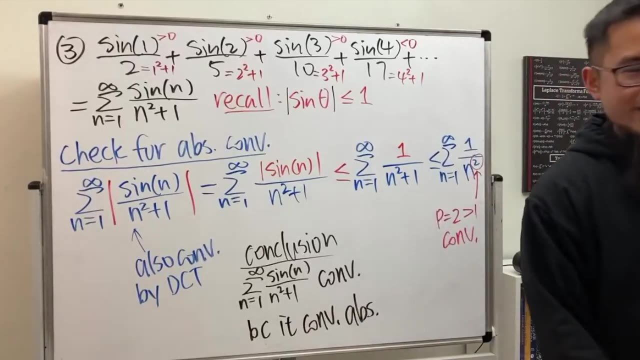 This right here converges, And the reason why is because it converges absolutely. So, because it converges absolutely, All right. So that will be the write-off for that question. One thing I want to make a note before we do anything else. 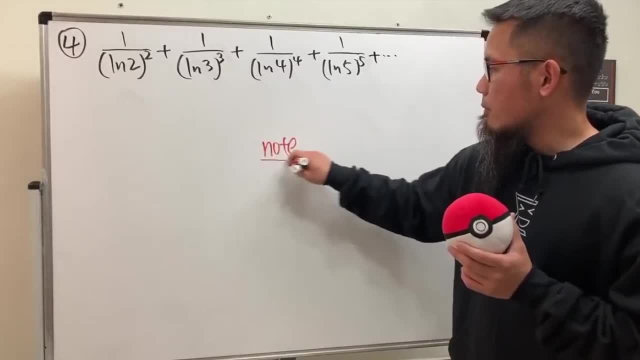 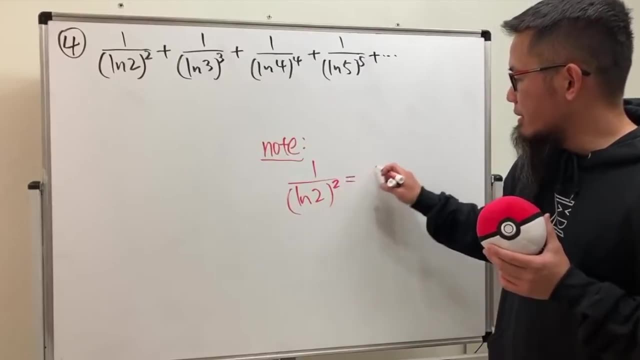 is that note right here? All right When we have 1 over L right. When we have 1 over L right, ln2.. Parentheses like this to the second power. this means 1 over ln2 times ln2, because the 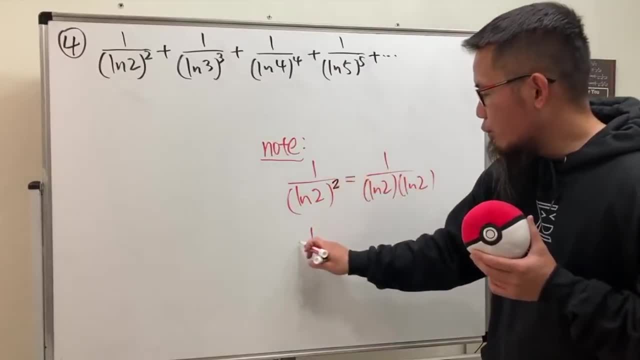 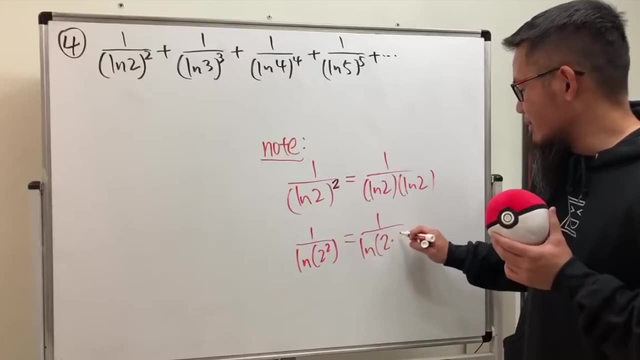 2 means you do this twice. When you have 1 over ln2 squared, this means 1 over ln and then 2 times 2.. And for this, right here we could do it as you can bring the 2 to the. 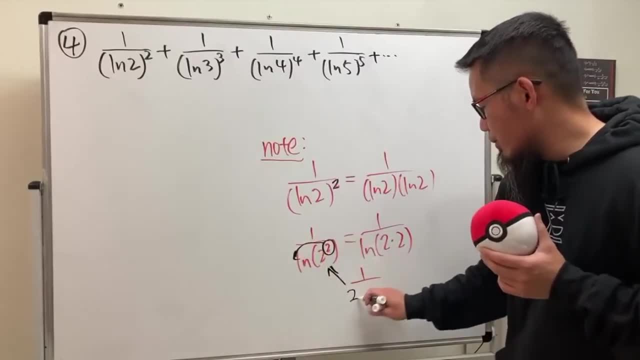 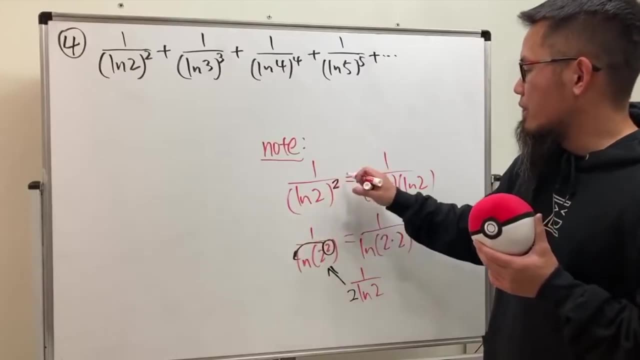 front, which is 1 over 2 ln2.. But if you have the 2 right here outside of the parentheses, we cannot bring the 2 to the front. So don't say this right here: it's the same as 1 over. 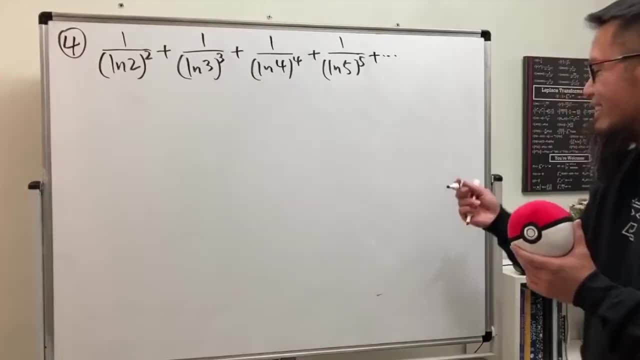 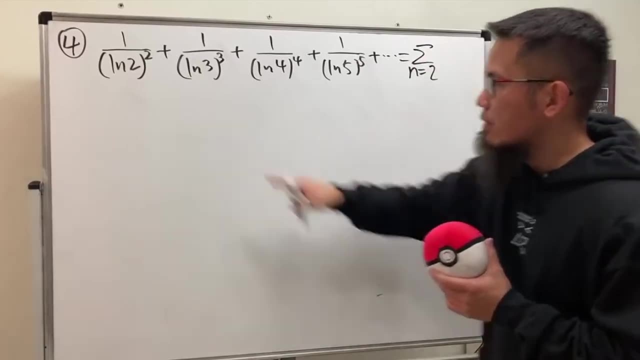 2, ln2, right This and that they are not the same. So this right here. not so bad, you have this number and that number the same. So this is just. series n goes from 2, starting with 2, to infinity 1 over ln n. 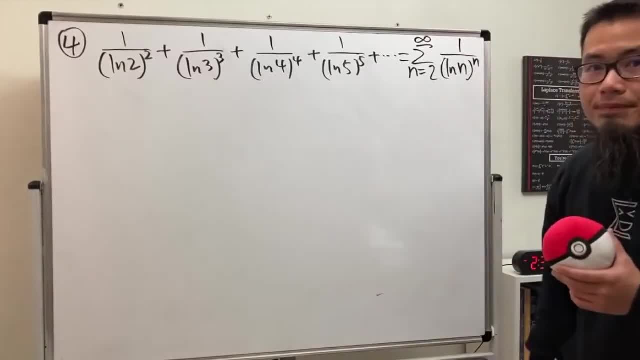 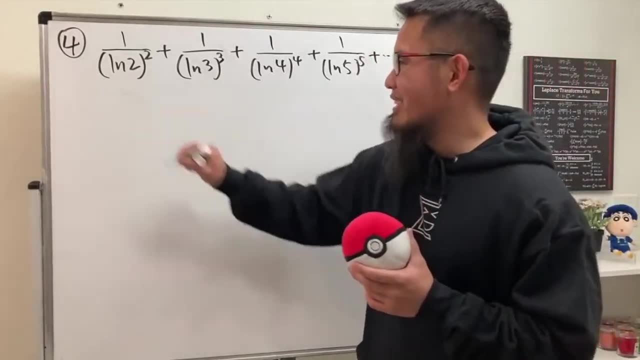 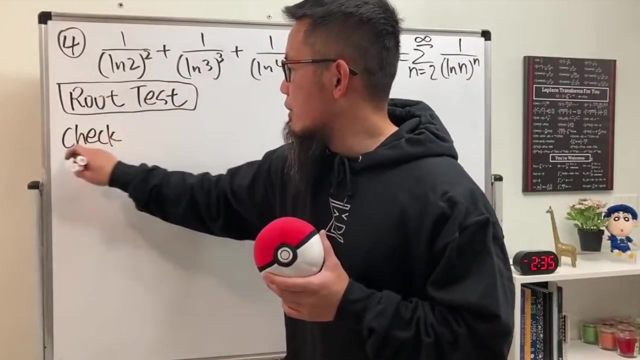 And then you raise that to the nth power. right Now you see that we have the n in the power. This right here root test will work And it works really nicely. so let's go ahead and do the root test. This right here we have to just to check the limit. 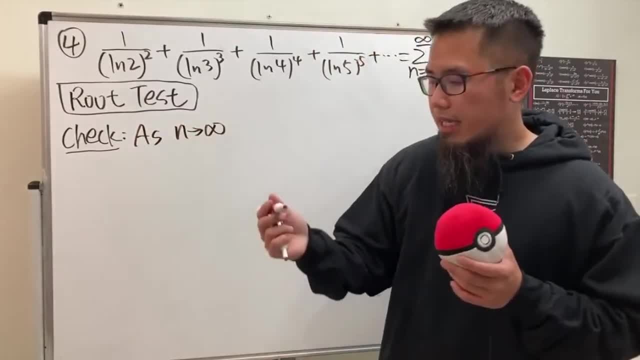 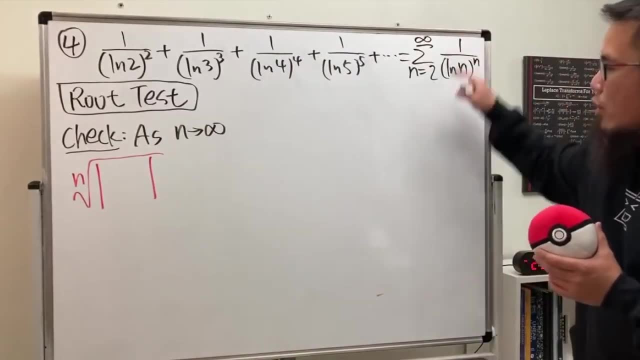 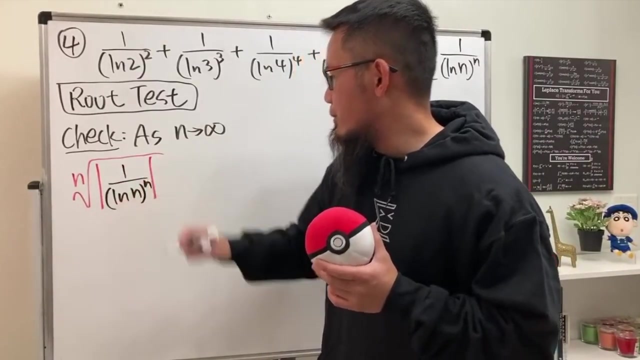 right. So I'll just say, as n goes to infinity and we will take the nth root and technically we apply the absolute value and we are going to draw in Expression in here. So that will be 1 over ln. n raised to the nth power. 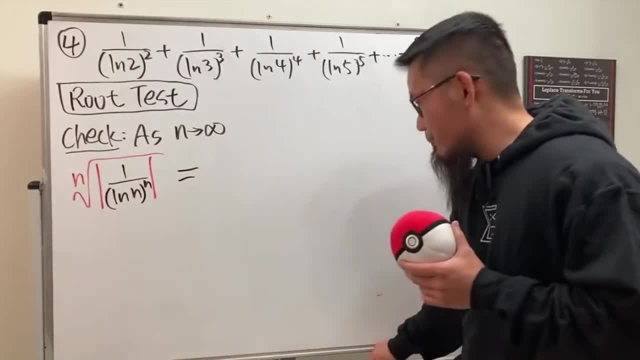 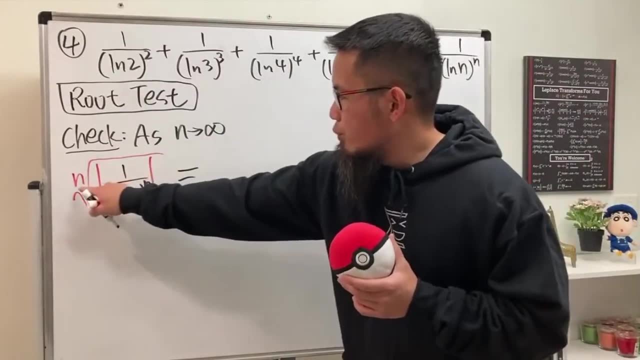 All right. the nice thing about this is that I'll cross this out. Actually, no, I will show you guys the work. The nice thing about this is that when you take the nth root of 1, it's just 1, and we can drop the absolute value because everything inside is positive. 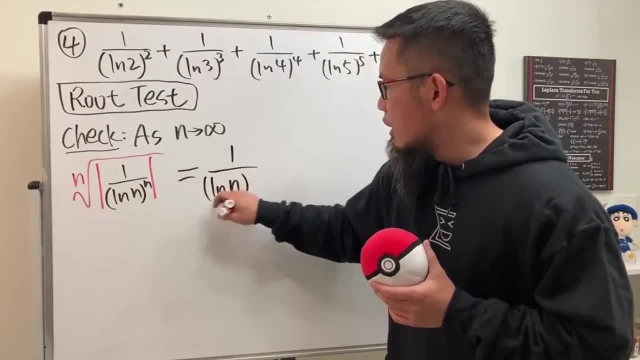 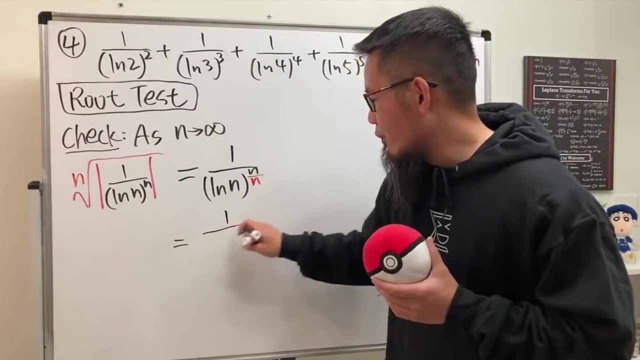 And then this right here becomes ln n raised to the nth power. It's raised to the n, but you divide it by the nth power. Of course that can also be 1, so we are just looking at 1 over ln n And you know what, Remember, we are taking. 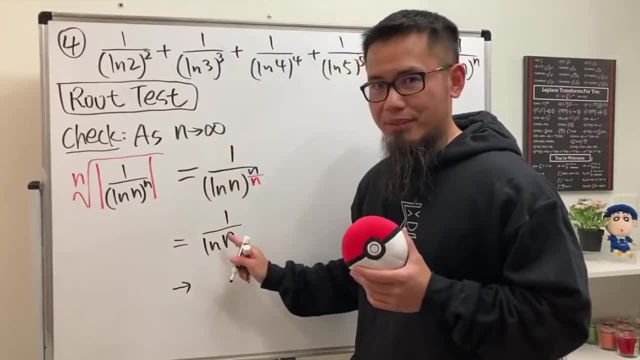 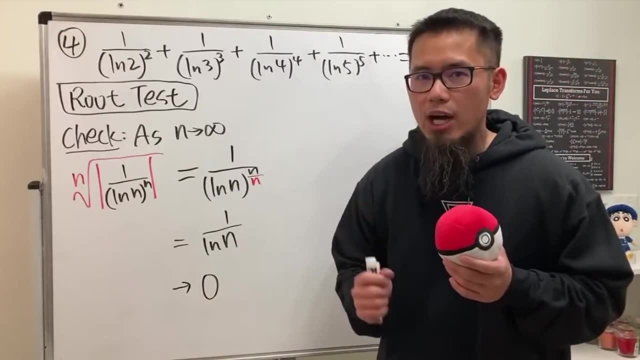 the limit as n goes to infinity. This is where you go to infinity. 1 over infinity is nicely equal to 0.. Now we have 0.. Does 0 help? Yes, it does. And again, do not just say: we have. 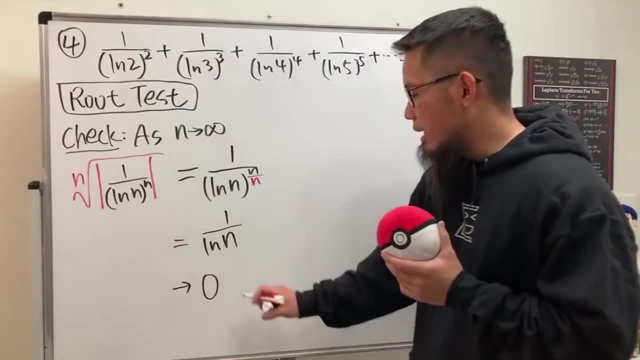 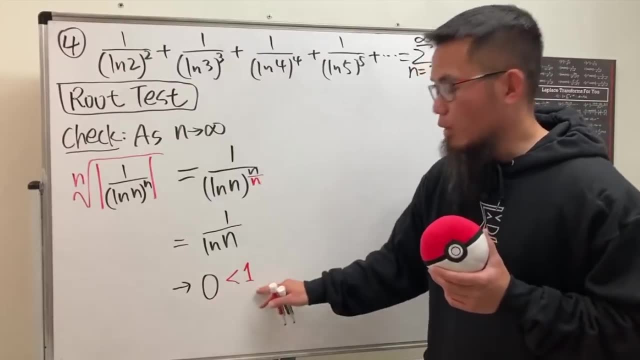 0 and draw a conclusion. You have to mention that because 0 is less than 1, you have to use this as an indicator right. 0 is less than 1.. And by the root test, when you have the limit, end up to be less. 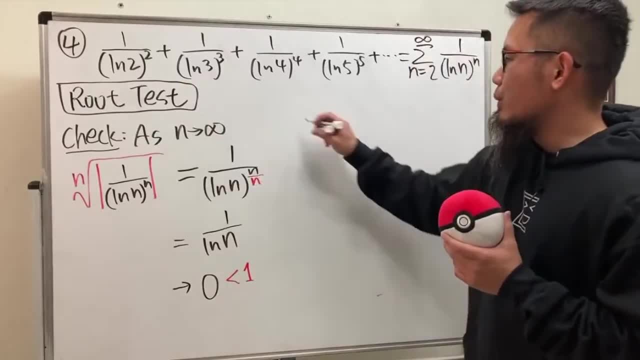 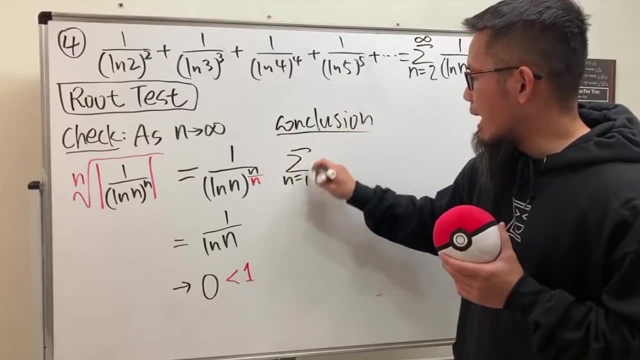 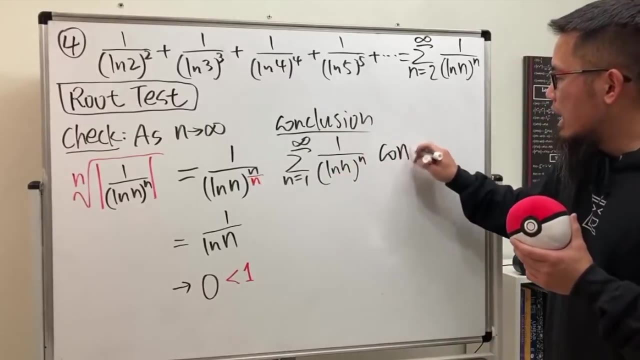 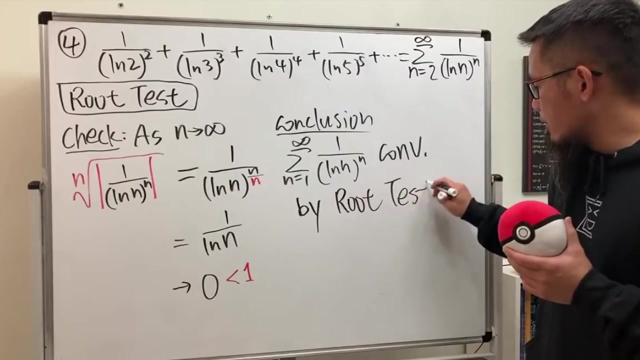 than 1, this series converges. So we will just say: here is the conclusion. The conclusion is that the series as n goes from 1 to infinity, 1 over ln, n raised to the nth power, this right here Converges and we will just say by the root test, Right, So that's it. If you take a look, 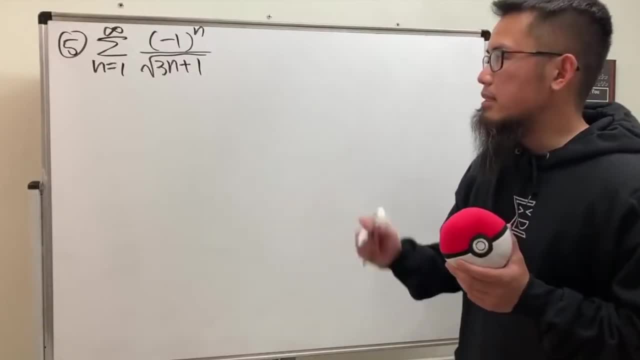 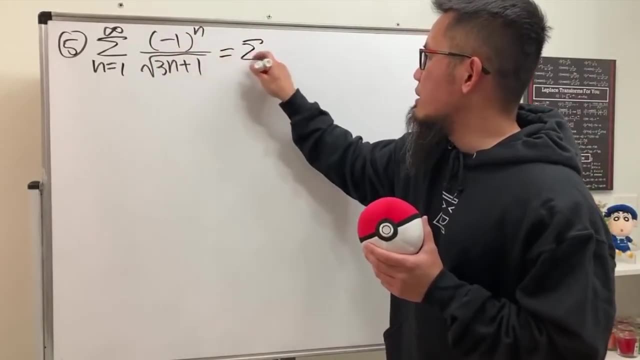 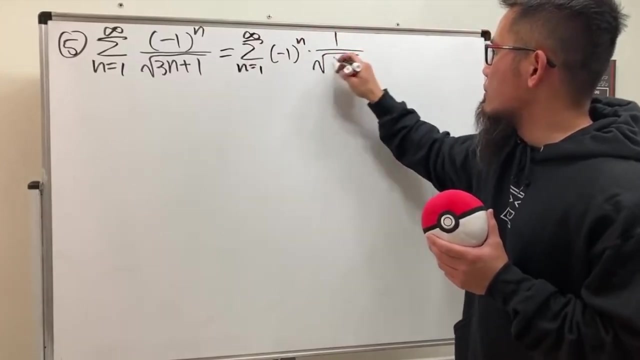 right here. if the question is only asking you: does this converge or not? Well, because we have this factor here, we can just put that aside and say: this is the series as n goes from 1 to infinity negative, 1 to the nth power times 1 over square root of 3n plus. 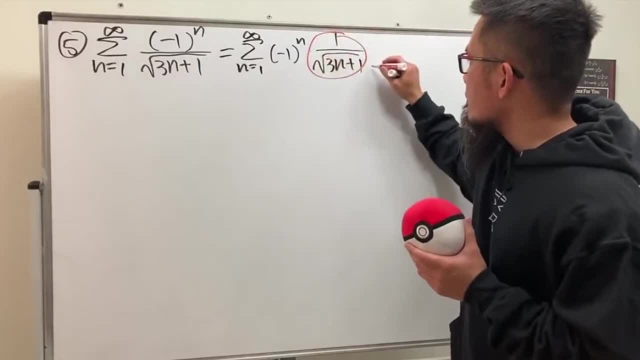 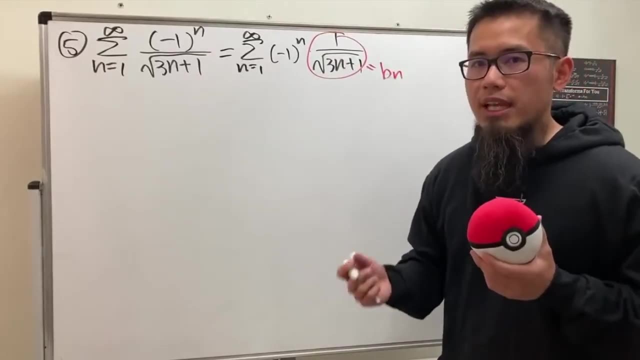 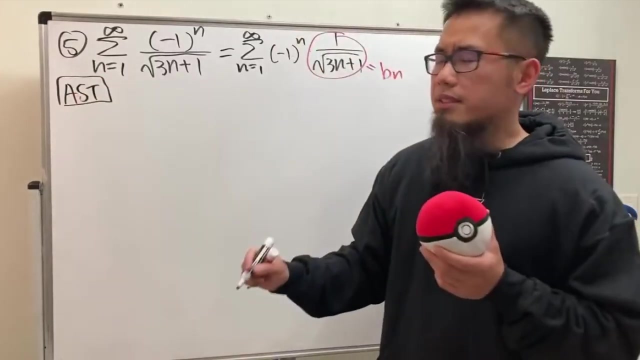 1. And you can see that this right here is exactly the bn that we are looking for, So we can just go ahead and use the alternating series test because, again, thanks to that factor- So let me just write that down right here- For the alternating series test, we have to 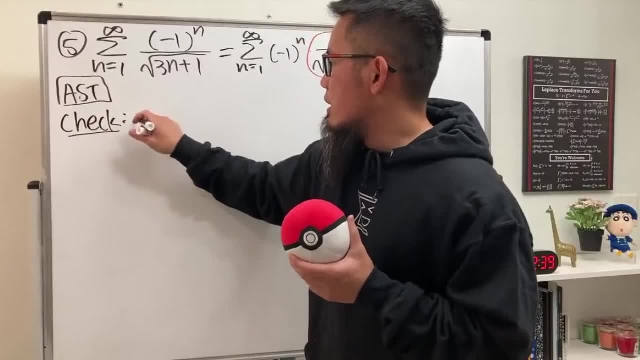 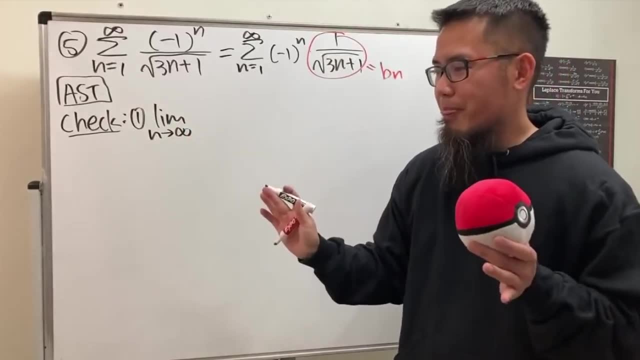 check two things. First thing, we check if the limit as n goes to infinity. See, I wrote down this again, but I really just don't know why. Okay, The ratio or the root test I just said as n goes to infinity, Anything else, I just 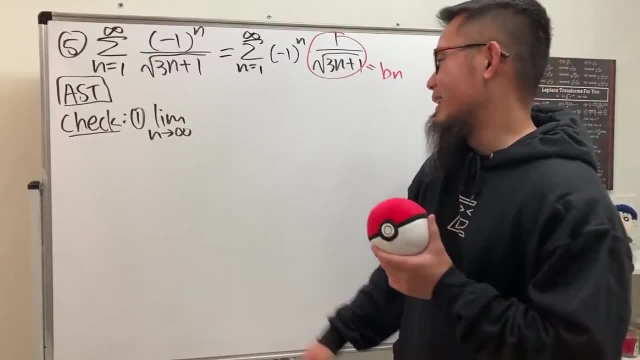 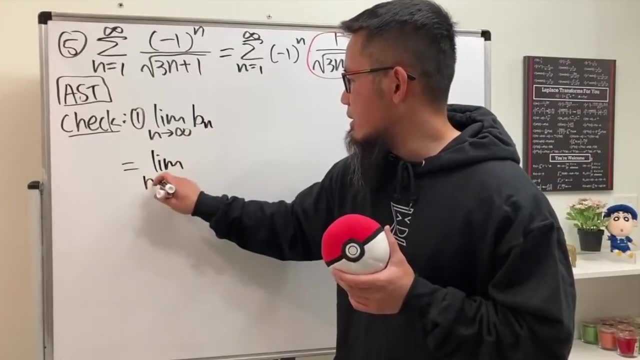 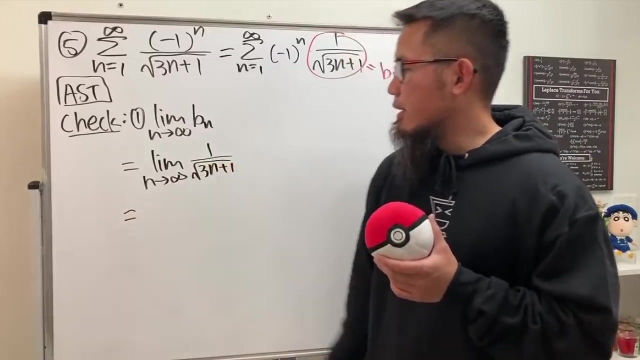 put down my ym. I don't know why I apologize. Anyway, take the limit of bn right And let's see, this is just the limit, as n goes to infinity 1 over square root of 3n plus 1.. When you 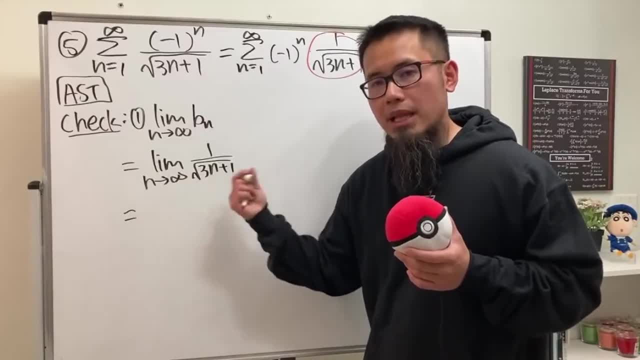 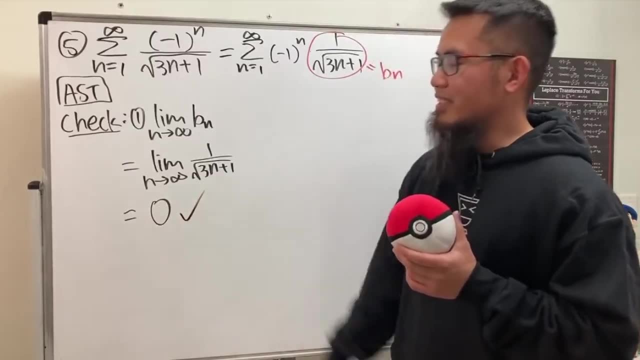 put infinity to here: 3 times, infinity is infinity. plus 1 is still infinity. and you take the square root, it's still infinity. So this is just the limit, as n goes to infinity, but 1 over infinity is equal to 0. So this right here checks. So it's pretty clear to 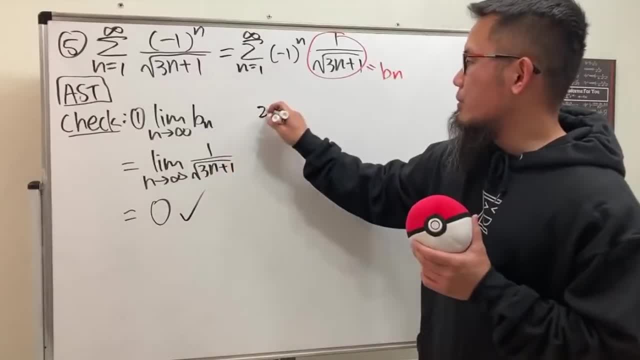 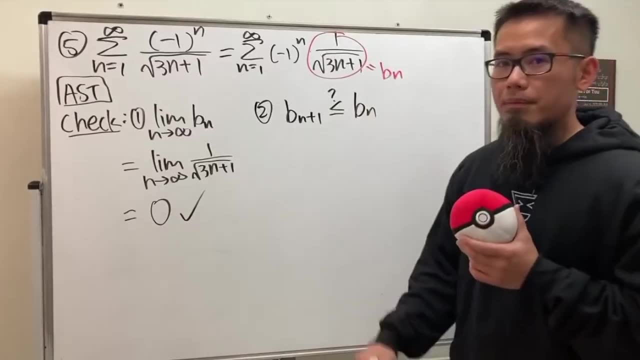 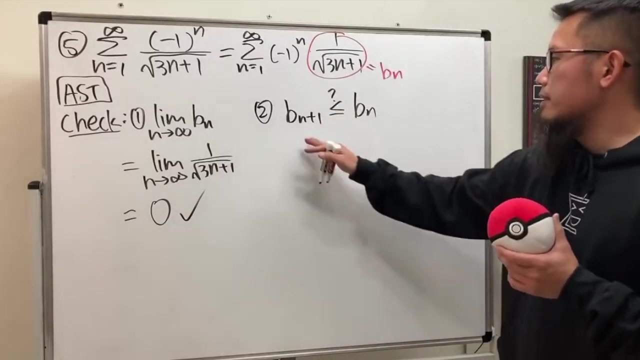 just go from here to here. Number two: we are going to check if bn plus 1 is less than or equal to, but we don't know yet bn. This means we have to make sure that bn is legitimately decreasing, at least non-increasing in this case. Anyway, this right here is 1 over square. 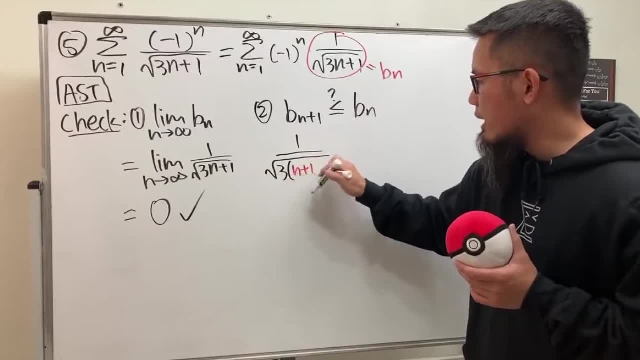 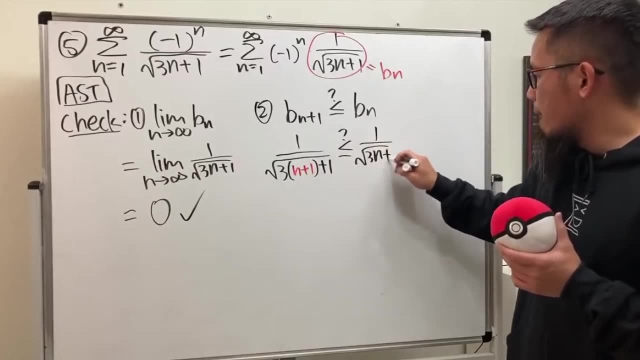 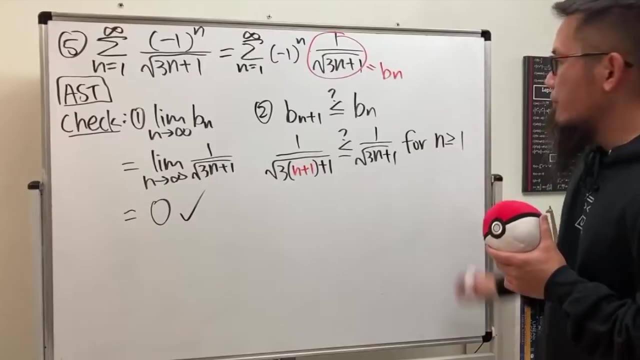 root of 3 times infinity. So what's the eigenvalue of bn? Let's take this to the next step. Let's see what's going on here. So bn is equal to 1 over square root of 3n plus 1 over square root of 3n plus. 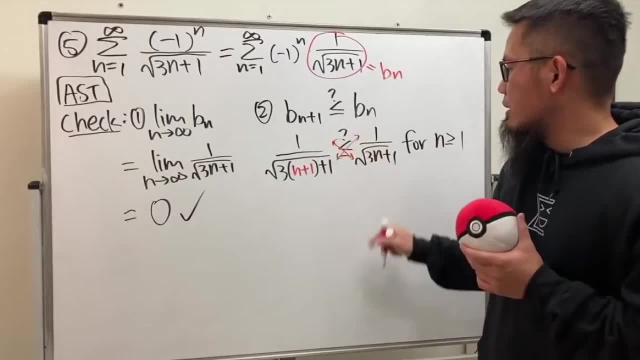 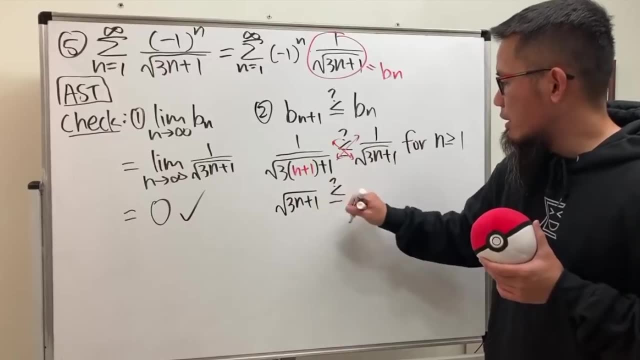 infinity. This is 4 times n plus 1, and then plus 1.. Is this less than or equal to bn, which is just the original? Well, it's true, but let me just show you guys more work so we can see this is legitimately true, right. 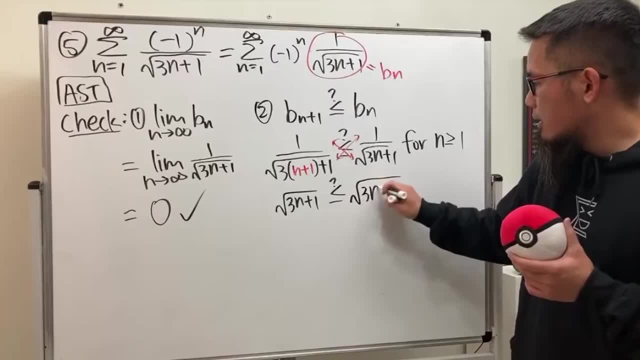 Alright, so we have this here. this x is equal to bn. I said that's not true, right? Anyway, just go ahead and cross multiply This times. that is square root of 3n plus 1.. Is this 3n plus 3, and then plus 1, which is plus 4.. 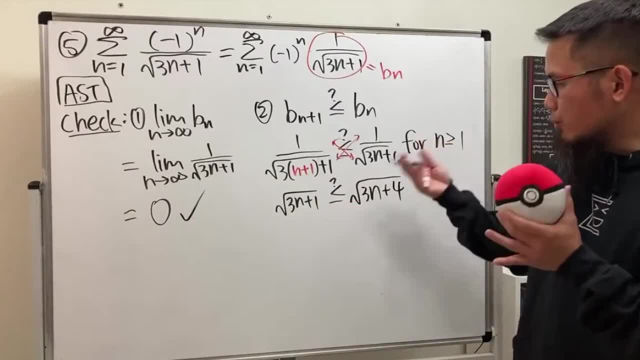 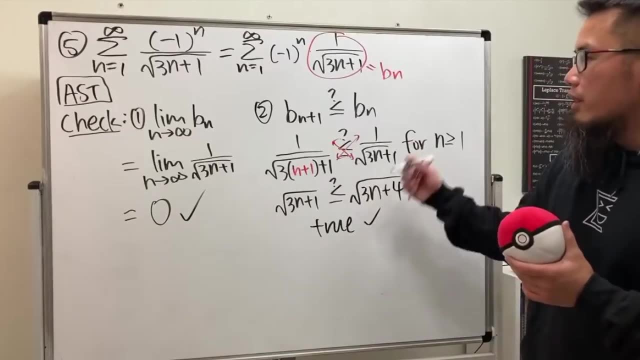 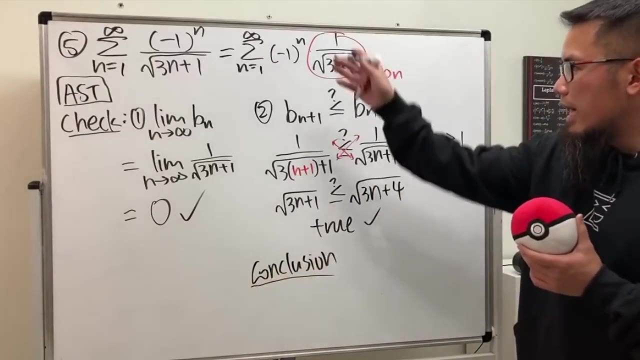 So it's really clear, right. So just do enough algebra to show it's true. So, of course, this is true Checks. So thanks, Conclusion, Conclusion, yeah, Conclusion, that the series as n goes from 1 to infinity. 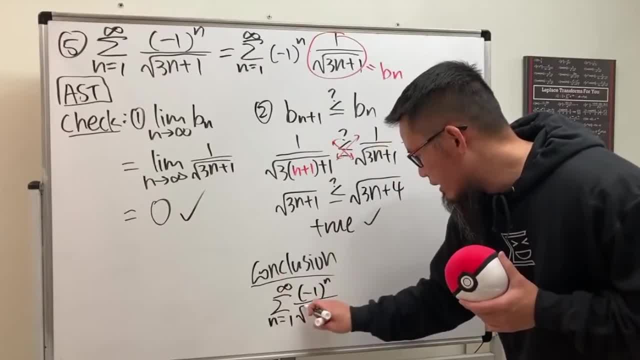 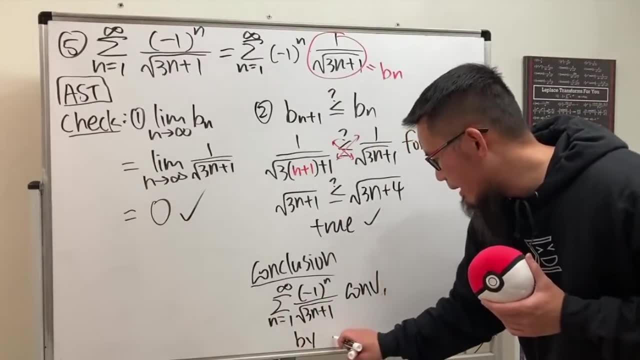 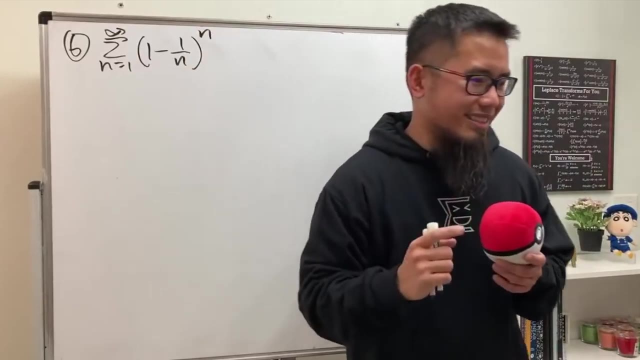 negative 1 raised to the nth power over square root of 3n plus 1, this right here converges y by the alternating series test. And that is it. You guys do this real quick. Does it converge or diverge? 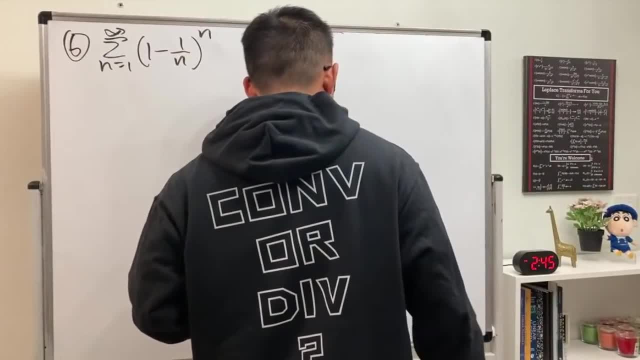 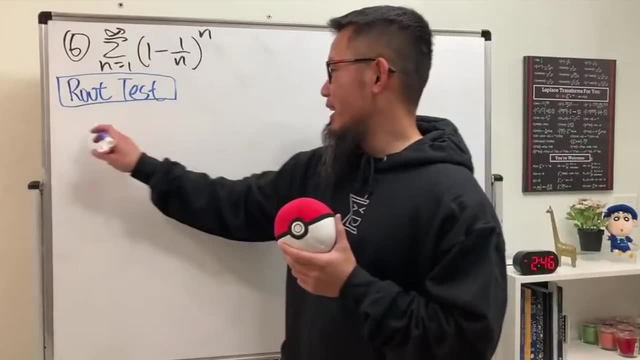 Again, this is the question. right, Converge or diverge? Just look at the back of my hoodie When you have the n in the exponent. maybe we should just do the test For the root. what we do is we check. 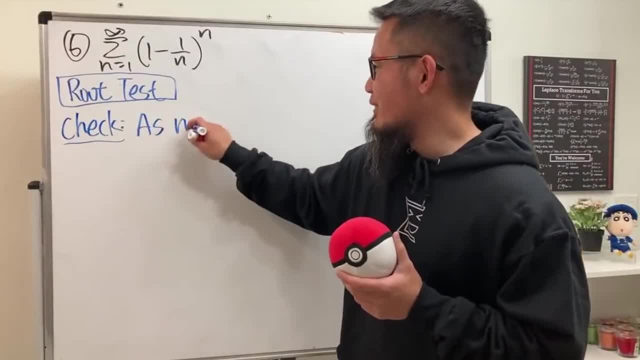 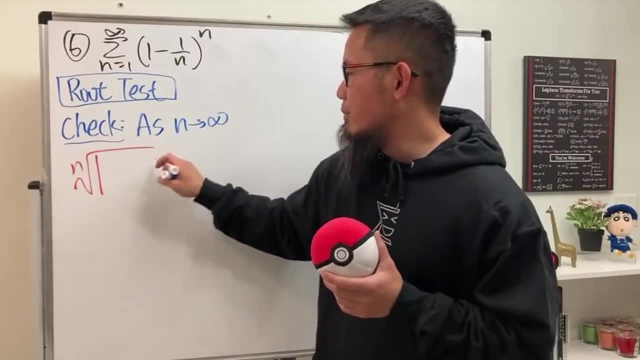 And now, here we go As n goes to infinity. I don't really know why. anyway, As n goes to infinity, we look at the nth root and you technically put down the nth absolute value, and you put this down here, which is 1 minus 1 over n. 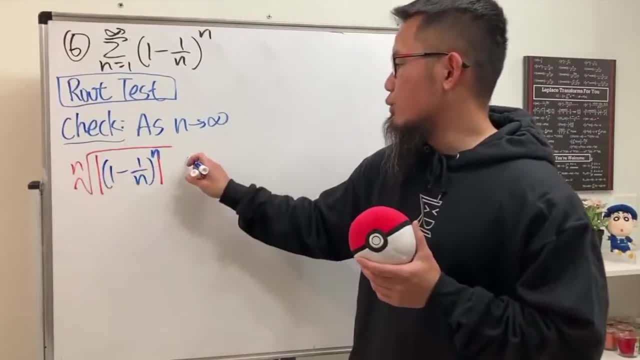 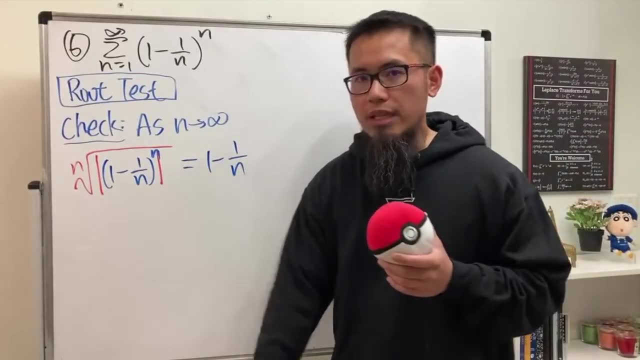 raised to the nth power. This and that can solve really nicely. So we just have 1 minus 1 over n And especially everything inside is positive. We don't need the opposite for you anymore. Well, as n goes to infinity. 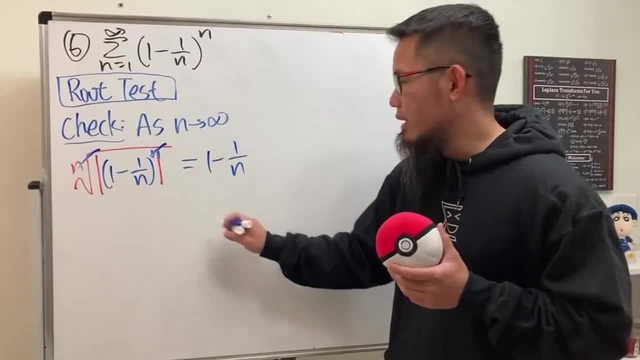 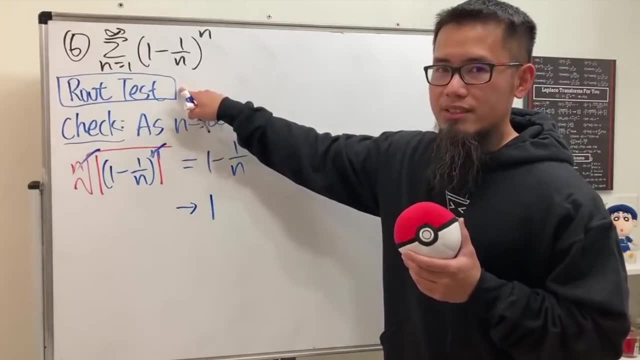 1 over infinity is 0. 1 minus 0 is 1. So this right here goes to 1. Uh-oh, We are trying to do the root test And we end up with 1. Does this 1 do us any good? Let me know. 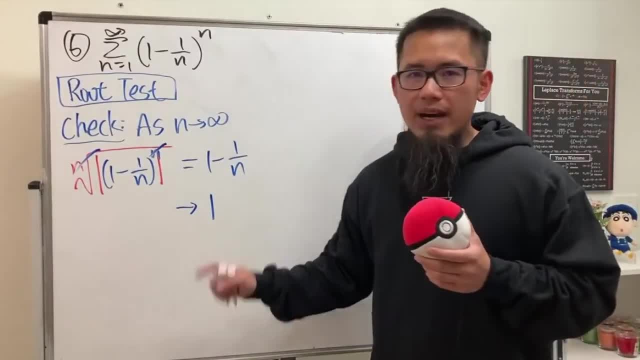 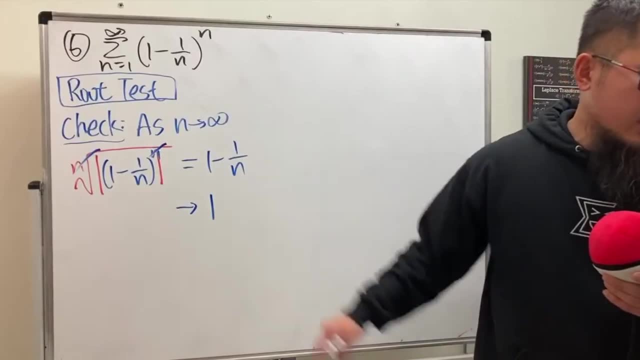 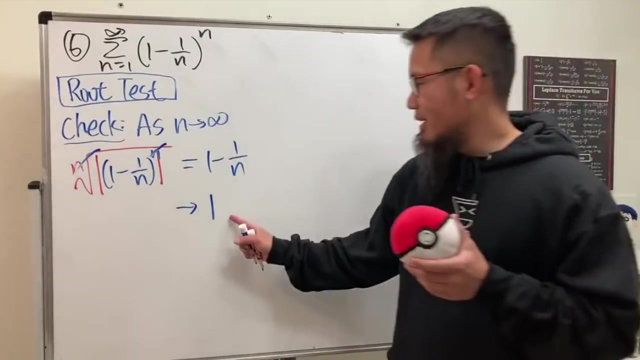 Well, 1 is not undefined. You are not supposed to use that term. 1 is not undefined. Does that do us any good? No, it doesn't right. No, it does not right, So I'll do this right here. I'm sorry if I pronounce your name wrong. 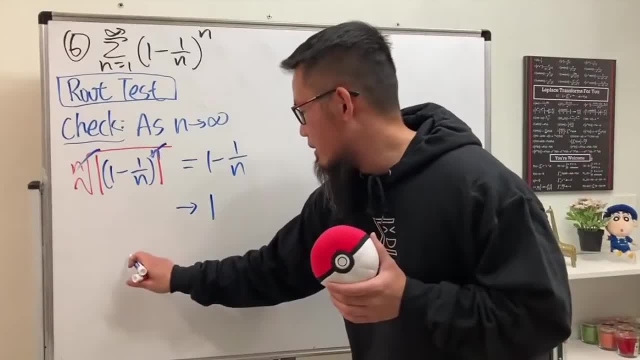 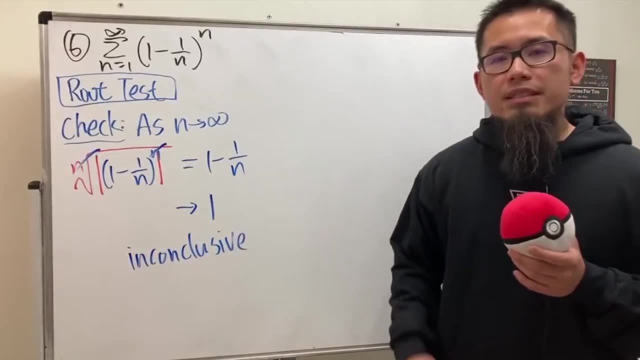 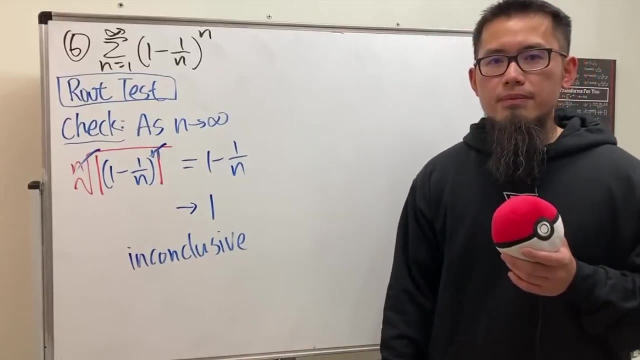 But yes, 1 is inconclusive. So this right here Is inconclusive. So what does that mean? Does that mean that root test is inconclusive? And then we are done, Moving to the next question. No, it does not. If you see, inconclusive This means that 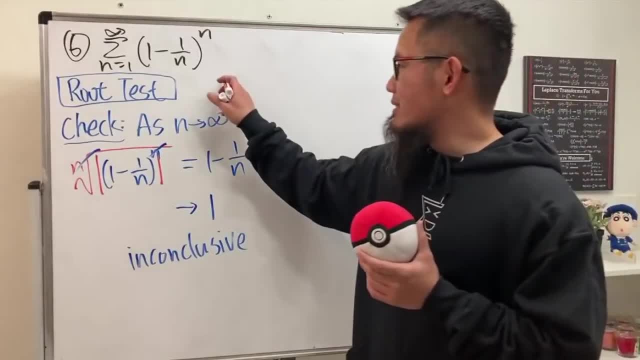 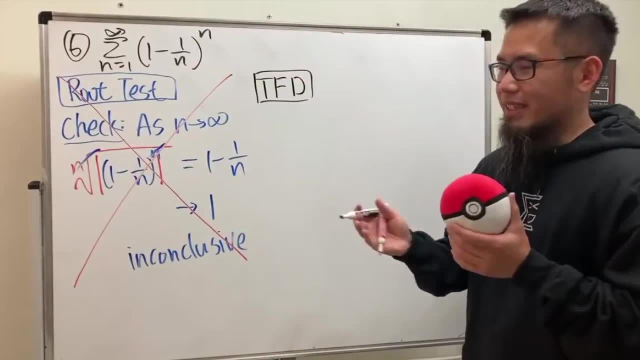 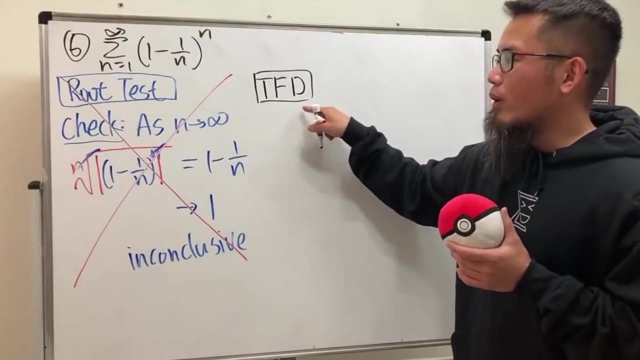 Man, We will just have to cross this out Because it does not work And we just have to pick something else To do more work. Yes, remember. In order to do all these things, You will also have to remember the things That we have done before. We are going to do the test for divergence. 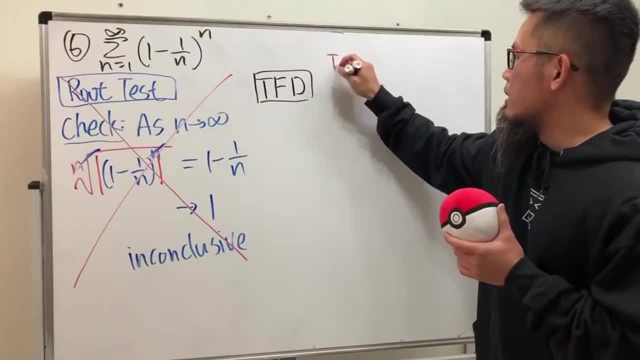 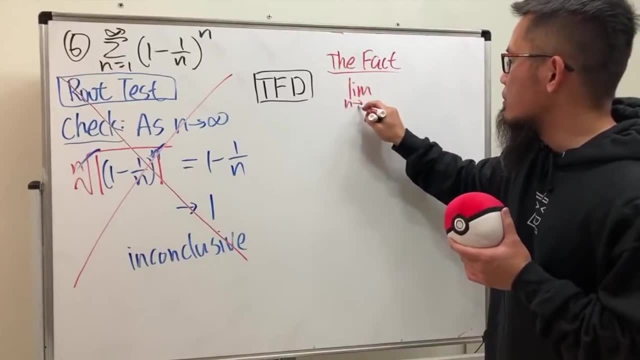 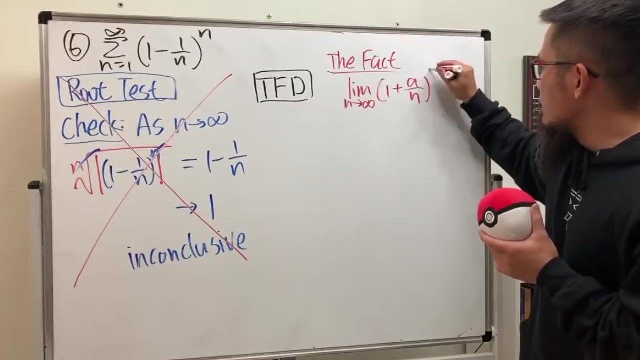 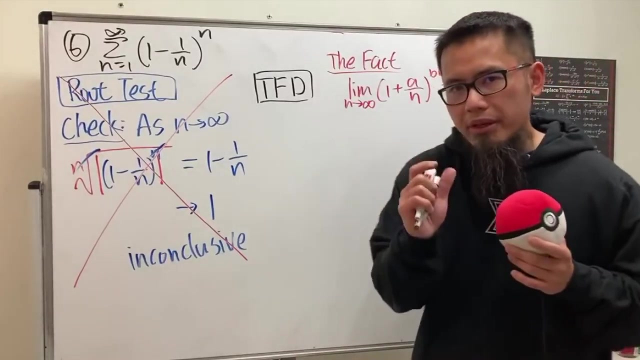 And again as a note, This is the fact. Well, we take the limit As n goes to infinity: 1 plus a over n n. this is an n Raised to the bn power. This, right here, will give you e to the ab power. And here's the. 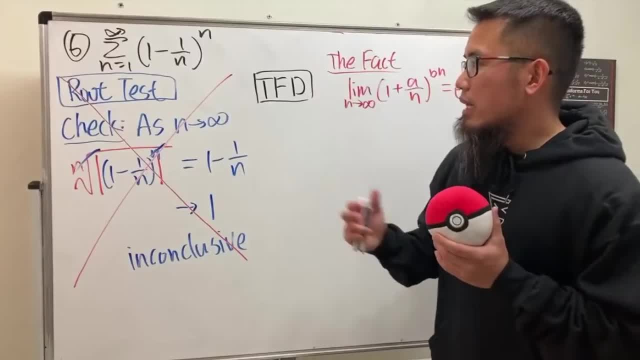 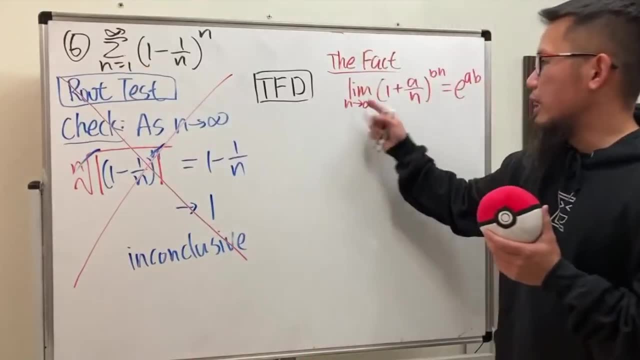 Perhaps the most confusing part Not a lot of students make, And that's why I did the first live stream, for It's the comparison between The sigma notation And also the lim Alright. so just to make sure, Just keep that in mind, Well, whenever you are trying to test out. 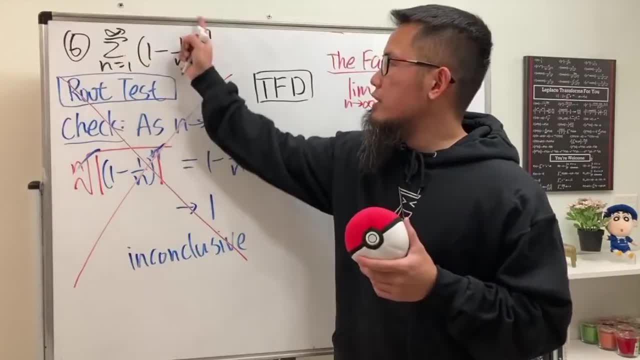 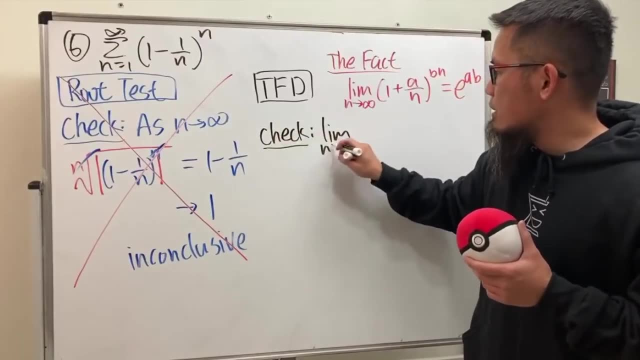 If a series converges or not, It's always a good idea To just check the limit of this thing. So we are going to check The limit As n goes to infinity And we put this down right here: 1 minus 1 over n Raised to the nth power. 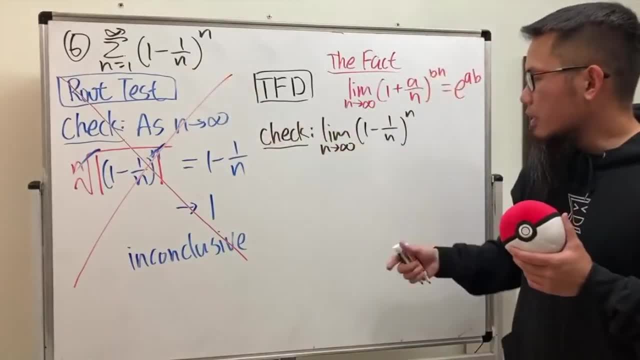 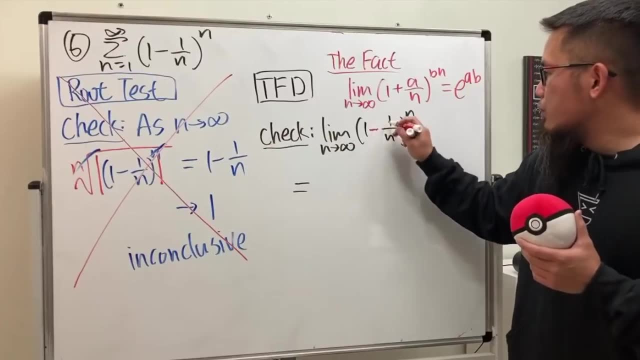 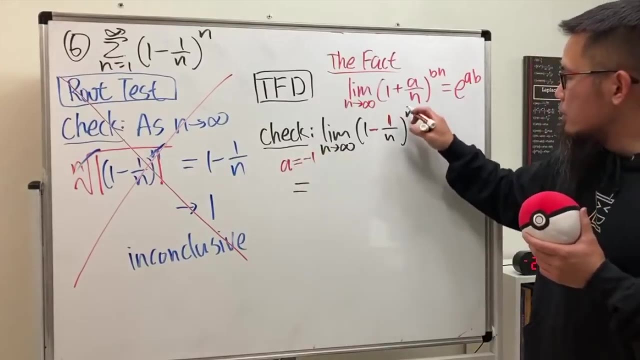 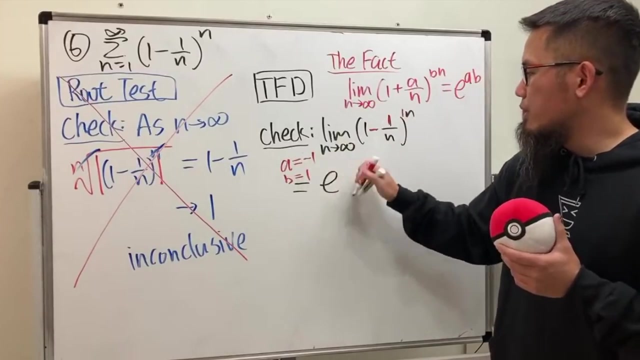 Just going to check this Right, just going to check the Am portion And take the limit for that. Well, how can we do this? Notice that a is equal to negative 1 And b is equal to 1, So this limit, By the fact, Is just equal to e to the. 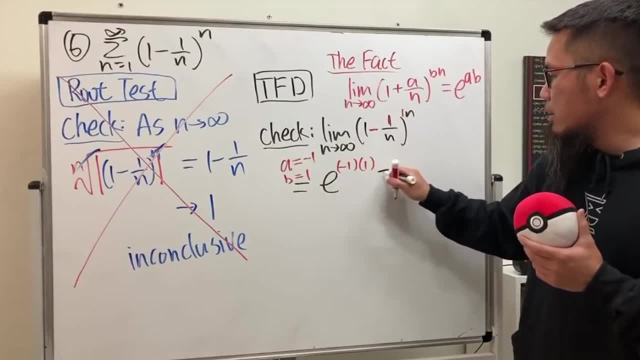 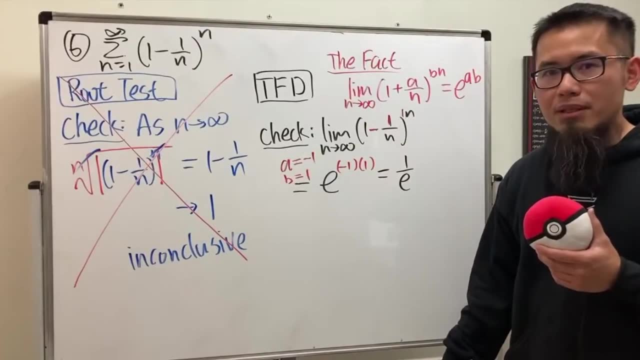 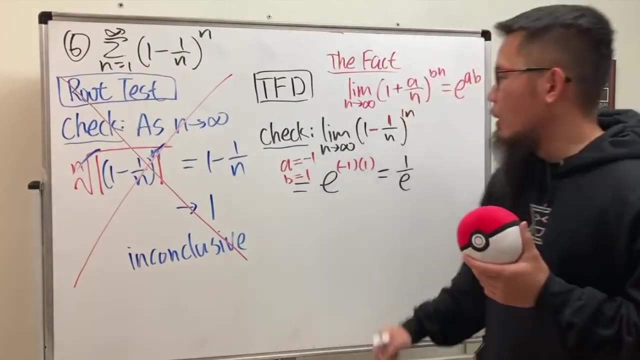 Negative 1 times 1, Namely e, to the negative 1, Which is 1 over e. So what does that mean? Does that mean that this right here converges to 1 over e? No, it does not. We are trying to do the test for divergence. 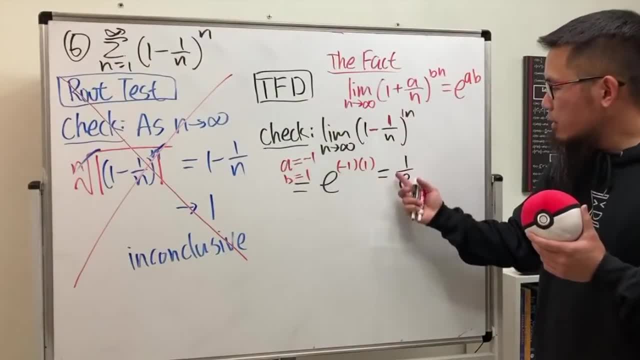 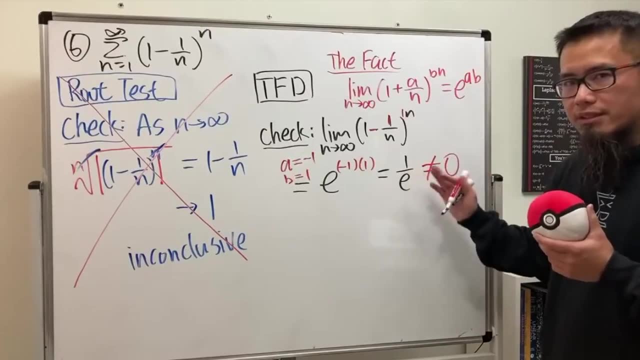 And when you have 1 over e, As long as this number right here Is not equal to 0. So again, do not say this is 1 over e. You have to say this is not equal to 0, Then congratulations, We get to draw a conclusion. 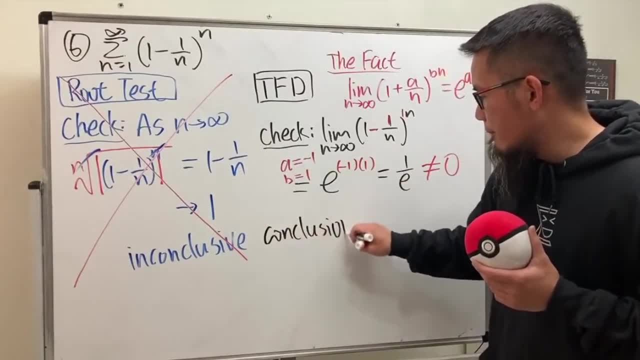 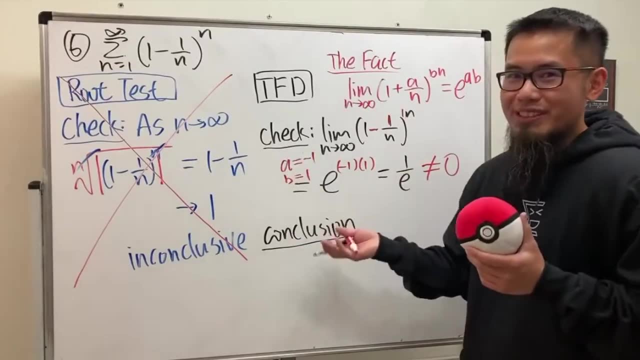 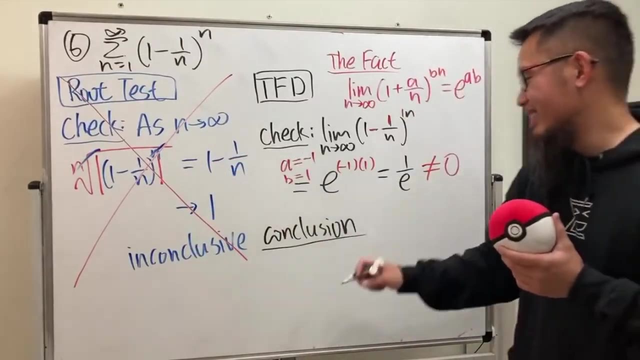 And the conclusion is the following- And, by the way, We actually did the same question On the first live stream. Okay, So we will just do that. And the thing is that When you learn more tests, You should not forget about the old tests either. So that's the idea. 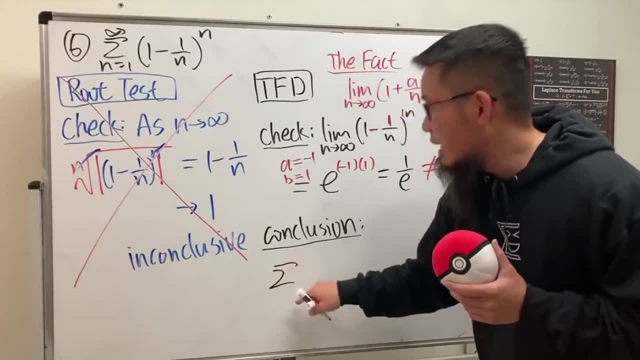 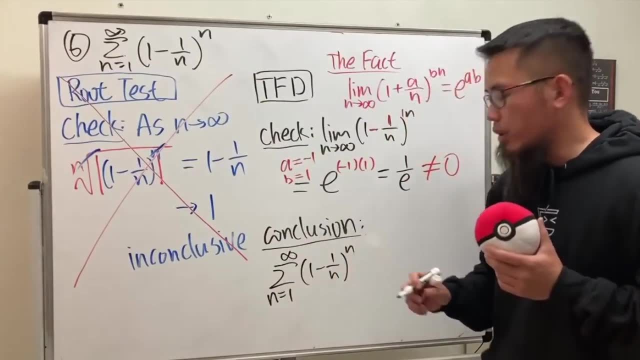 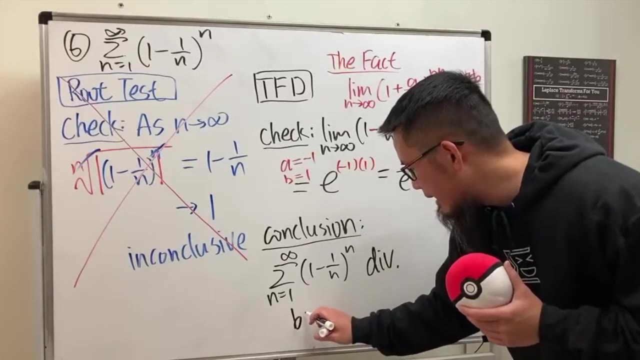 Anyway, here's the conclusion. The conclusion is that The series As n goes from 1 to infinity, 1 minus 1 over n, raised to the nth power. This guy right here Diverges Y by The test for For divergence. Hurry up, hurry up, hurry up. 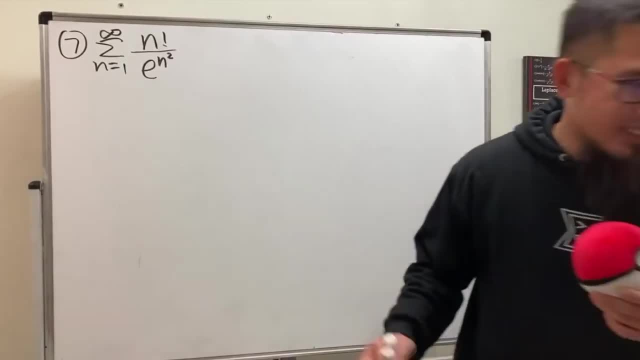 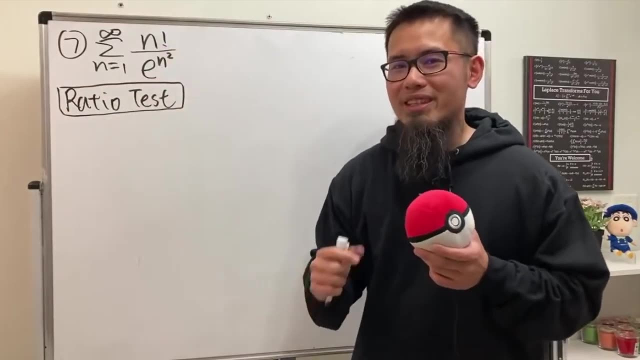 Ratio test will work. I'll do java. that's correct. Yeah, So let's go ahead and do the ratio test. Why ratio test? Well, Factorial, right, That's usually a good indicator. You should use the ratio test. Give it a try. Ratio test says: 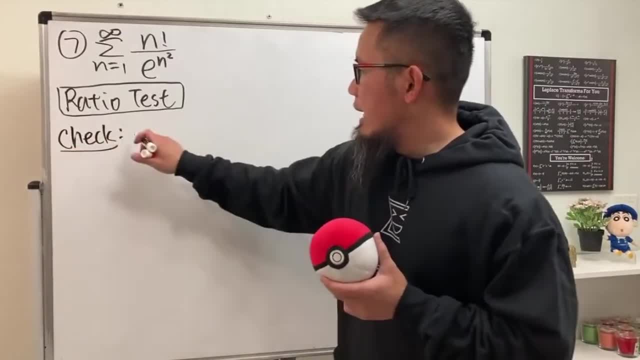 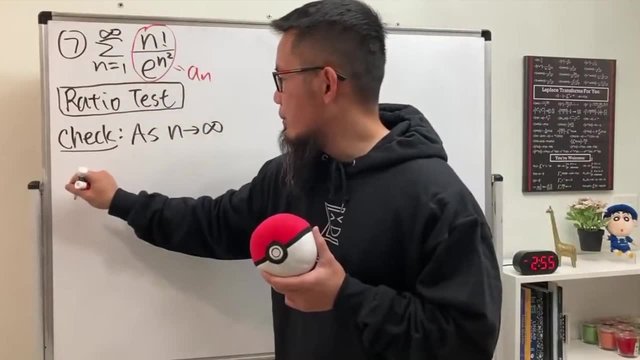 We are going to check As n goes to infinity. Here is the a n, And here is the a? n, And we are going to do the. We are going to do the absolute value, We are going to do the a? n plus 1. So on the top here, 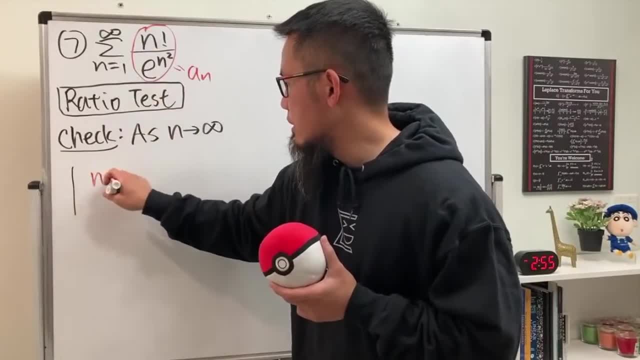 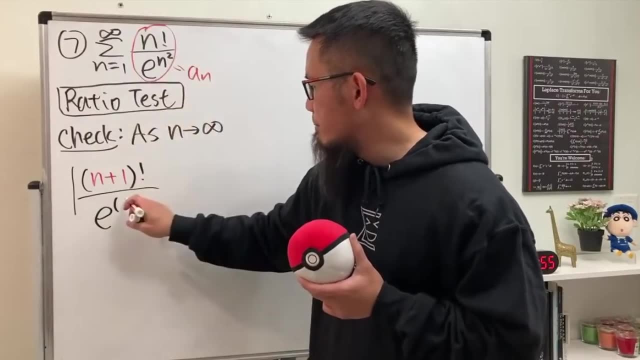 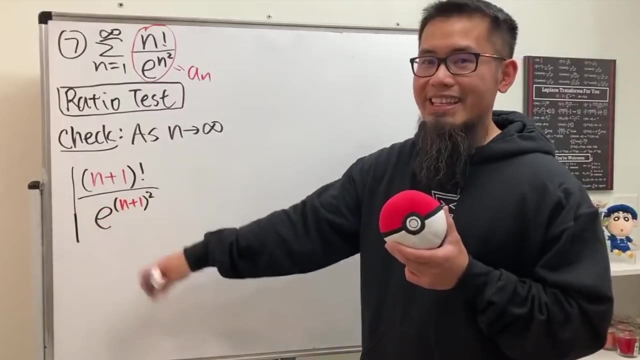 It becomes n plus 1 factorial. So let me just write that down: n plus 1 factorial, that And over e, And then the n becomes n plus 1, And then you raise that to the second power like: so Right, So that's a n plus 1. 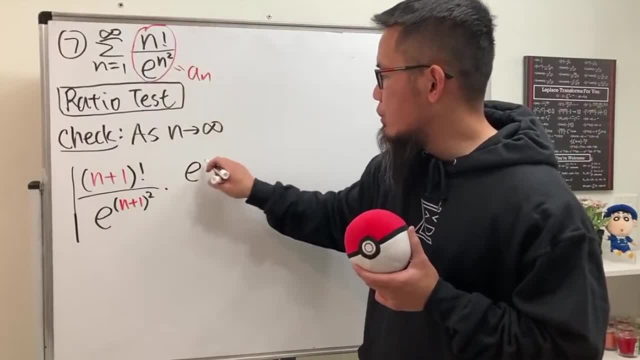 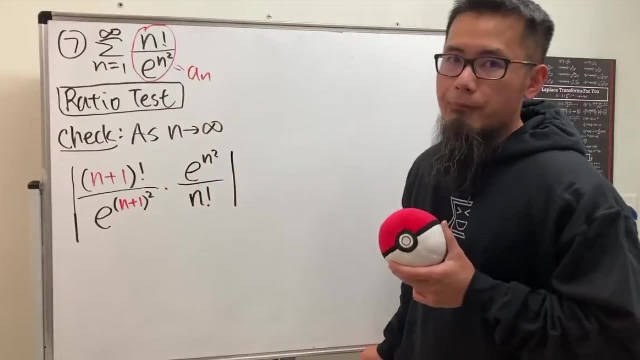 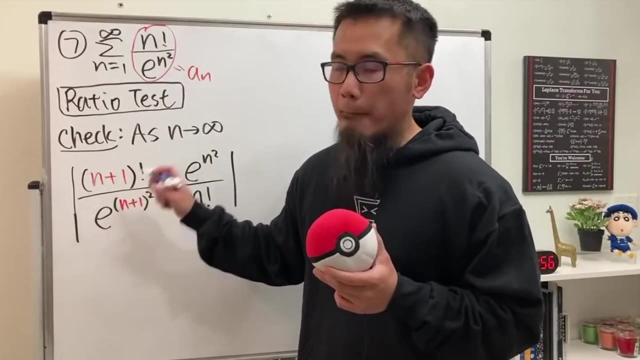 And we will multiply by the reciprocal of that. So we get e to the n squared, n squared over, just n factorial. Pretty good so far. Now we are going to simplify the bigger factorial And also the bigger exponent For this guy. n plus 1 factorial means You put down the inside first. 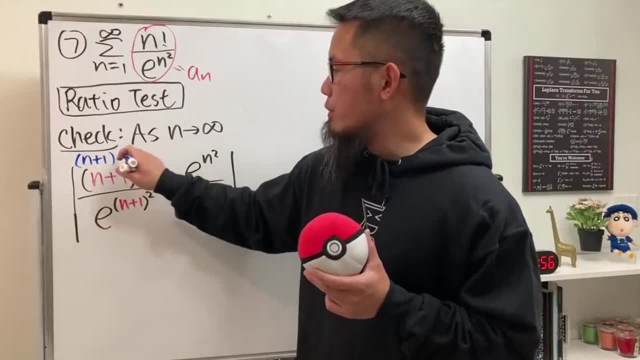 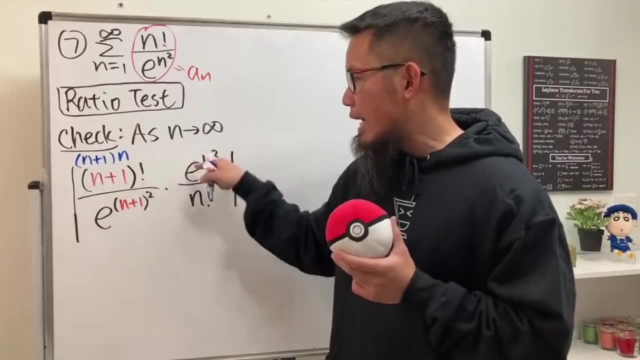 Which is n plus 1, And the next. You put down the next number, which is n, And then you put down n minus 1, And then you put down n minus 2, and so on. But all that is just Nicely equal to n factorial. Now to simplify this exponent: 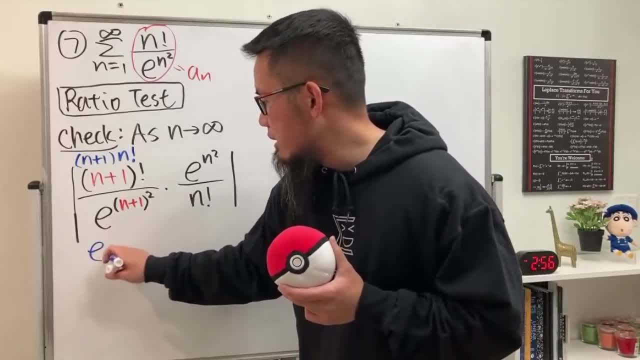 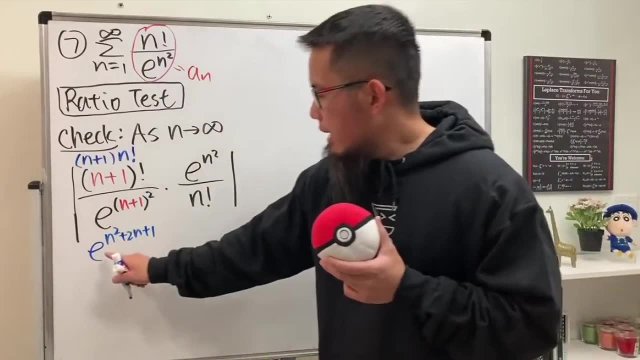 Of course we can just multiply this out, Which is e, And then we have n squared plus 2n plus 1 After you multiply that out, And then we can use the rule of exponent And rewrite it as e to the n squared Times, e to the 2n. 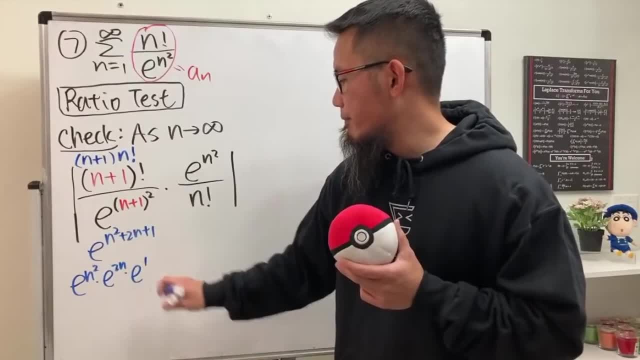 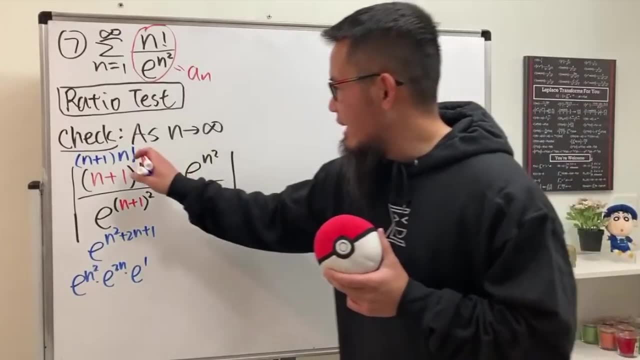 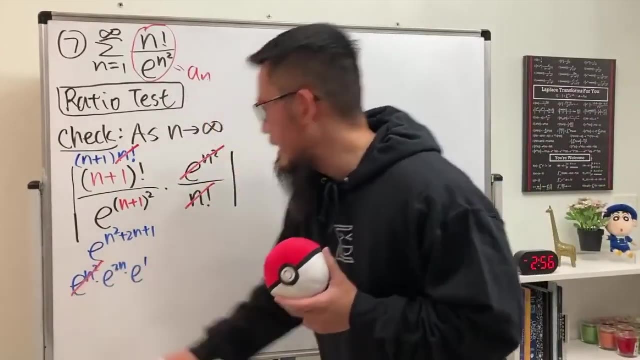 Times e to the first power. And now we are going to have fun Because we can do a lot of cancellations. Not really, but at least two cancellations, Ladies and gentlemen. Let's cancel this out with that Also. let's cancel this out with that. Pretty good so far, huh. 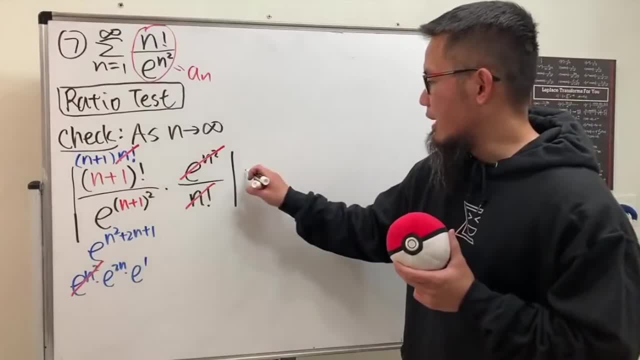 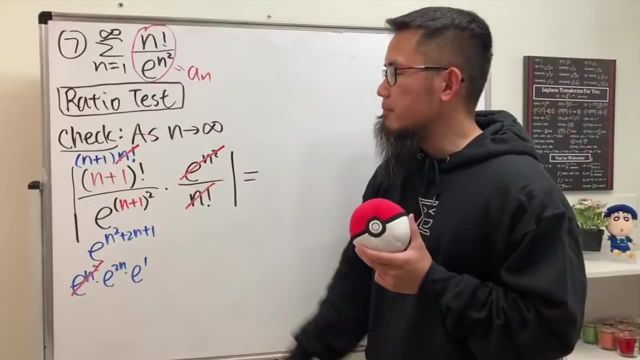 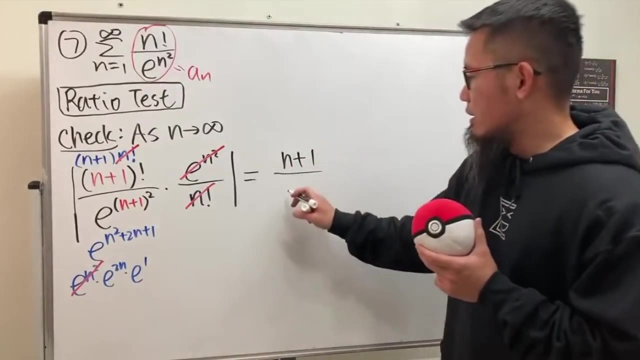 As I told you, it's pretty good. Alright, so after the simplification We will get Absolute value, doesn't matter, So don't even need to put that down, Because everything says positive. On the top we have n plus 1. On the bottom we have this. Perhaps you will write it as: 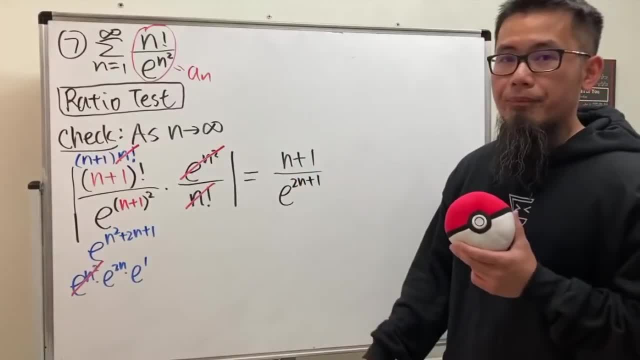 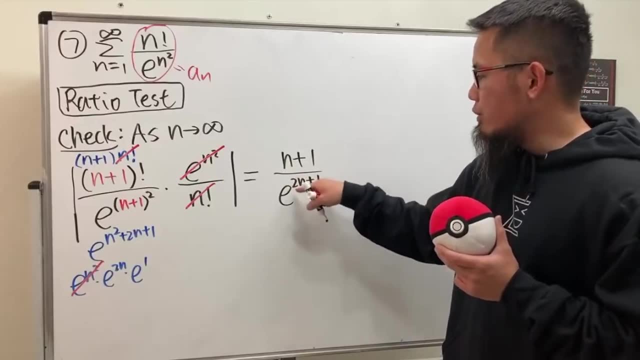 e to the 2n plus 1. So that's what we have Now. as you can see, we have Just n to some power Over an exponential Right e to the 2n plus 1, and all that This right here, You can just tell me real quick. 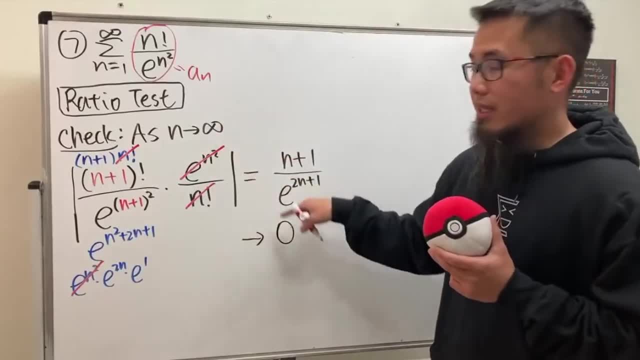 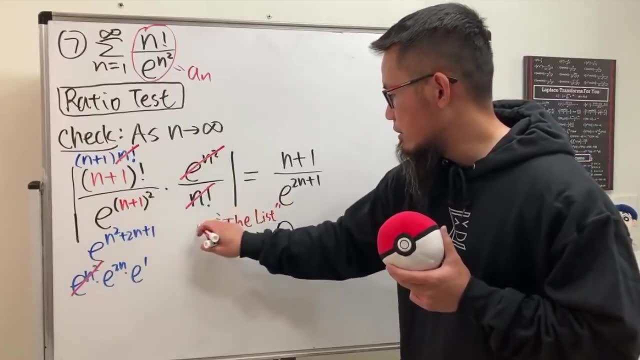 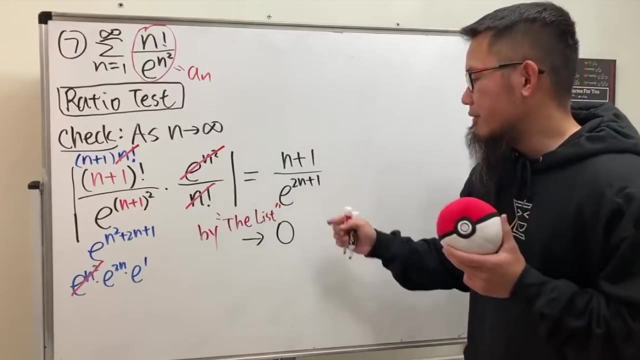 It's equal to 0 And again We are doing the limit. So we can say By the list. Right, so just say by the list, Because this is way bigger than that, How much bigger? Big enough that you will get 0 If you do the smaller one. 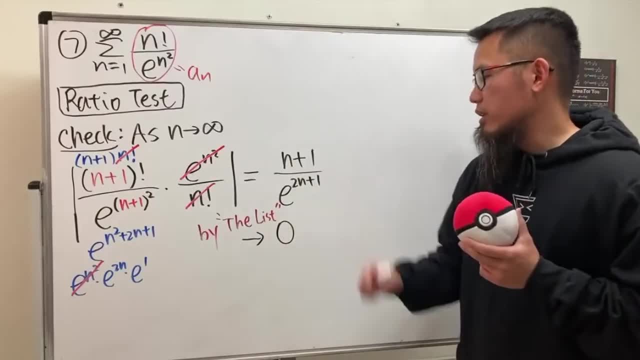 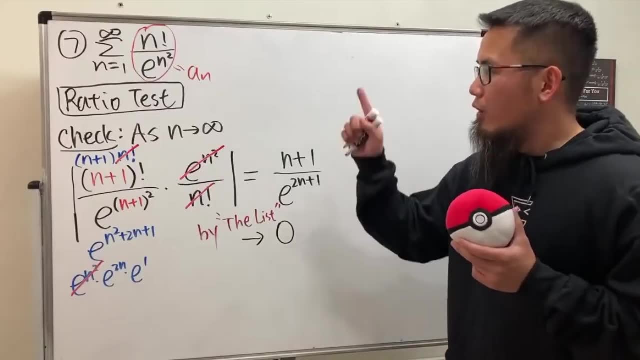 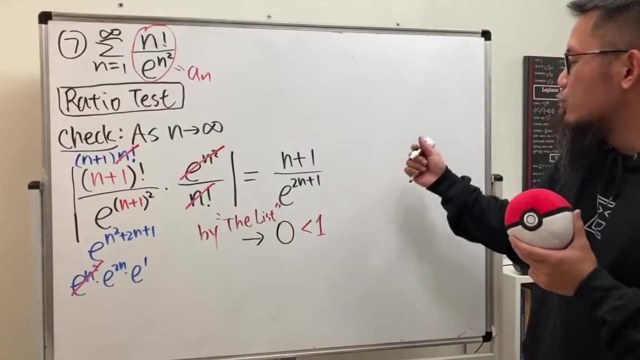 Divide the big one And take the n goes to infinity. That's what this is saying. Well, does 0 do us any good? Yes For the ratio test. If we end up with 0, Then please mention that This is less than 1. Therefore, we can draw the conclusion. 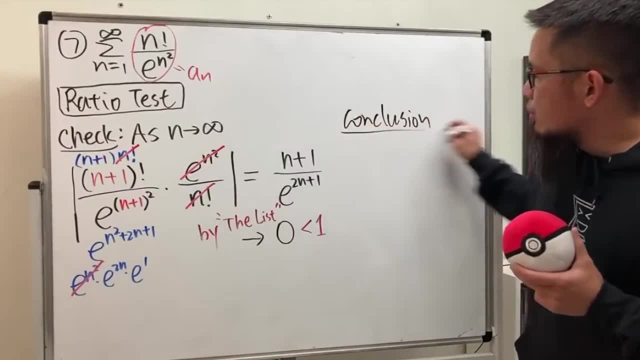 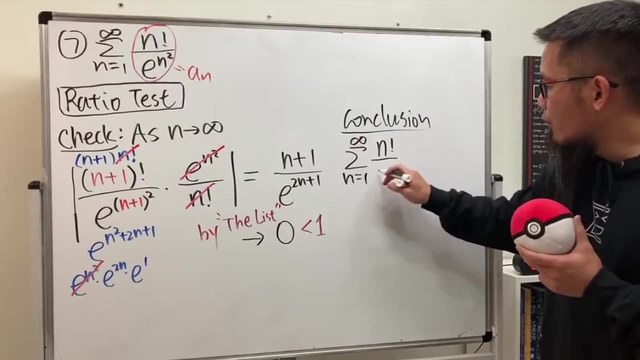 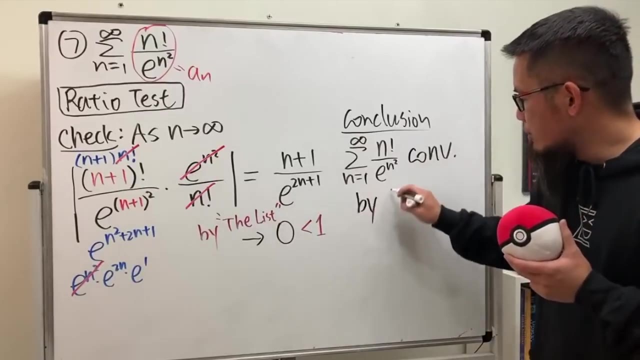 So let me just write that down here. The conclusion is that The series as n goes from 1 to 0, n goes from 1 to infinity, n factorial over e to the n square. This guy converges y by the ratio test, Ratio test, And then we are done. 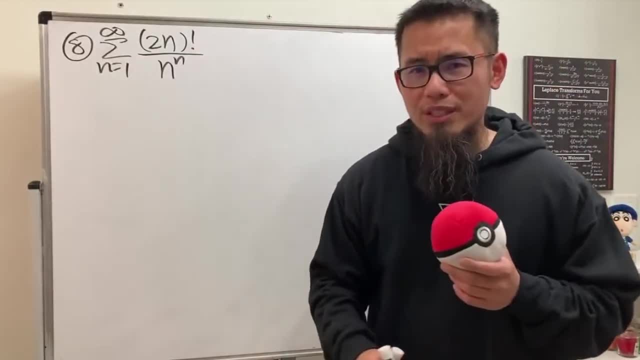 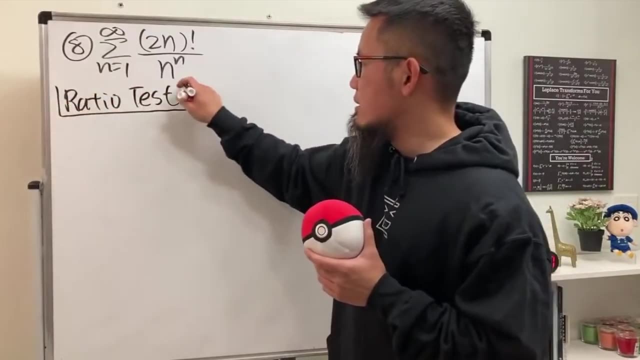 Converge to diverge. We have the factorial and also the n Ratio test is a good idea, Right? so here we do the ratio test, And usually the ratio test is One of everybody's favorite Because it has a good indicator That when you should use the ratio test. 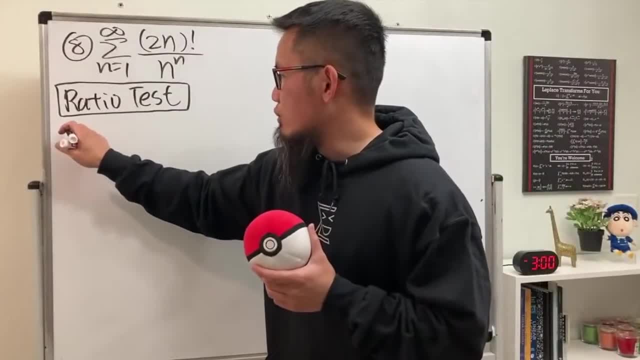 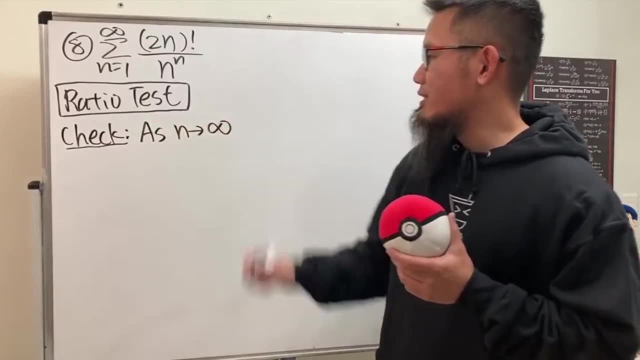 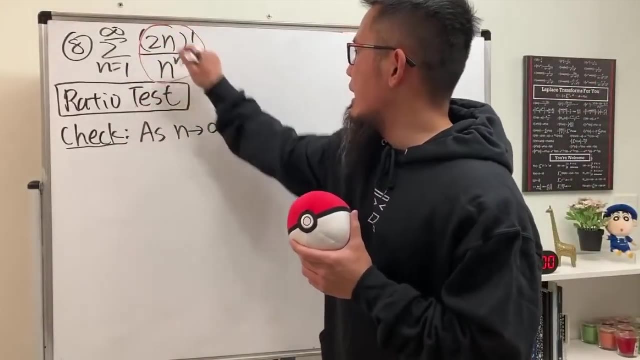 Right because of the factorial, And then you can do a lot of algebra. I think this is one of the things that Students might like: the ratio test More than the other ones. Anyway, take the limit as n goes to infinity. Alright, here is the a- n. Go ahead and put down a n plus 1. 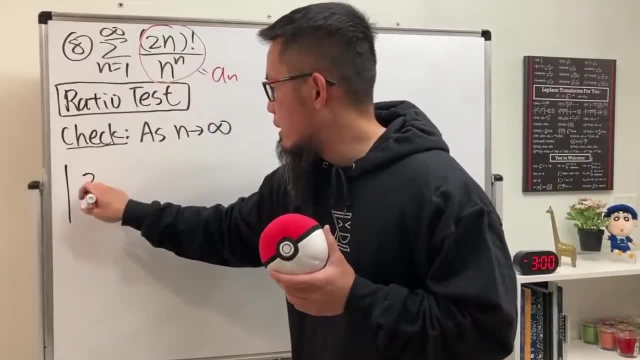 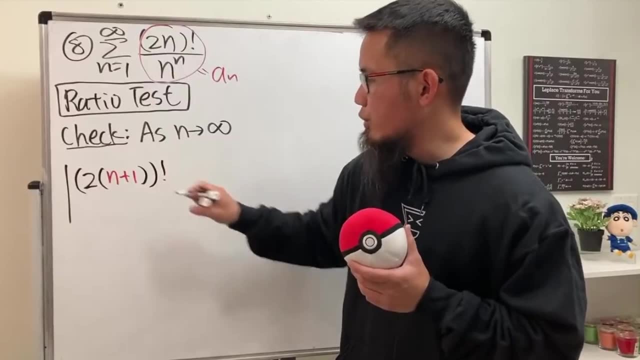 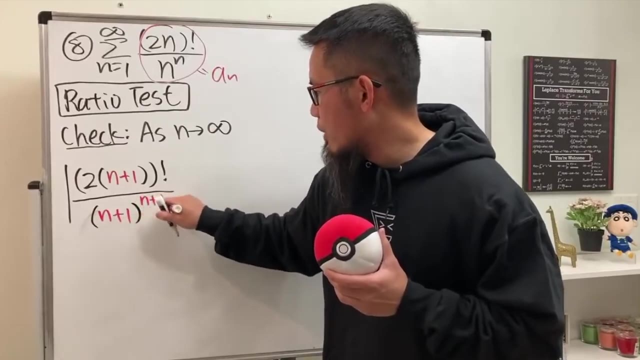 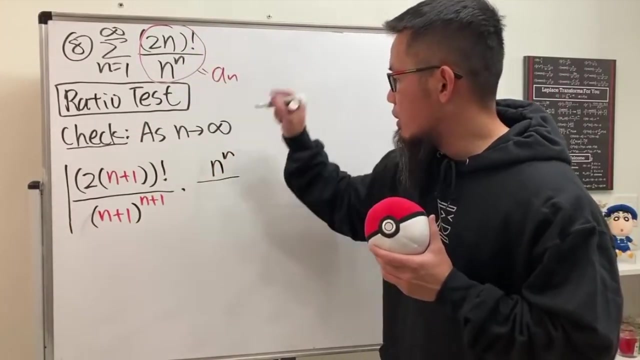 So be really careful, though. We have 2 And the n becomes n plus 1, And then after that, After this, we factorial this And then divide it by n plus 1 and then n plus 1, And we will multiply this by It's reciprocal n to the n over 2n in the parentheses. 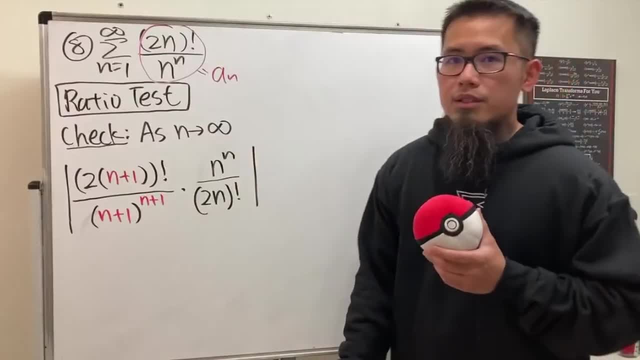 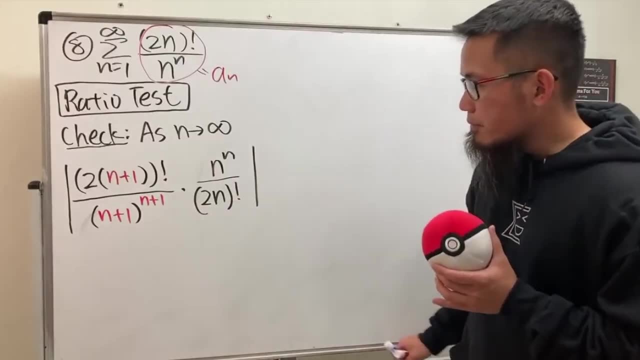 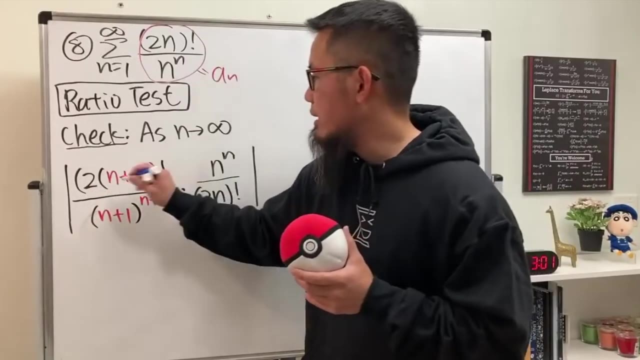 And then we factorial that Like that. So for this right here, the trick Is just to simplify the factorial carefully And also simplify the exponent Carefully, like that. Here is the deal. This right here is the same as 2n plus 2, And then you factorial that right. 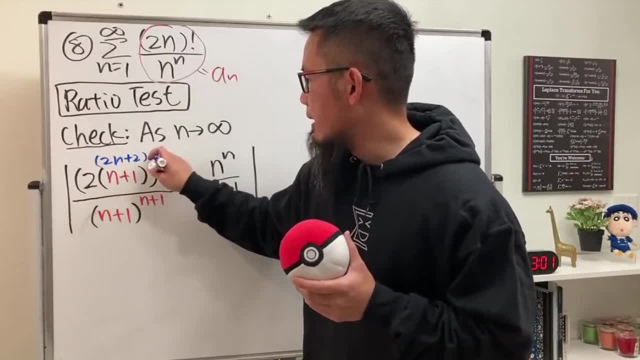 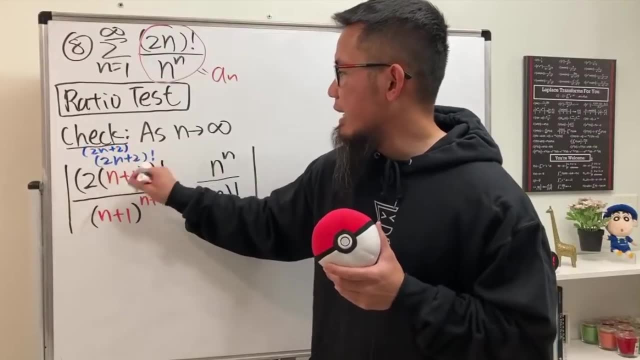 So this is 2n plus 2 factorial. How do we simplify that? Well, we first write down 2n plus 2, That's the first guy, And then we multiply by the next one, Which is 2n plus 1, And then the next one is just 2n. 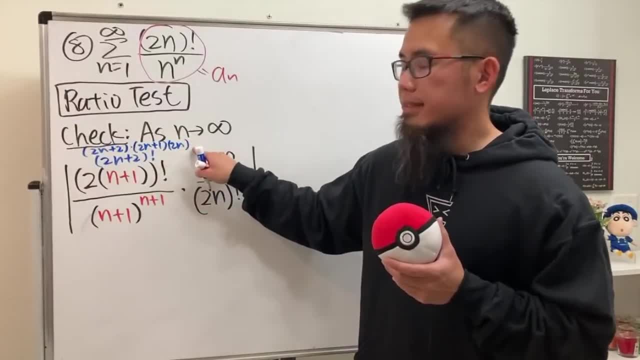 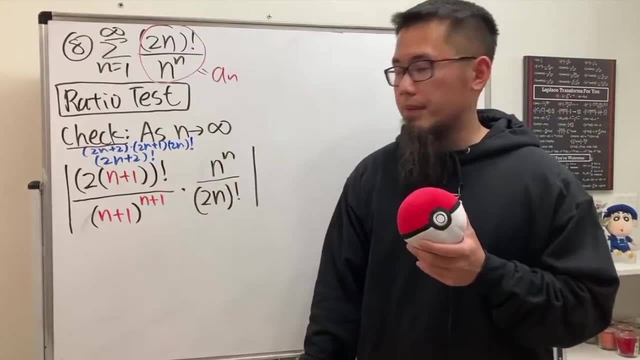 In the parentheses. And then the next guy is 2n minus 1, And then 2n minus 2, and so on. So all this becomes 2n factorial like. so Simplify this. The base stays the same. So we have n plus 1 raised to the nth power. 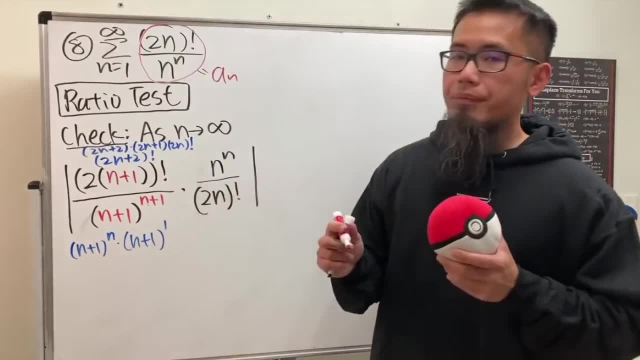 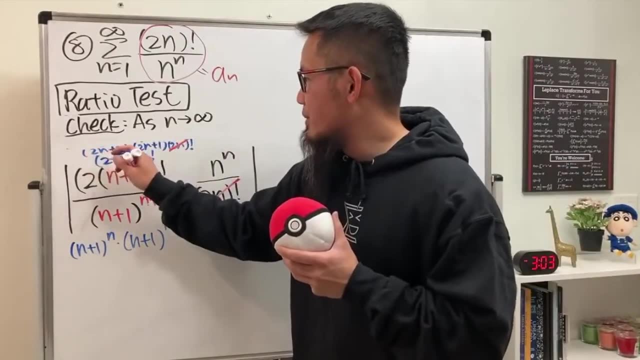 Times: n plus 1 raised to the first power. Alright, Happy cancelling This and that. cancel out The 2n plus 2 is the same as 2 parentheses n plus 1, And of course we still have the 2n plus 1, Right so? 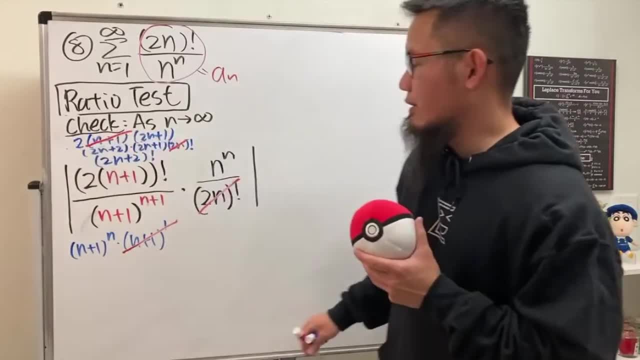 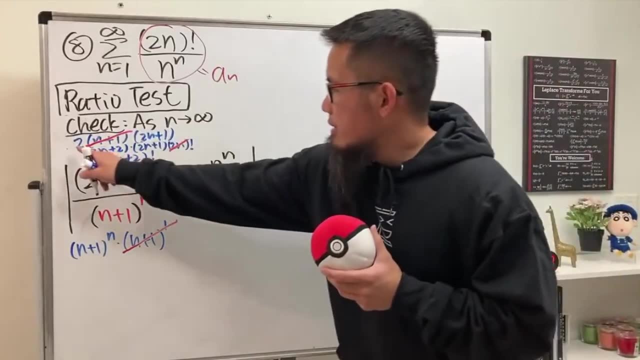 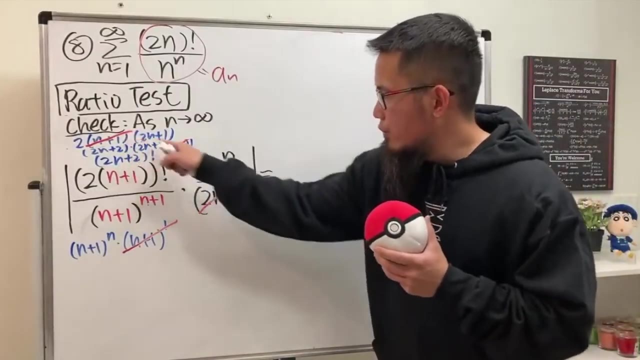 This guy And that guy Cancelled out nicely. Okay. So so far, so good. And now what's the result? After all the algebra On the top, we have this times that, So 2 times. Let me write it down like this: 2 times that. So it's 2 times 2n plus 1. 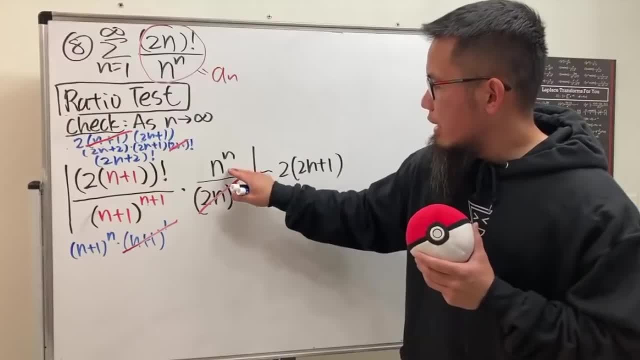 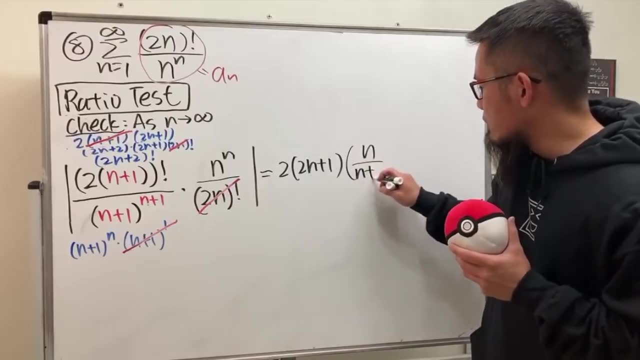 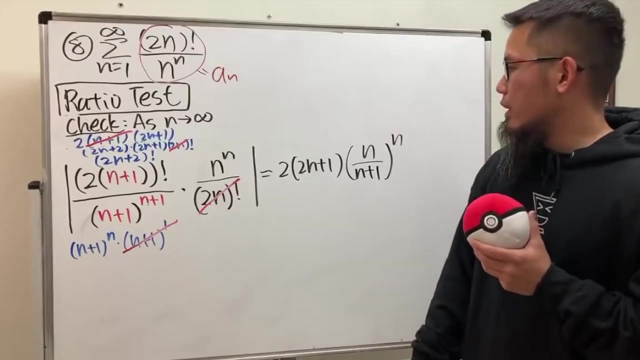 Okay, Well, we still have n to the n Over that, But both of them have the nth power, So I'm going to write it as n over n plus 1 raised to the nth power, Like so, Alright, So now, how can we simplify this? Well, I'm going to bring up the 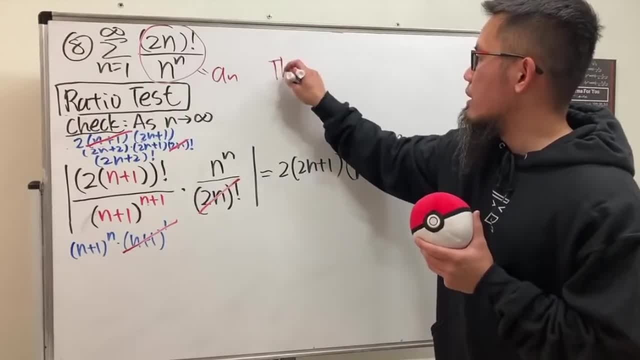 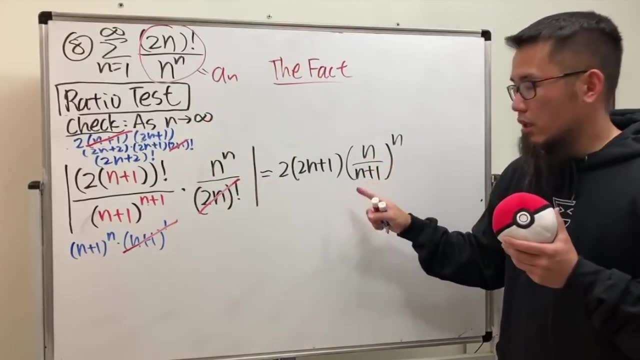 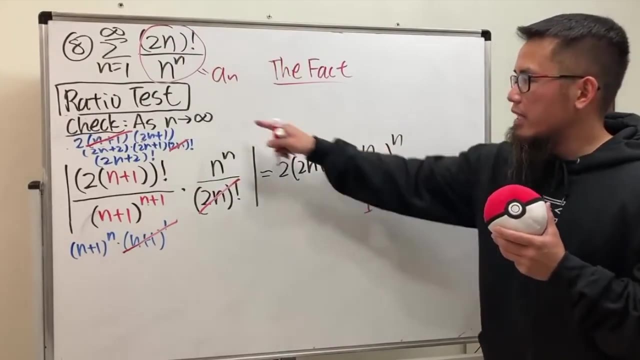 Fact again. Maybe just write it down real quick, Because Here's the thing: If you put infinity into here, You get infinity. Well, inside here you have 1, Because you just care about this and that. So it's actually 1 Right. And then, if you put infinity to here, 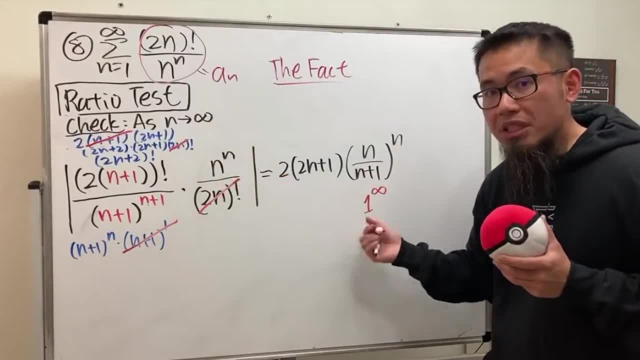 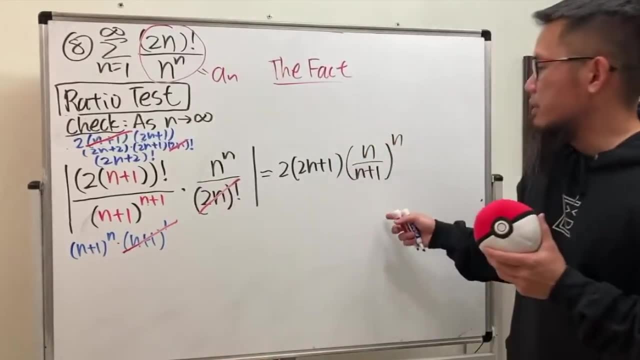 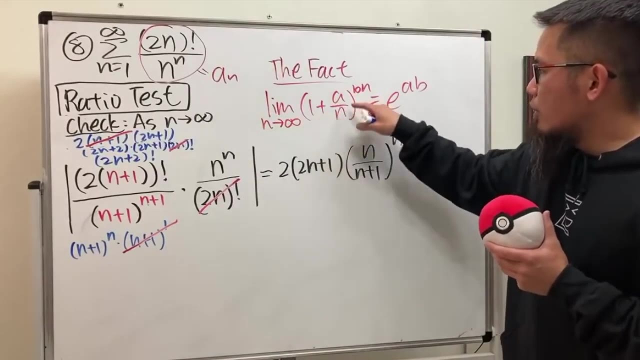 You have 1 to the infinity, But unfortunately We cannot draw a conclusion on this Right, So we cannot draw anything. We cannot draw any conclusion on this, But this right here Is actually really similar To the fact, You see, that We have 1 plus a over b. 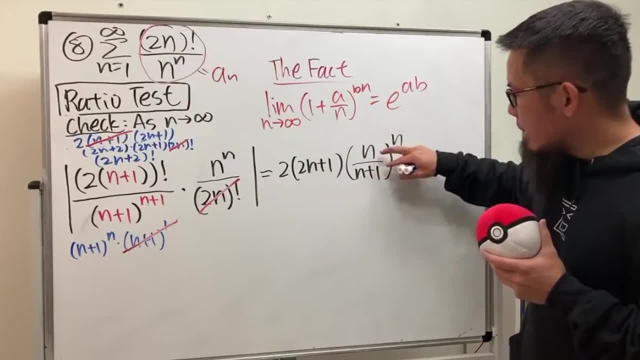 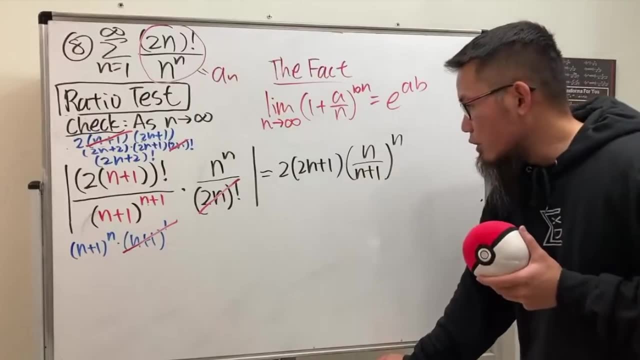 This right here is n over n plus 1. Imagine if we do the reciprocal. That would be much better, Because then we just have n on the bottom And then we can split the fraction. So here's how we are going to do it. We still have the 2. 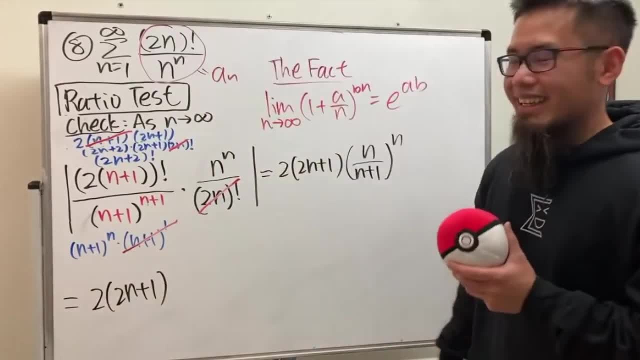 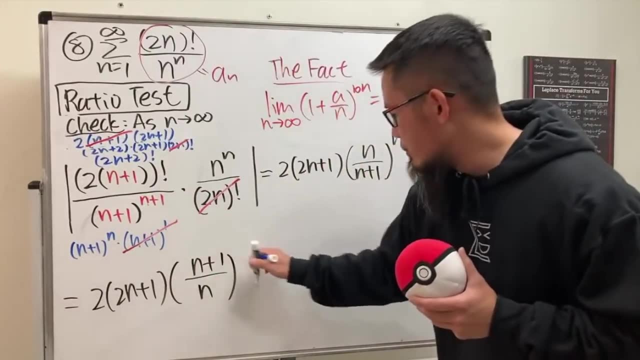 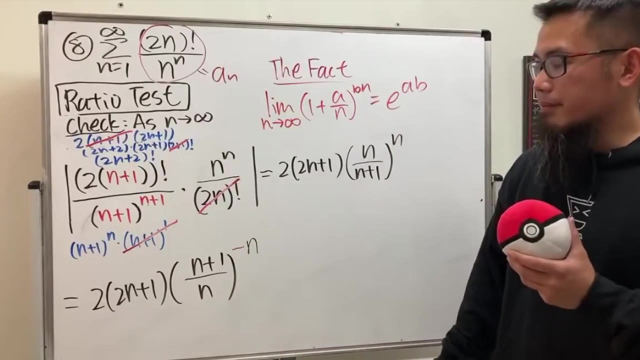 And then 2 n plus 1, And for this I'm going to just turn it Upside down like so n plus 1 over n, But I will actually do the negative power here, So this becomes negative n. So I can just do the reciprocal like that. 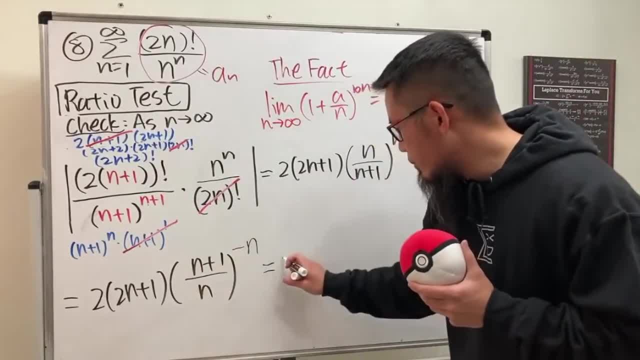 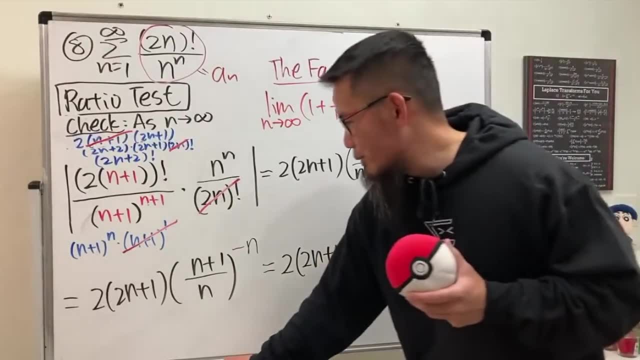 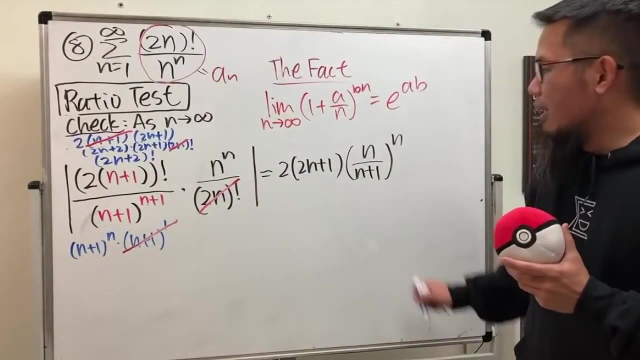 And now check this out. This right here is 2 times 2n plus 1, And You know what? I'm going to write it down like this. It's going to be cleaner. I just realized how I can write it down clean. Sorry, I'm going to do this statement. 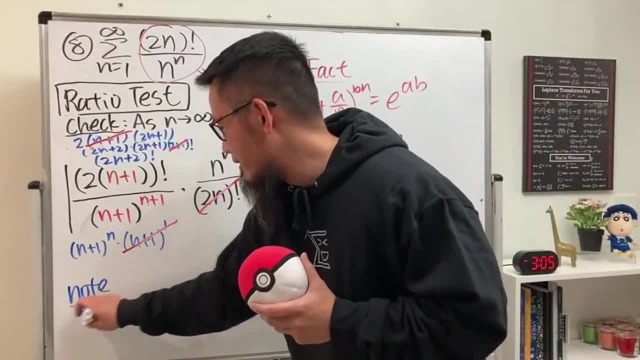 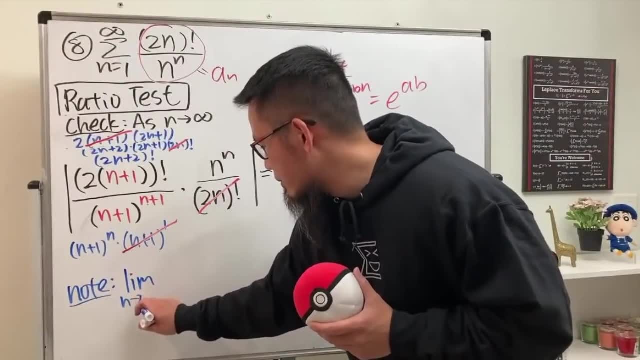 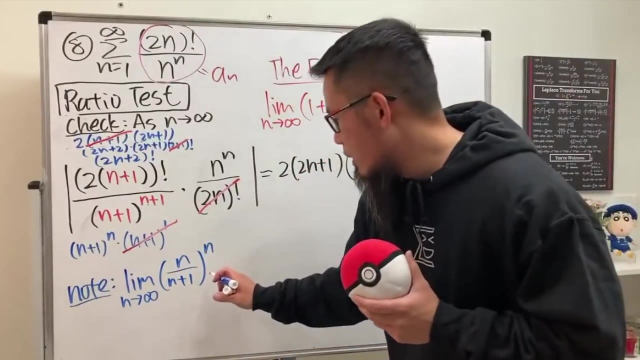 On the side here. So hopefully That will make everything more better, More better. Yeah, I guess, If you look at this, The limit as n goes to infinity, Just that part right Over n plus 1 raised to the nth power. This right here. Well, you can write this down as: 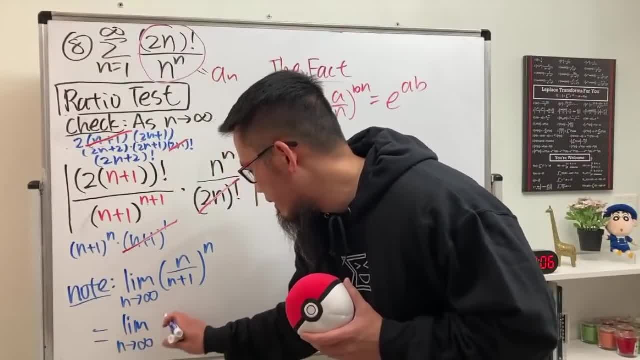 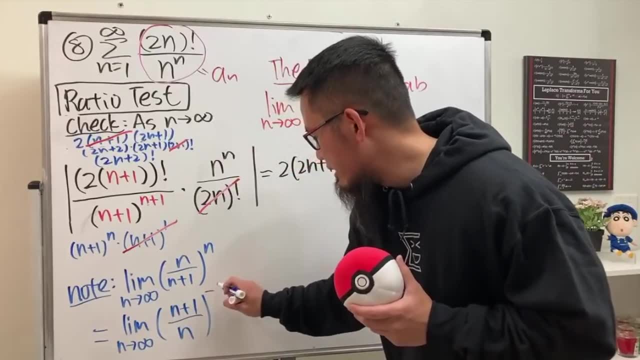 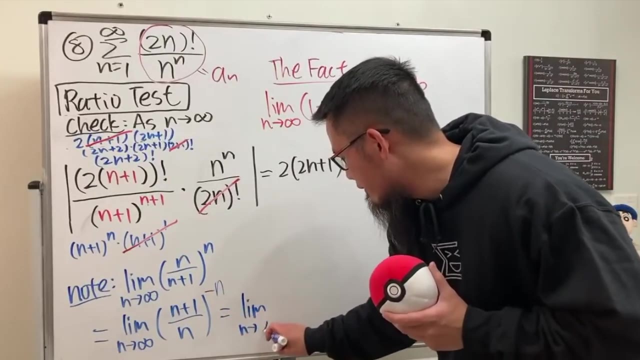 The limit, as n goes to infinity. Do the reciprocal, So you have n plus 1 over n, And then, raised to the negative nth power, Like: so: Split the fraction. So this, right here, is The limit, as n goes to infinity, And then you have 1 plus 1 over n. 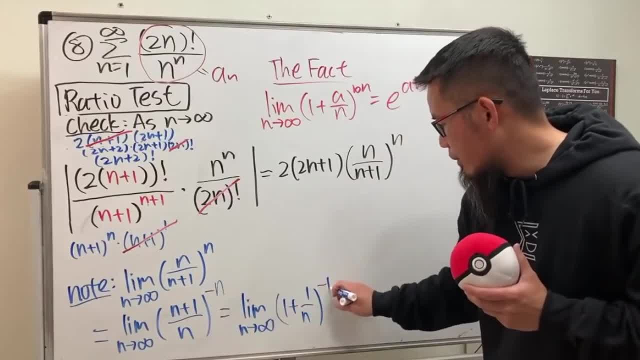 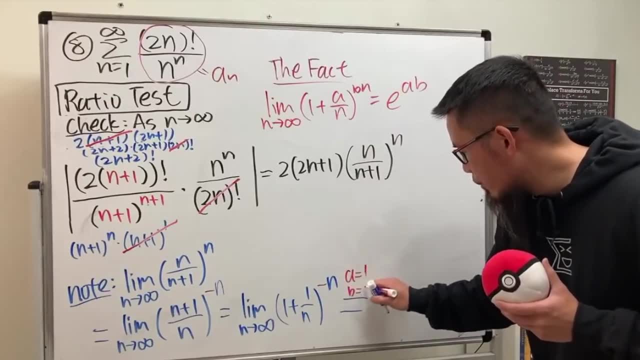 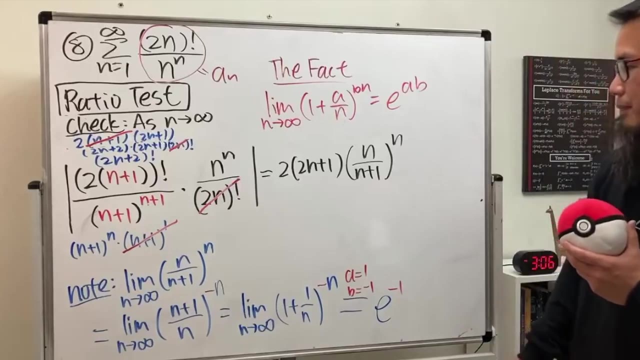 Raised to the negative nth power. There we go. In this case, a is equal to 1 And b is equal to negative 1. So this right here gives us e to the negative 1 power again. Alright, So now Remember we are still taking the limit, The limit of the product. 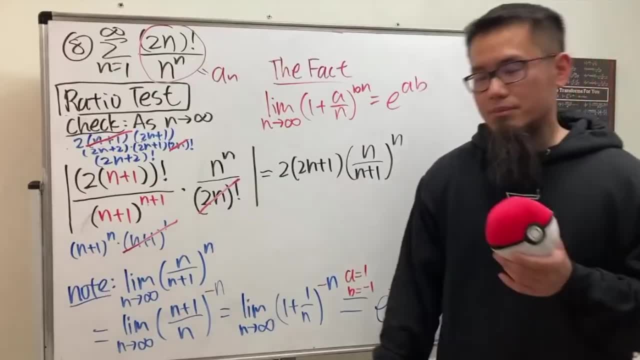 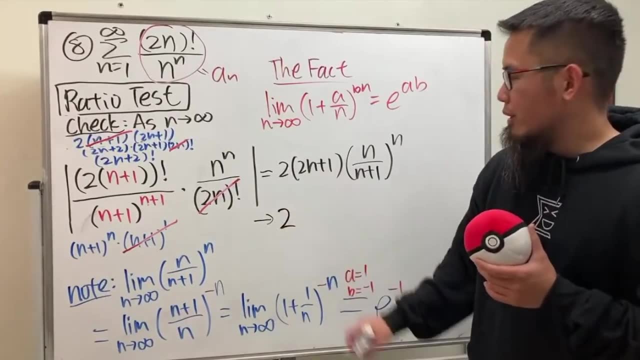 Is the product of the limit, If each limit exists. Have a look right here. This right here, Is going to approach- We still have the 2 right here, No big deal. And for this guy It actually It's going to give you infinity. Right, This guy is going to give you infinity. 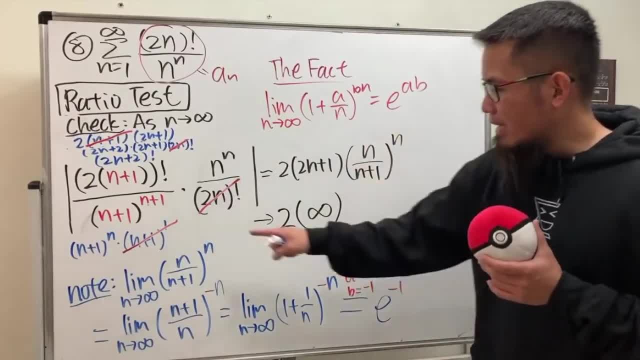 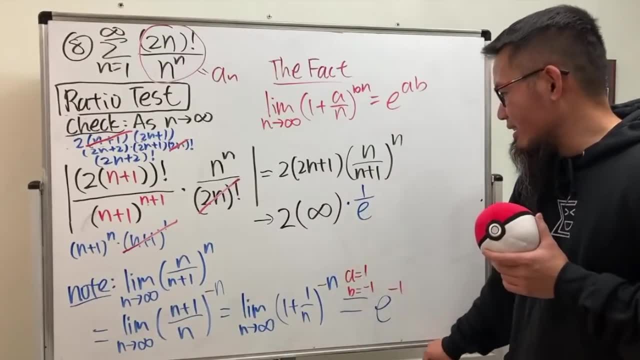 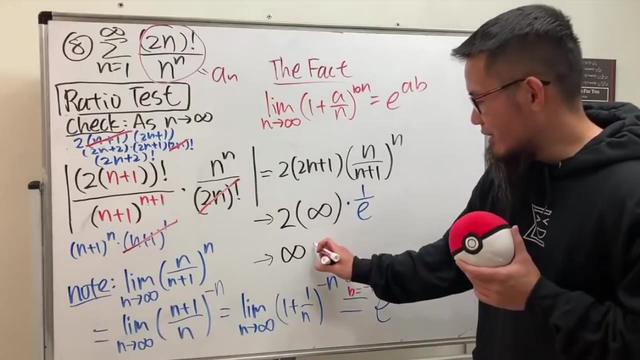 Because n goes to infinity And for this, By the blue portion, It's going to give us 1 over e. This right here becomes what? Just infinity. So this right here is actually just going to be approaching Infinity. Therefore, This right here is- This right here is greater than 1.